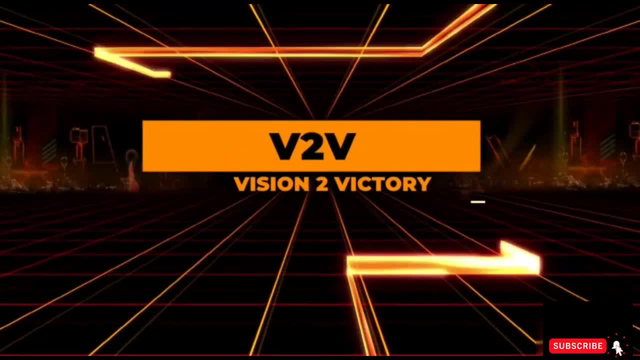 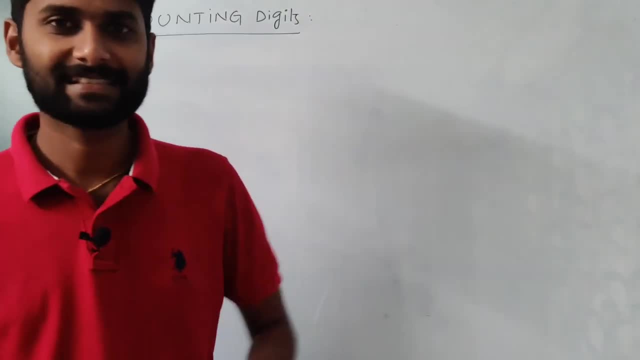 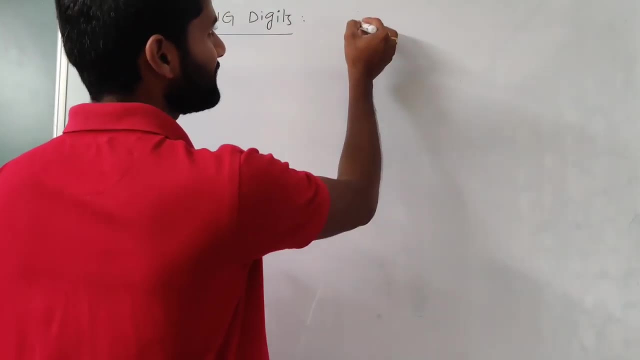 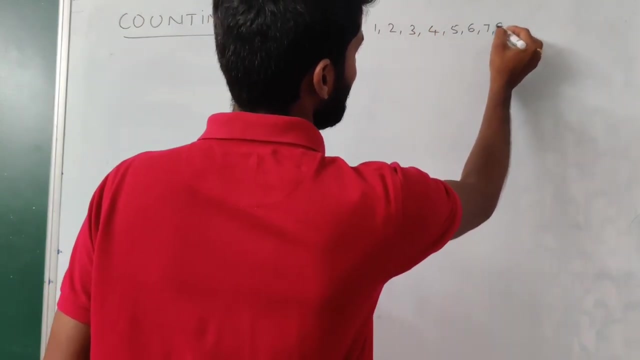 Let's see the next topic in number system, counting digits. See, we know that numbers, so we'll start with the numbers from 0.. So 0, 1, 2, 3, 4, 5, 6,, 7,, 8, 9.. So out of these numbers, 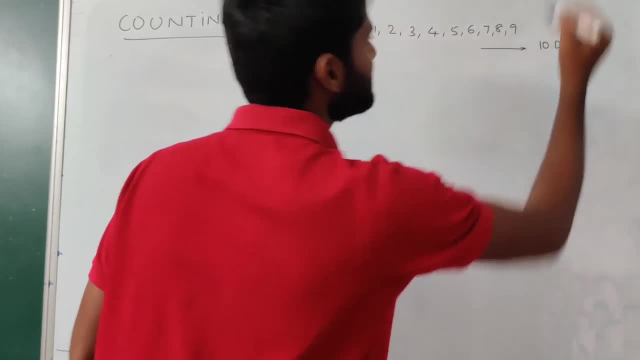 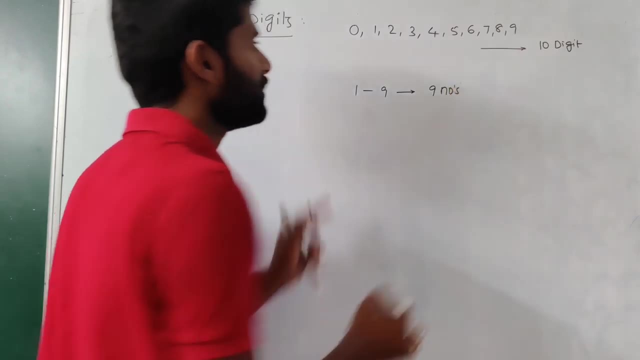 we are using. the total number of digits are 10 digits. For example, if you go with a 1 to 9,- 1 to 9, we have a 9 numbers. See 1 to 9, we have a 9 numbers. So if you form a number, 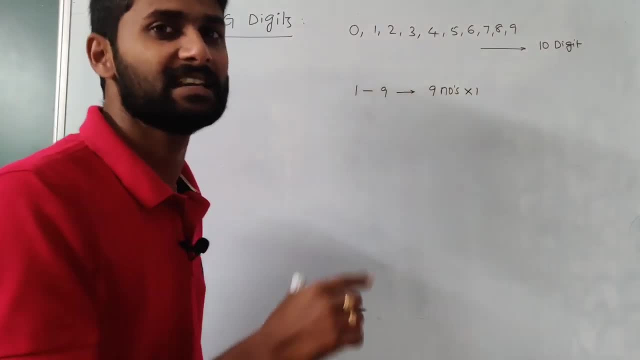 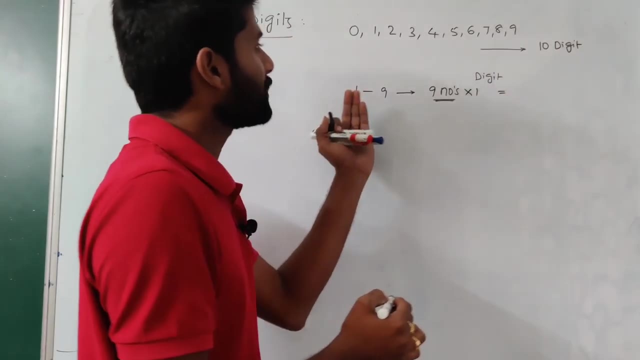 we require 1 digit, So that's why we can call it as a single digit number. So we have a 9 numbers. we are using 1 digit. The total number of digits we are using, from 1 to 9, is a 9 only. 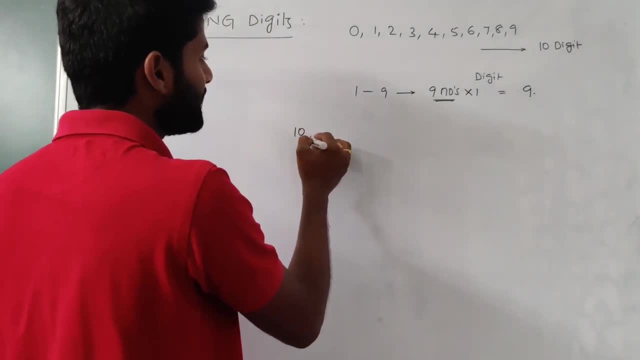 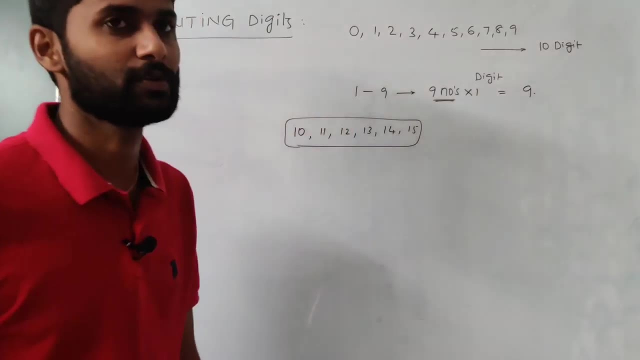 For example, if it is 10, 10,, 11,, 12,, 13,, 14, 15.. By framing 10 to 15, how many digits we are using: See total- we have a 5 numbers: See 10,, 11,, 12,, 13,, 14,, 15.. And if you're framing a 2: 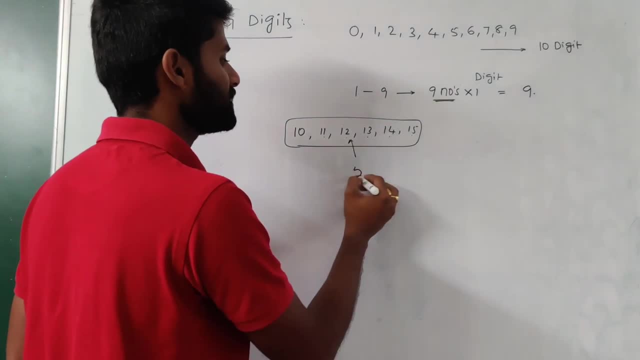 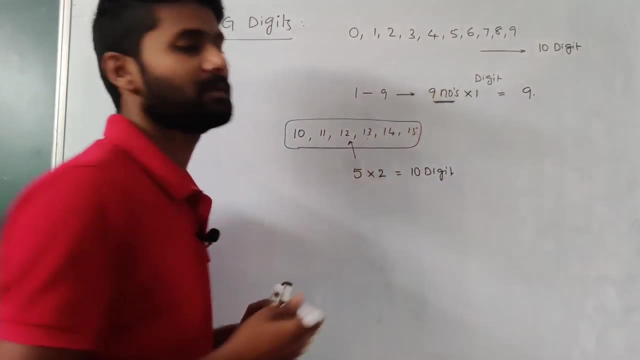 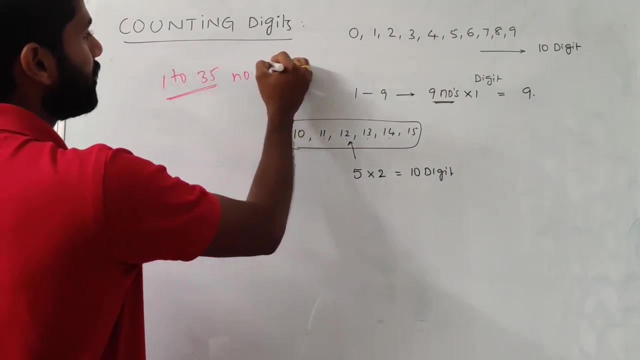 digit number. we are using 2 digits. It means we are using 5 numbers, So each number can frame with a 2 digits. The total number of digits are 10 digits only. Okay, based on this information, question number 1, 1 to 35, find the number of digits. So this is the question. So, from 1 to 35,. 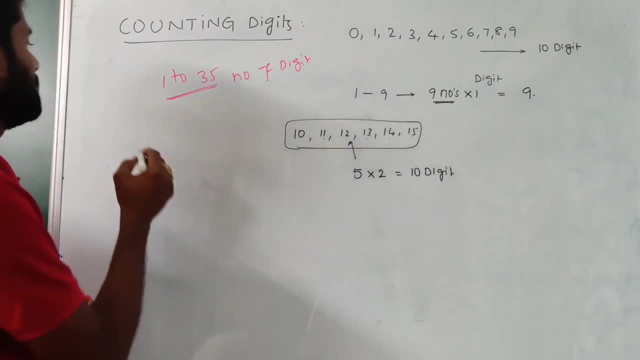 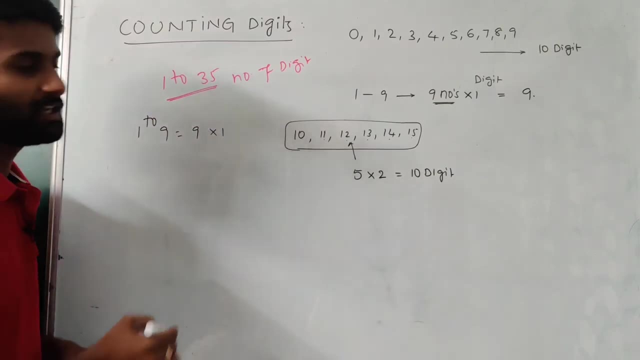 find the number of digits in the given one. First of all, see focus on 1 to 9.. 1 to 9, we have a 9 numbers. So by making 9 numbers they are using 1 digit. So 9 into 1, they are using. 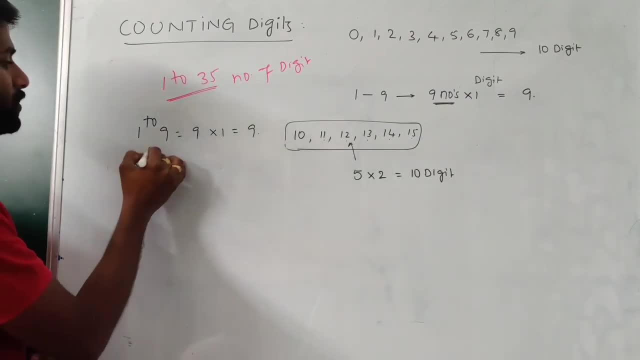 total 9 digits. See from 10 to 35.. So 10 to 35, first check it out. how many 2 digit numbers are there? 2 digit numbers are 10 to 35. So 10 to 35, first check it out how many 2 digit numbers are. 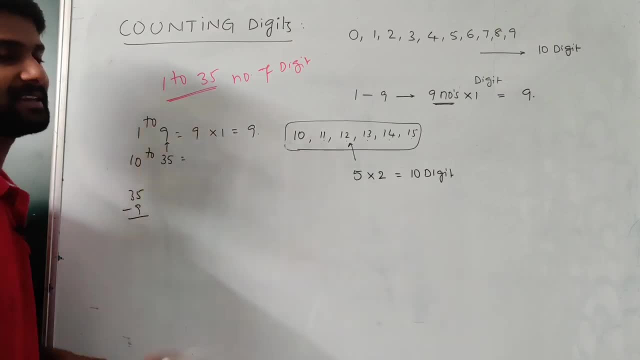 there 2 digit numbers. are there 1,, 2,, 3,, 4, 5.. So this 2 digit number means simply 35 minus 9, subtracted these minus these value, So 35 minus 9, the value become 26.. Means the total number. 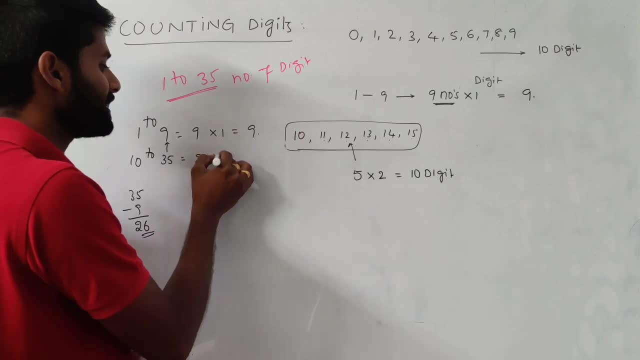 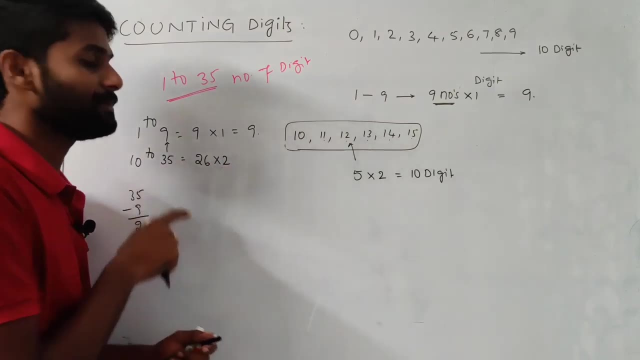 of 2 digits are 26.. And each 2 digit number can using 2 digits. So by forming 10 to 35, they are using each time as a 2 digit. the total numbers are 26 numbers, So 26 into 2,. 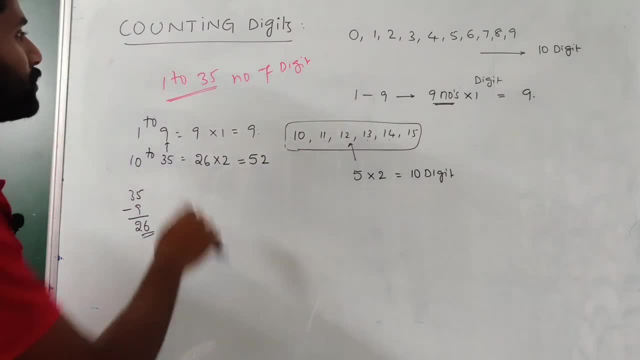 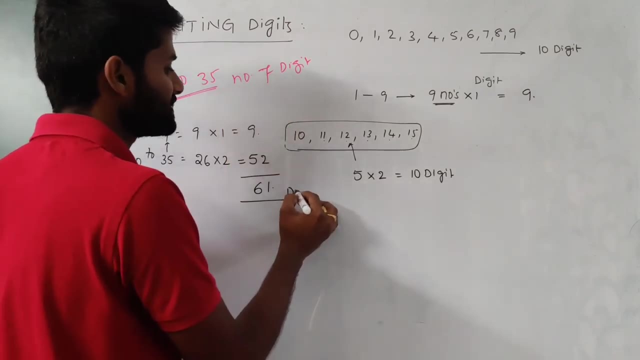 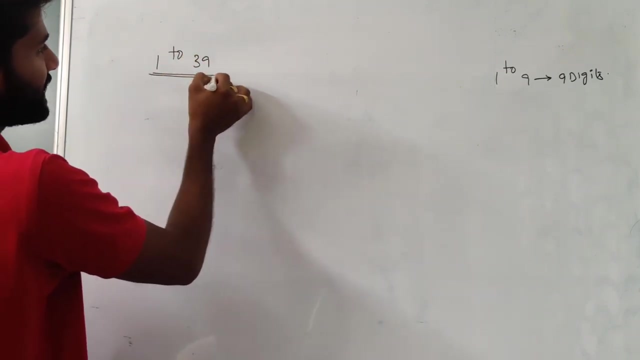 the total number of digits are 52. Here my question: 1 to 3, 35. I am using the total number of digits are 61 digits. That is the concept. So we will check one more example: 1 to 39. So if you form 1 to 39 numbers, 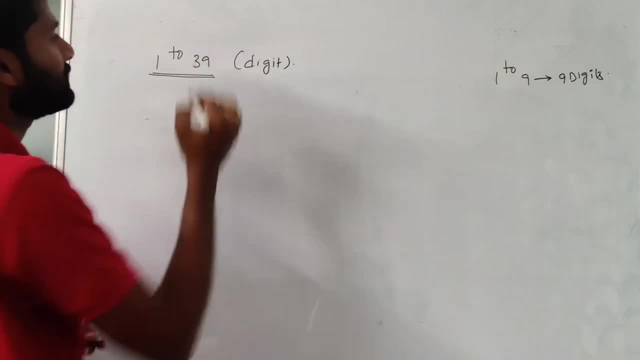 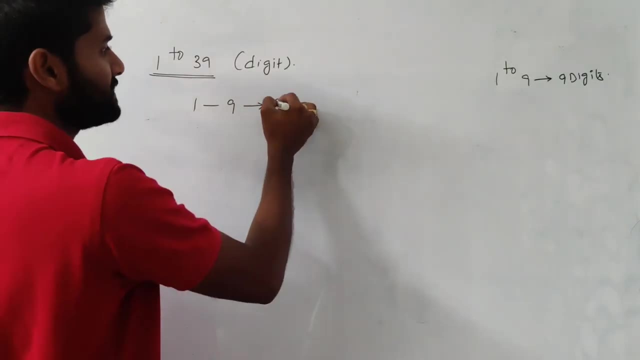 how many digits we are using. Find the number of digits in 1 to 39.. We know that 1 to 9, a single digit number, So we are using every time as a 1 digit means 9 into 1,. 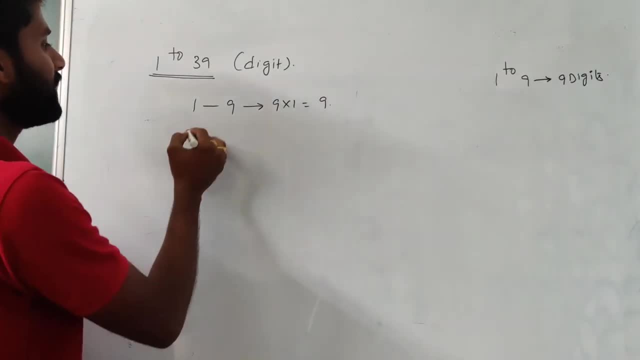 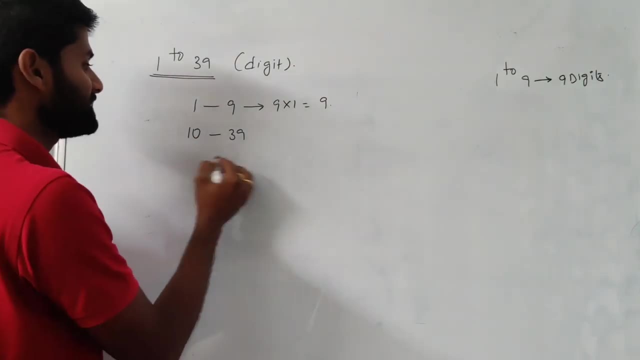 the total number of digits are 9 digits Clear From 10 to 39,. see from 10 to 39,. first of all, count it how many 2 digit numbers we are using. See simply 39 minus 9, we are using. 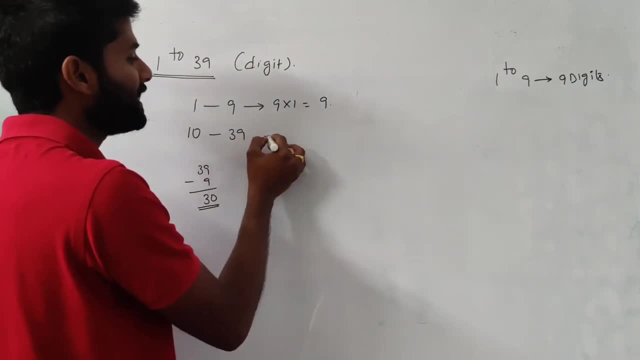 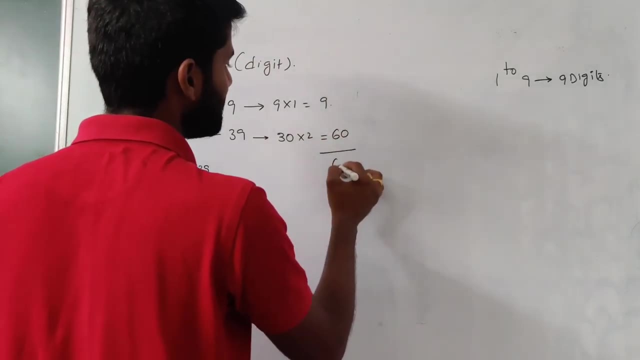 30 pair numbers And by forming a 2 digit number, every time we are using a 2 digits. So 30 into 32, 32 is a 60.. By making from 1 to 39,, we are using 69 digits. 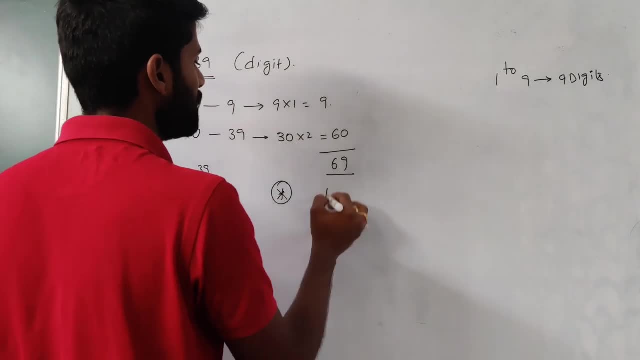 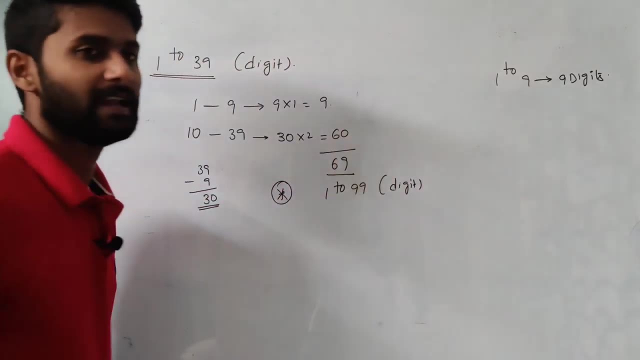 Okay, Same question, for example. one more example: 1 to 99,. 1 to 99,. find the number of digits in 1 to 99. Same concept, just see. So, first of all, 1 to 9, the total number of digits are: 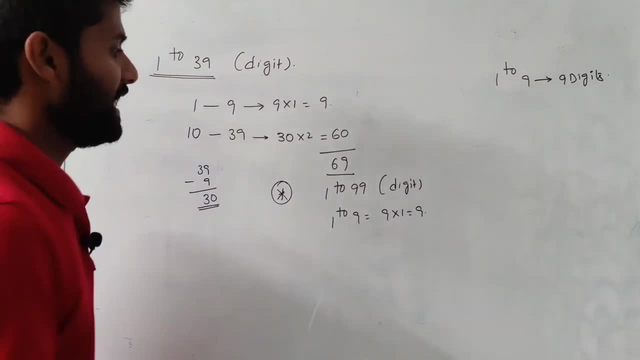 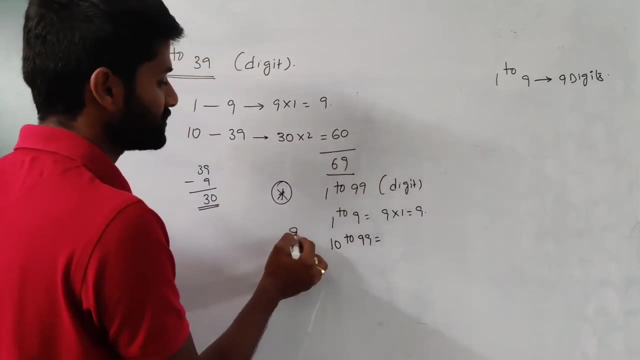 9 into 1, exactly equal to 9.. And the same thing from 10 to 99,. from 10 to 99,. first focus on how many 2 digit numbers are there. So 99 minus 9, the value become. 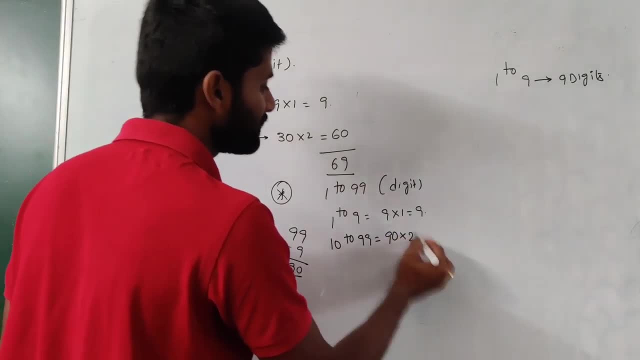 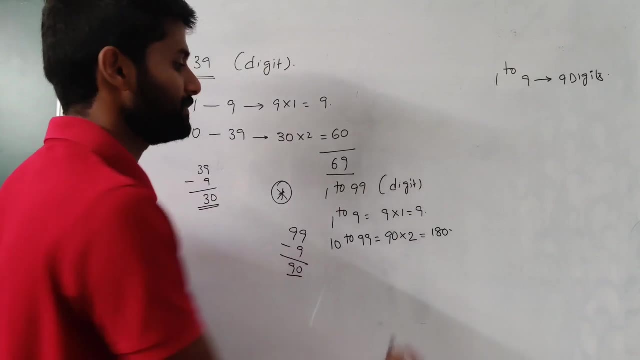 99.. 99 minus 9, the value become 99. And if you are framing a 2 digit number, definitely it consisting of 2 digits from every time. If you form 90 pair means we get 180 digits. Means the total number of digits from 1 to 99. 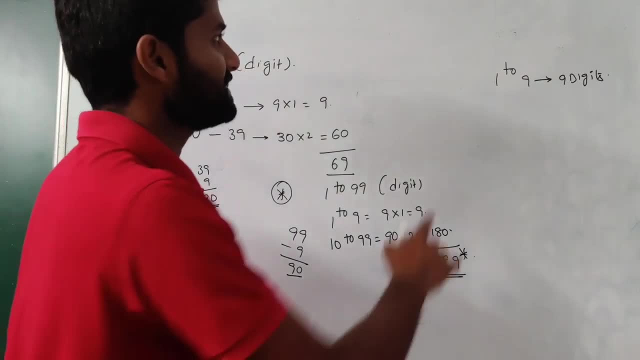 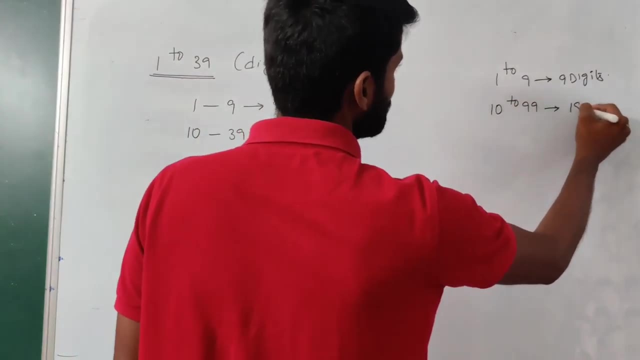 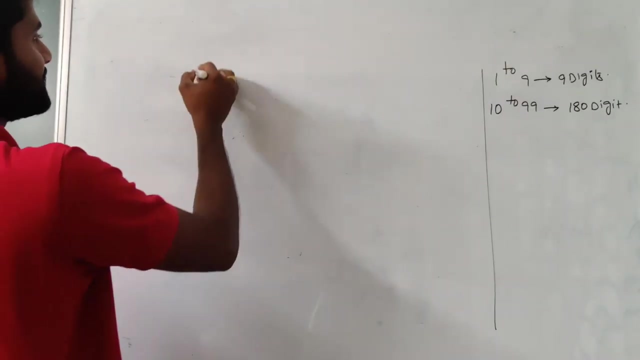 is equal to 189.. Let us see from 1 to 9,. we have a 9 digits. From 10 to 99, from 10 to 99, the total number of digits are 180 digits. Clear, Okay. let us see 1 to 129, find the number of digits in these numbers. Okay, we will go. 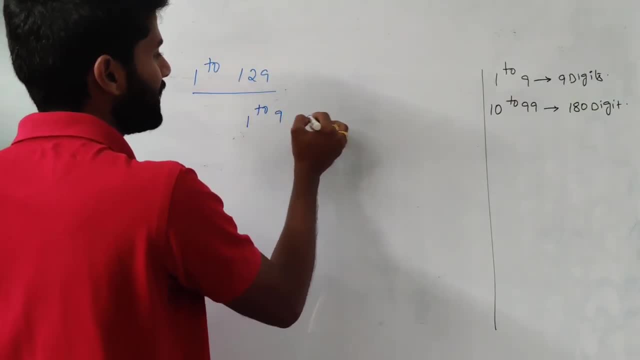 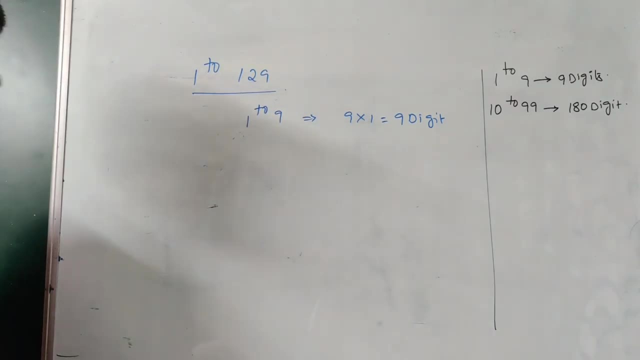 with the same approach. We already counted 1 to 9,. we are using 9 into 1, exactly equal to 9 digits. We are using 9 digits to make 1 to 9 numbers From 10 to 99, we already calculated. 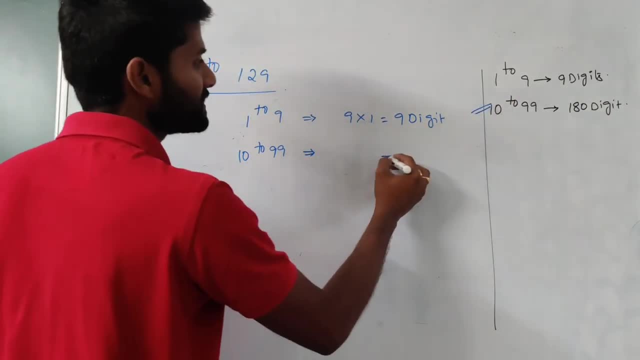 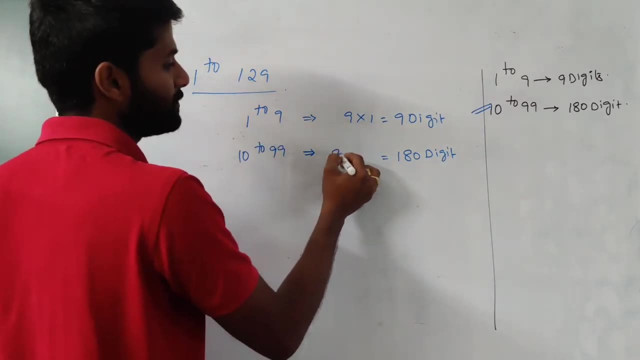 10 to 99, the number of digits we are using exactly equal to 180 digits. If you want to count it, it means 99 minus 9. So the value become 90 into 2.. We require up to 129. Means. move on to that. 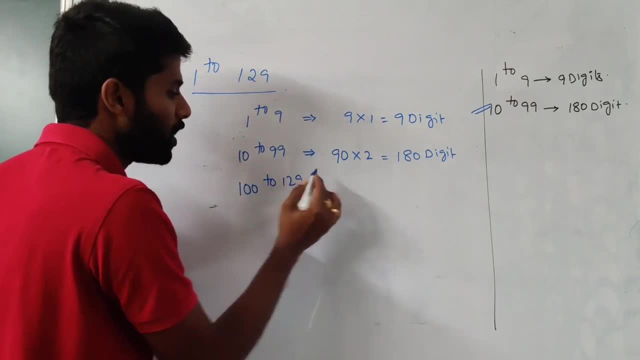 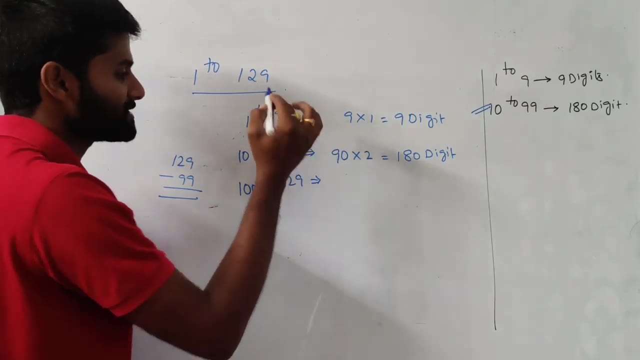 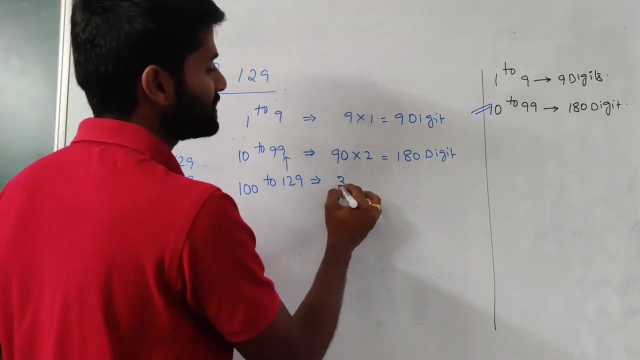 100 to 129.. First of all, how many 3 digits are there? See, simply, 129 is subtracted from 99.. Simply subtracted previous value. So 129 minus 99, we are using 30 digits, So we are using 30. 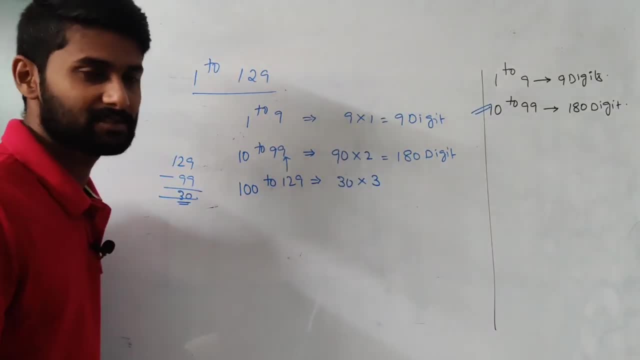 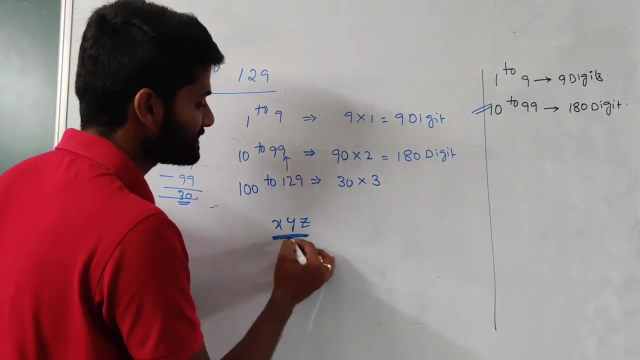 digits and each digit consisting of 3 numbers. 3 digit number consisting of 3 digits Means the x, y, z is a 3 digit number. So by making any 3 digit number, we are using 3 numbers. So same thing. So 30 into 3, exactly equal to 19.. 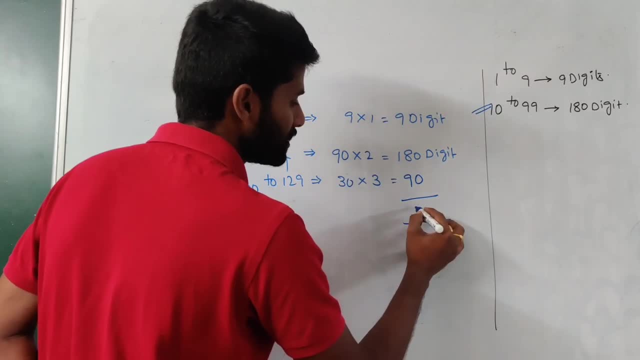 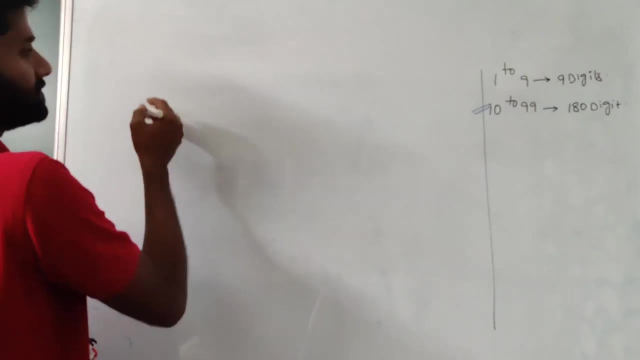 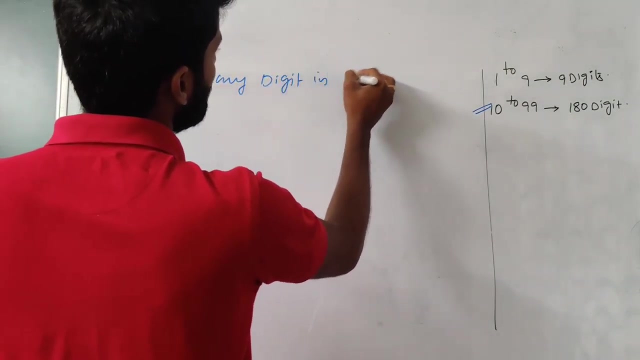 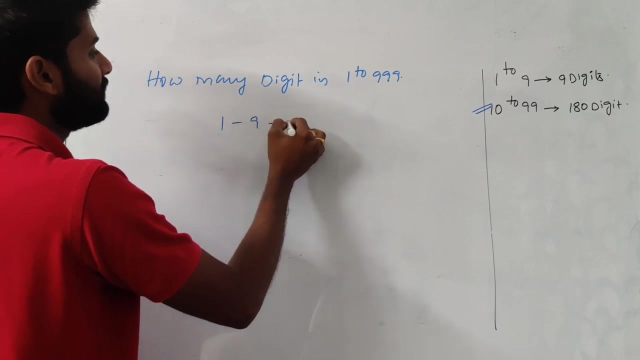 So if we count it as entire number, the total answer is equal to 279 digits. So this is the one more important. See the question: how many digits? How many digits In 1 to 999.. So this is our question. First, see simply 1 to 9, we have a 9 numbers Each. 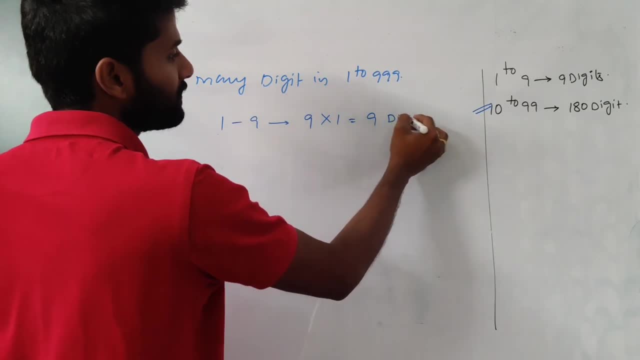 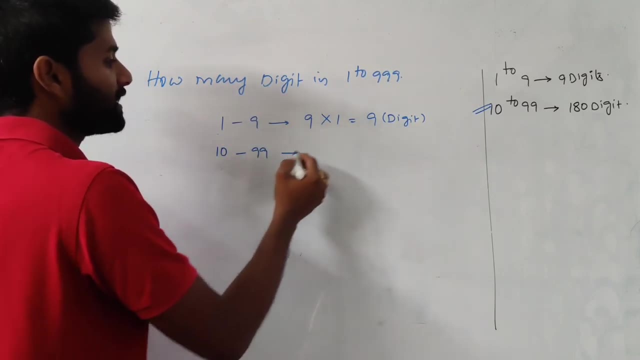 number having 1 digit, 9 into 1,, the total number of digits are 9 digits. Same thing if you go with a 10 to 99,, 10 to 99,, the total numbers are 90, and each number consisting. 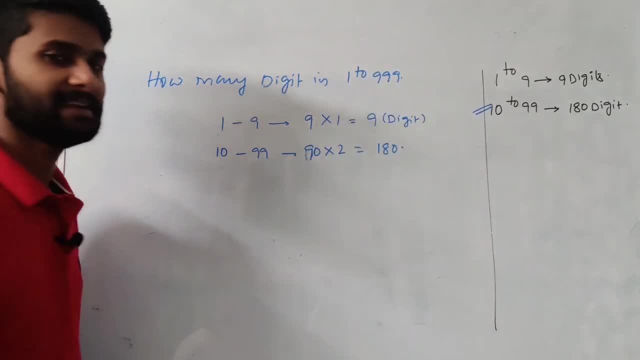 of 2 digits, and 19 2s are 180 digits. So this is our question. So if we want to calculate the total number of digits, how many digits? 10 to 999.. So this is our question. So this is our question. So if we want to, 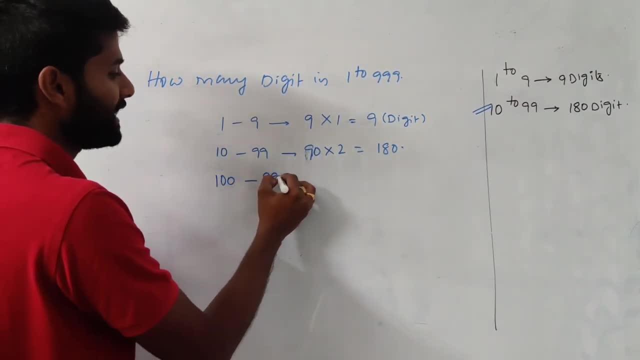 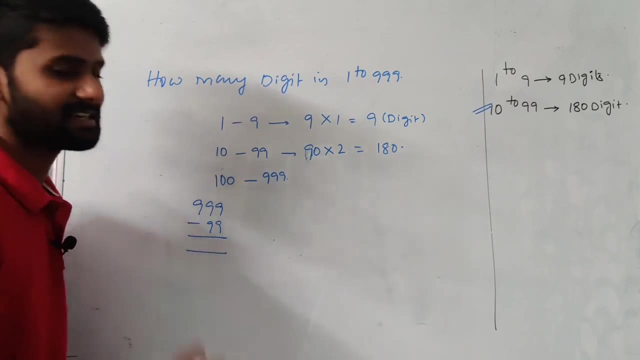 calculate the total number of digits. how many digits? 10 to 999, b 5 digit And the same thing, 10 to 999.. First, how many numbers we are forming? Simply 999-99.. You can simply subtract that these numbers, So 999-900, the total numbers we are framing. 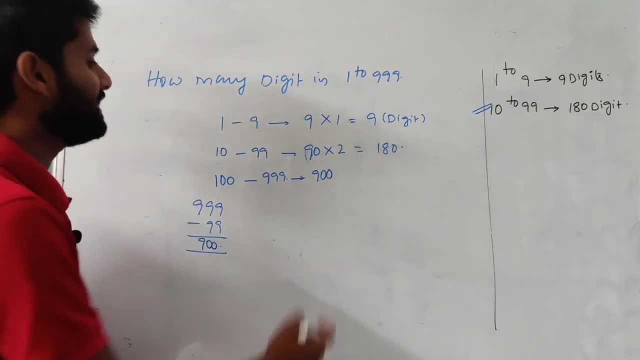 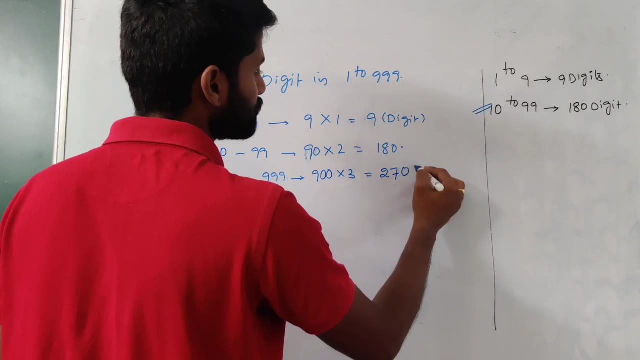 from these questions is 900 numbers And each number consisting of 3 digit number, So 900 into 3,, 900 into 3, the total numbers are 2700 numbers, So from 1 to 90,, 99,, 99,. 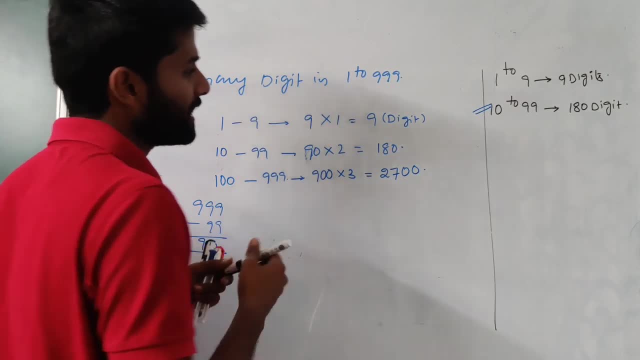 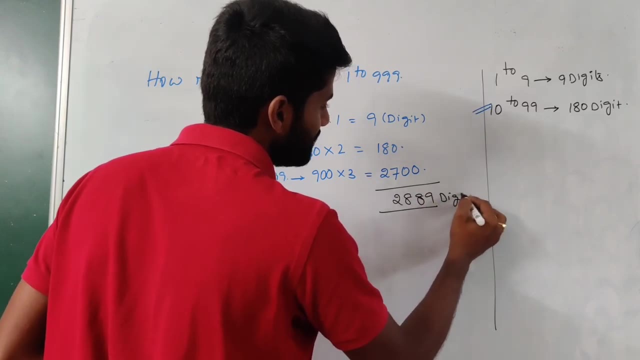 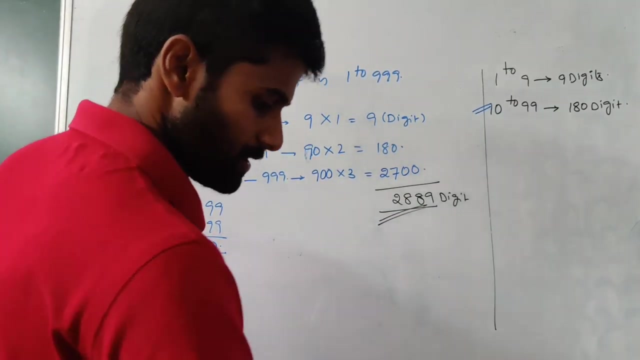 90, 99, 가능, And this number is 2 digits to 999,. the total number of digits: see 2889 digits. So that is your answer. The total number of digits from 1 to 999 is 2889 digits. Let us see the different example from this. 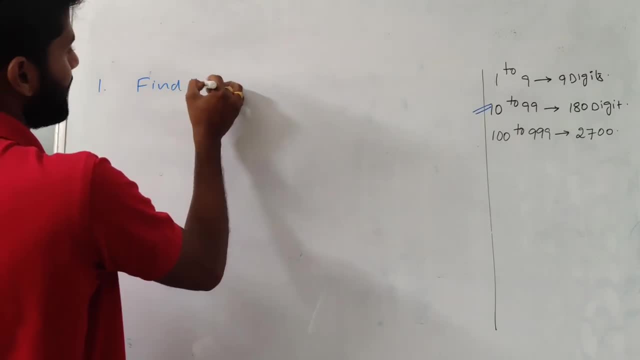 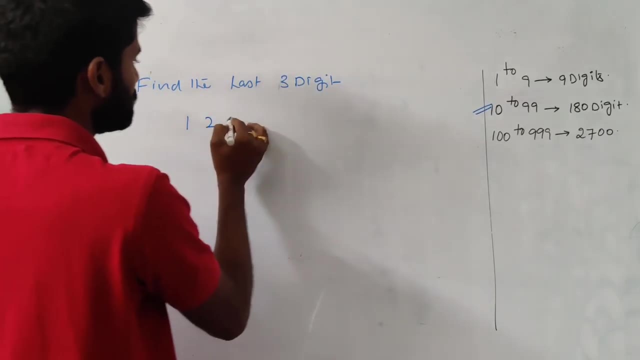 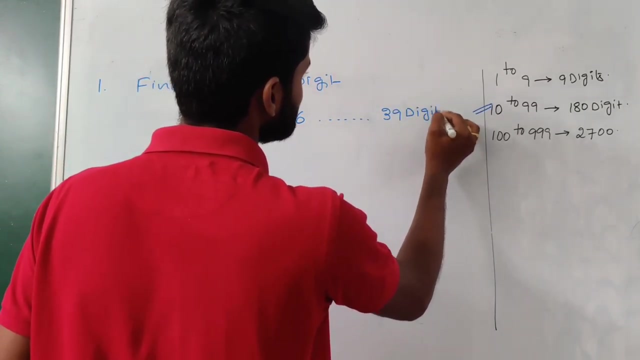 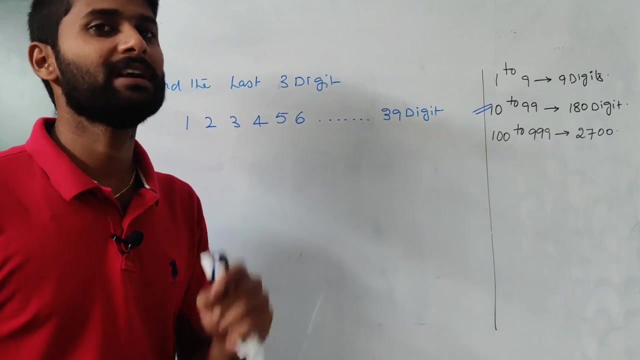 concept: Find the last 3 digits in 1,, 2,, 3,, 4,, 5,, 6,, up to so on 39 digits. So this is your question. First, see, we know that 1,, 2,, 3,, 4,, 5,, 6,, 7,, 8,, 9, all are single digit. 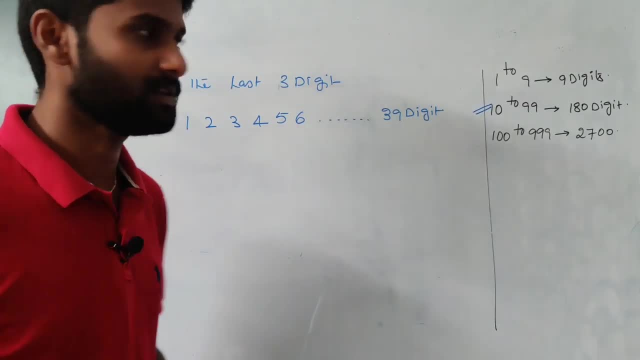 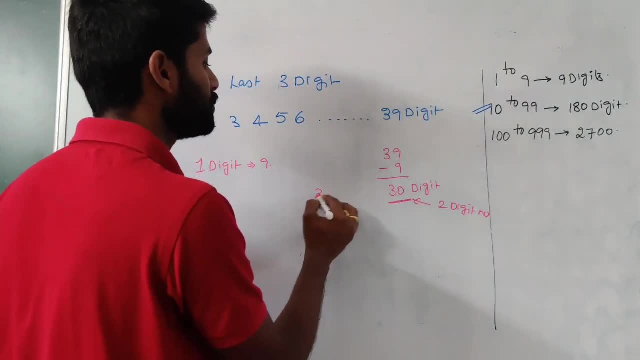 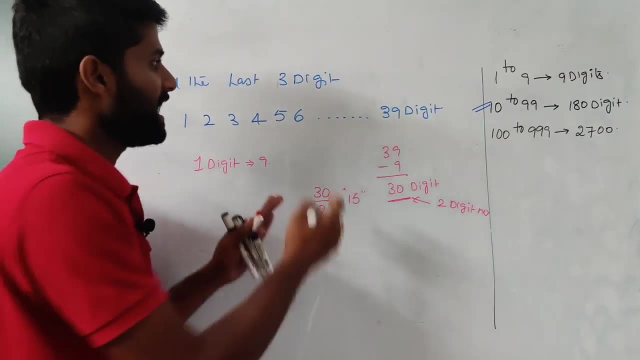 means it is consisting of 2 digits. Simply those value 30 divisible by 2, the value of final become 15.. That is your answer. See, after 9, we have a 15 pairs. See, we have not 15 digits, We have a. 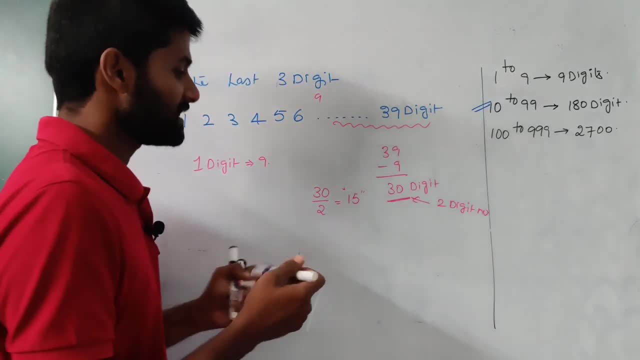 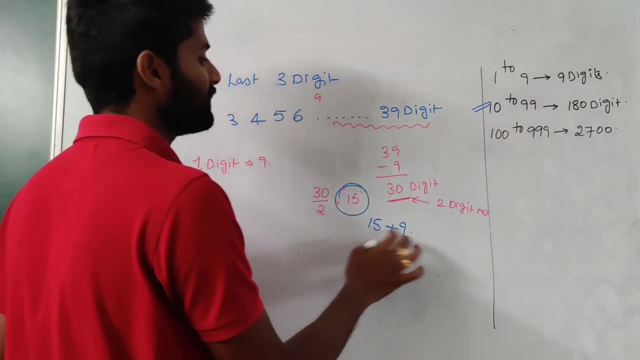 15 pairs If we want entire resultant means the 15 number. whatever the 15 number is added with previous number 9.. So 15 plus 9,, 15 plus 9, the value become 24th means the last 2 digits are: 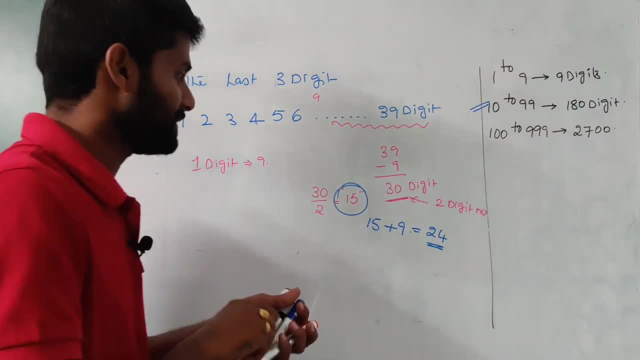 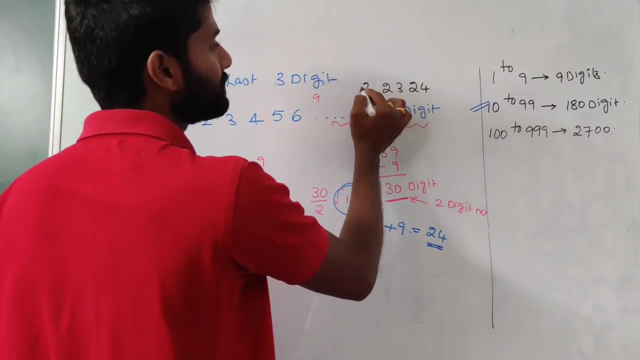 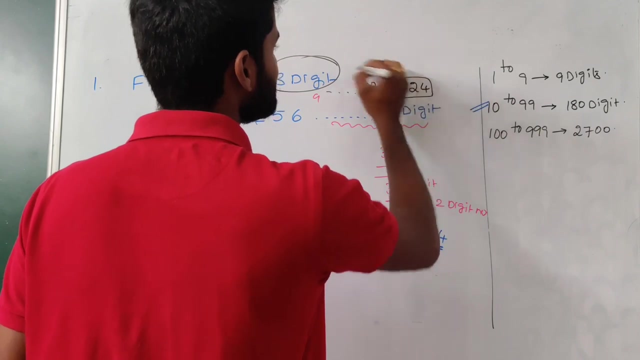 24.. It means the entire 39 digit, means the last digit is equal to 24.. The previous number is exactly equal to 23.. The previous number belongs to 22.. So here my question: what is the last 3 digits? Last 3 digits is exactly equal to 324.. So 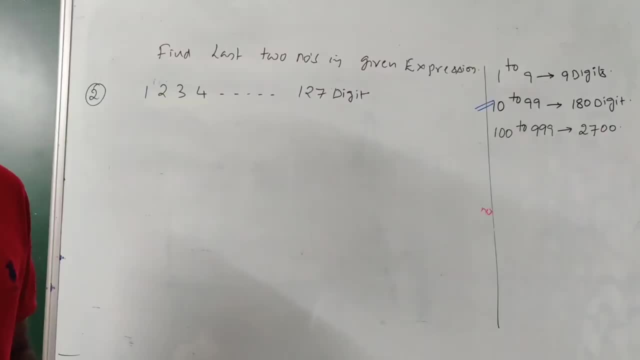 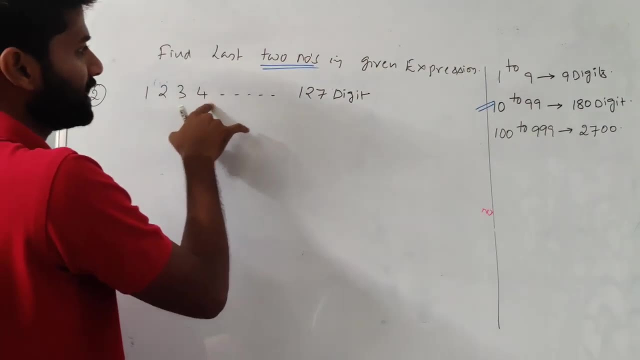 that is your answer. Let us see the question: Find the last 2 numbers. We need to find the last 2 numbers. The given expression is equal to 1,, 2,, 3,, 4 up to 127 digits. Not 127 is a number. 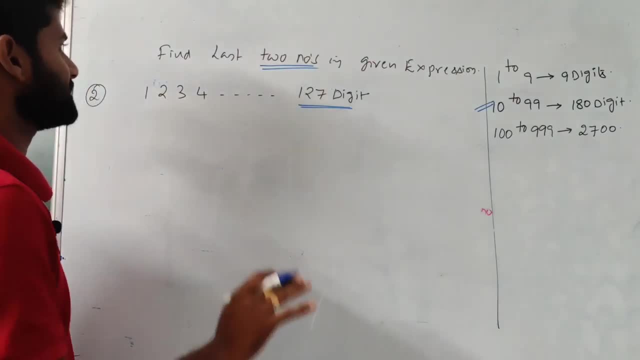 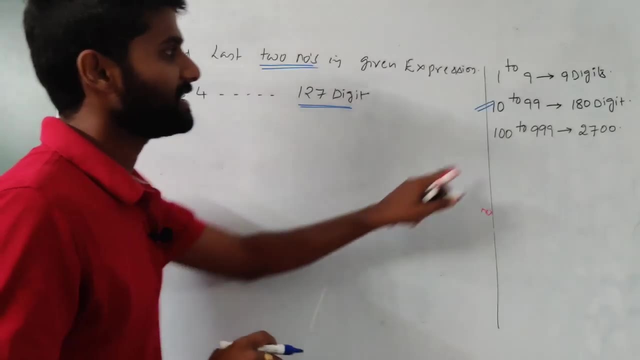 So they have 127 digits. First focus and see. So we have a single digit number is equal to 9 and remaining all the numbers are 2 digit numbers. Why? Because 10 to 99, up to we have 180 digits. 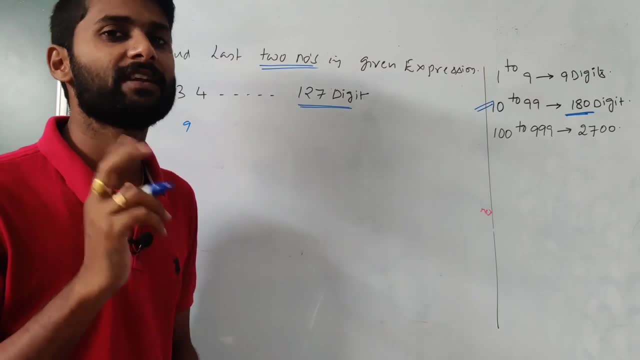 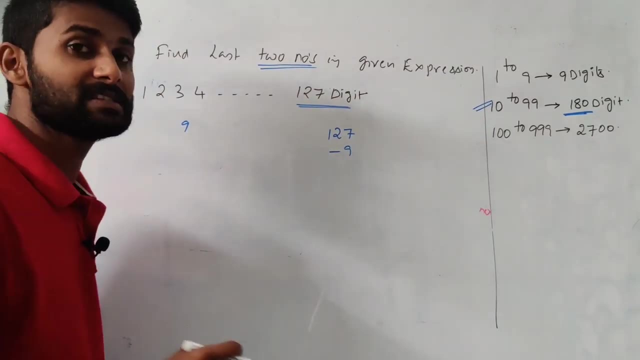 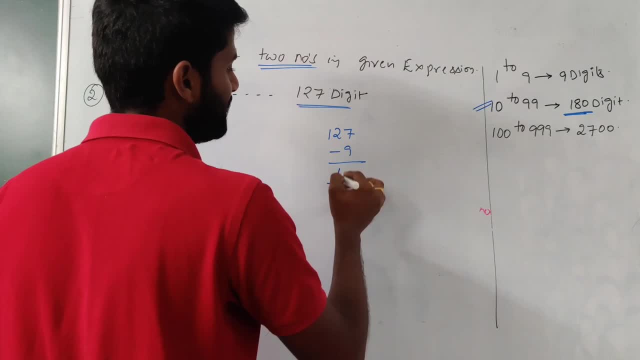 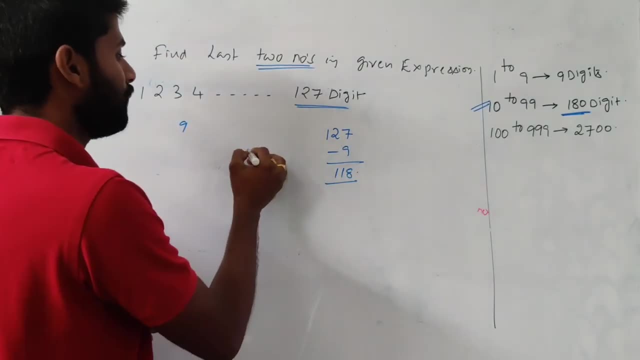 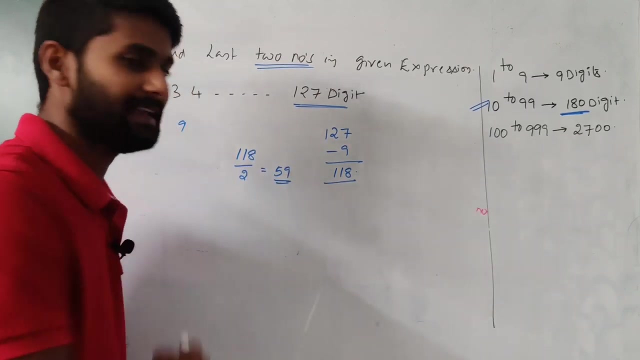 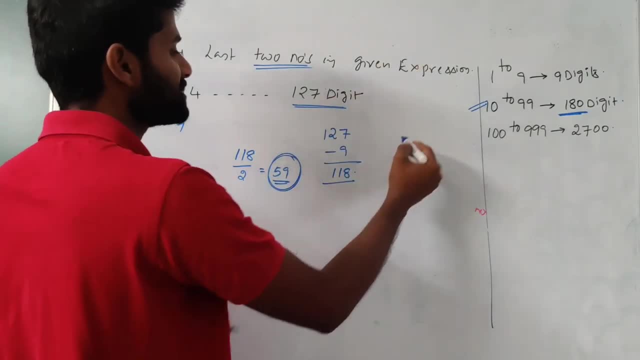 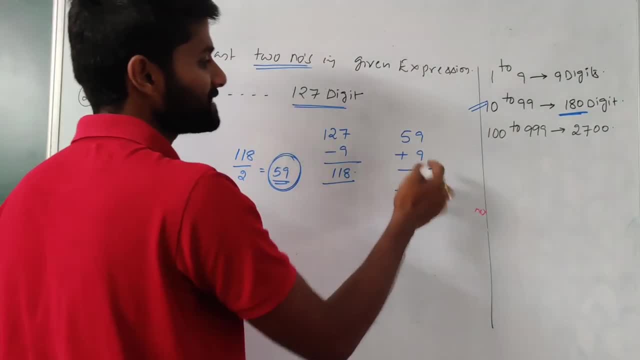 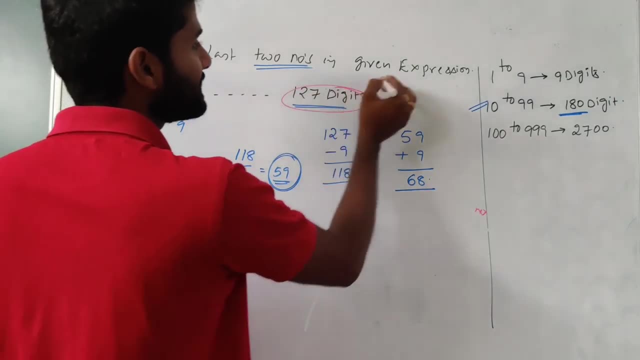 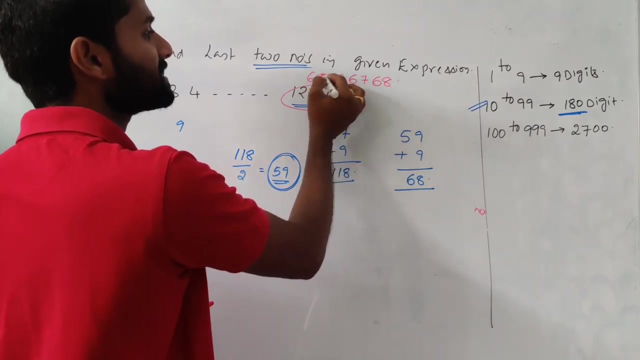 resultant of 9 means 59 plus 9. the total value become 68, means the last resultant. whatever. the last resultant is equal to 68.. If you want the previous answer: previous number 67, previous number 66, previous number 65, so on- In this question we need to find the last two digits. 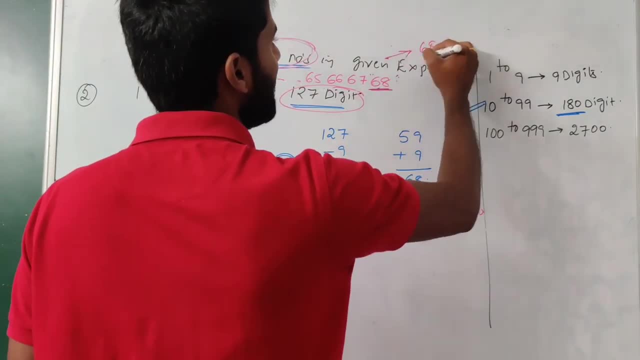 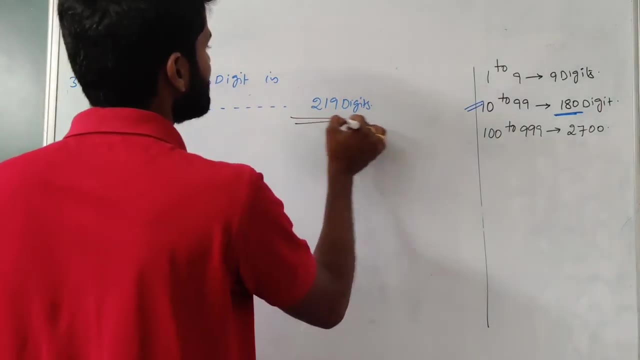 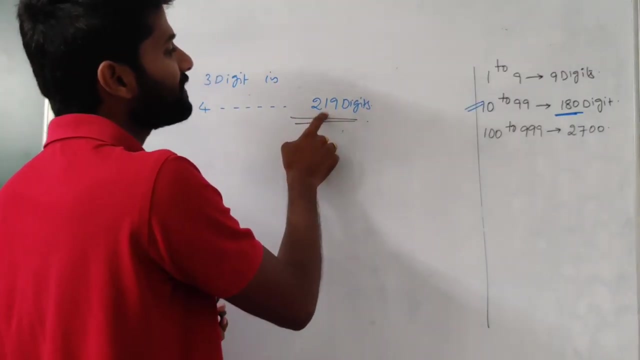 last two digit number is equal to 68. that is your answer. See, if number of digits are 219 digits, we already know that 1 to 9, 9 digits, 10 to 19 and 180 digits. so if they given for 219 digits, definitely. 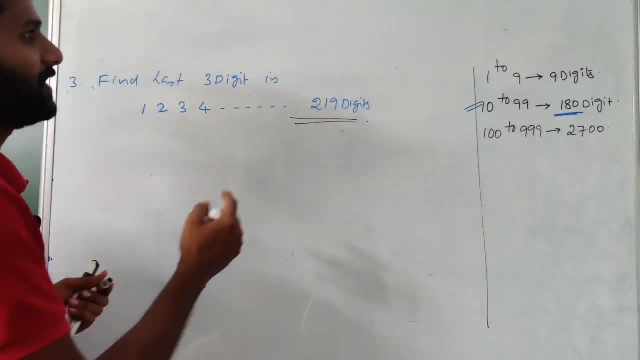 it is a 3 digit number. So how we are focusing, see, we already know that 1 to 9, we have completed 9 digits. then 10 to 19 digits, we have completed 9 digits. So how we are focusing, see we already. 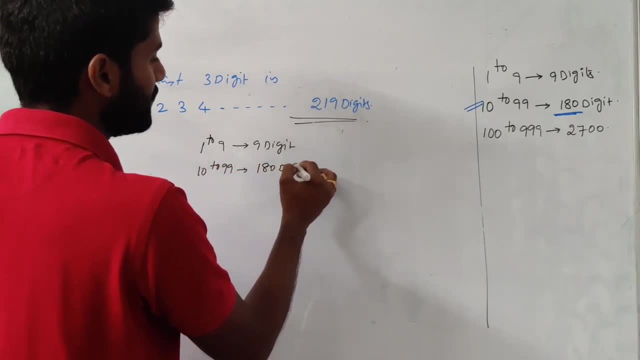 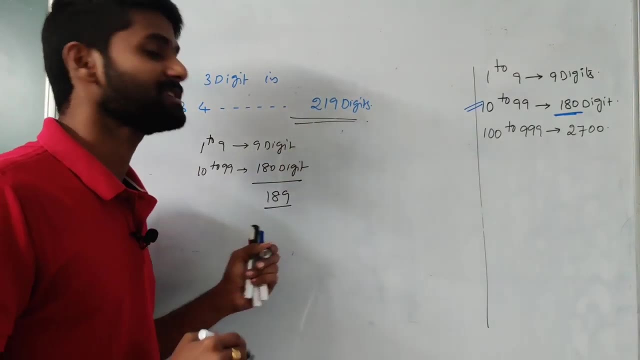 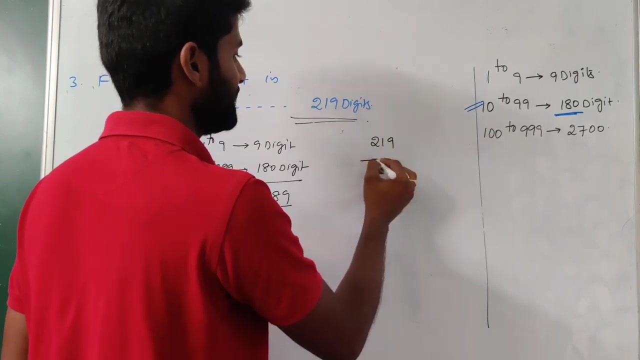 know that 1 to 9, 9 digits we have completed. 10 to 19 we are completed. 180 digits means 189 digits is a combination of single digit and a two digit, and remaining all the numbers are 3 digit numbers. Just for cut sense, after 189, how many digits we are left means 219 is subtracted as: 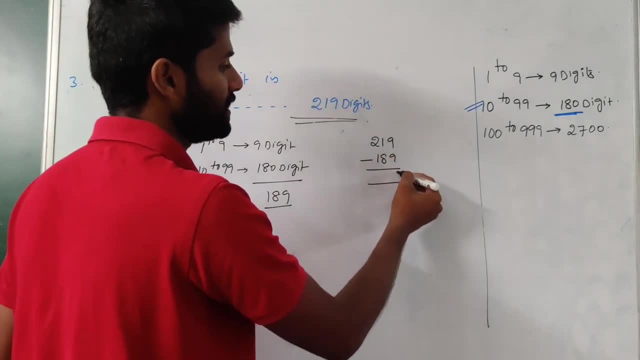 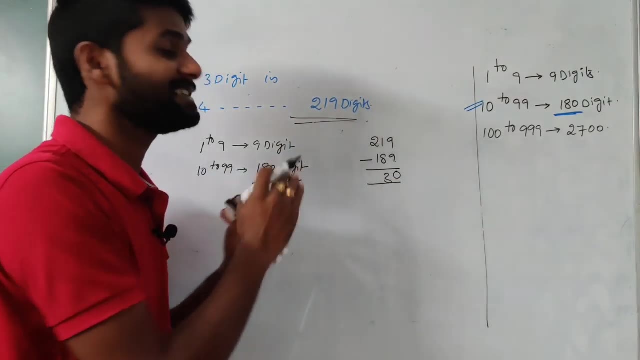 189.. So if you subtracted these value, it says 0 and a 30 numbers. So these 30 numbers is a part of a 3 digit numbers, means it consisting of 3 digits. So if you subtract these numbers, 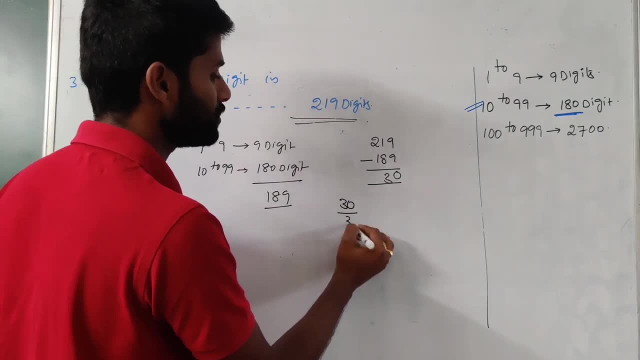 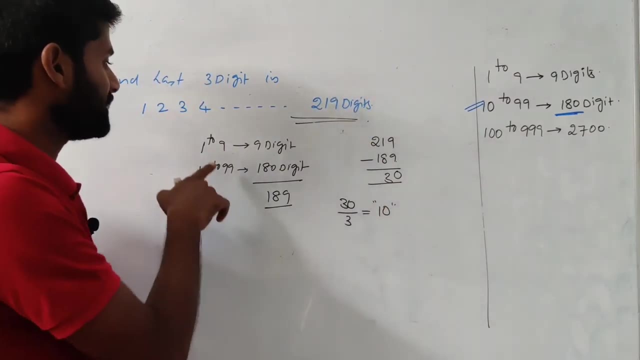 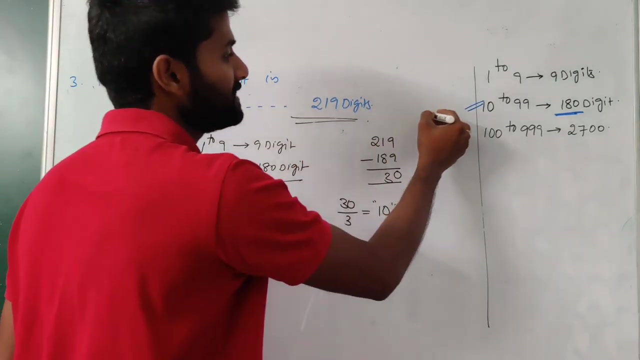 of three variables. That is why 30 divisible by 3.. So the total number of three pair numbers are 10 only, And we already know that the single digit highest number is a 9,. two digit highest number is 99.. After 99, we have a 10. numbers means 99 plus 10, the exact resultant is equal to. 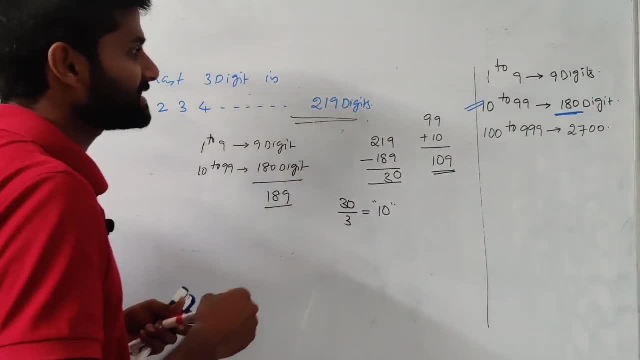 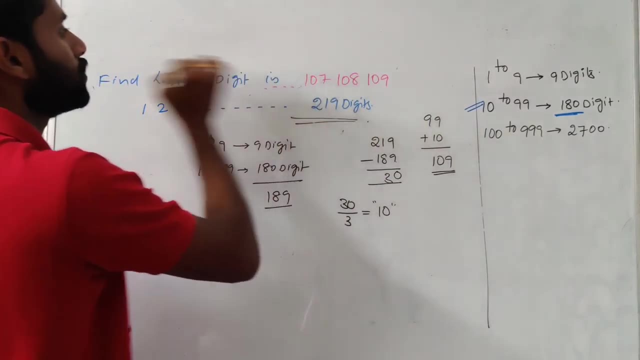 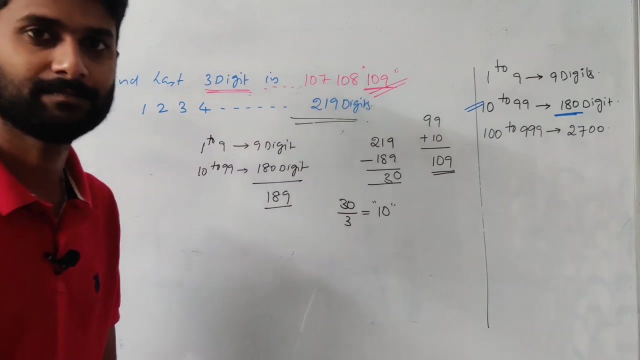 109. Means last digit of a number is equal to 109 and the previous number 108, the previous number 107, so on. He said that what is the last three digit number? What is the last three digits here? 109 be the answer. See, if they given for number of digits greater than 180, you need to. 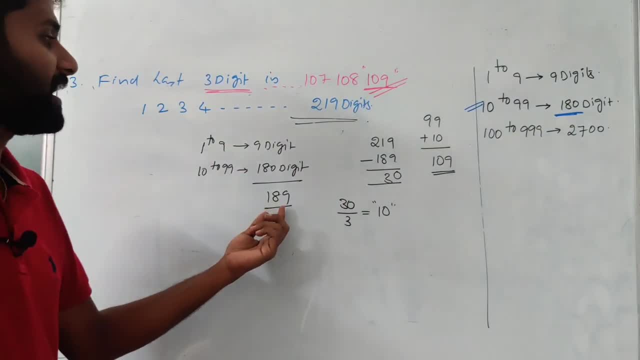 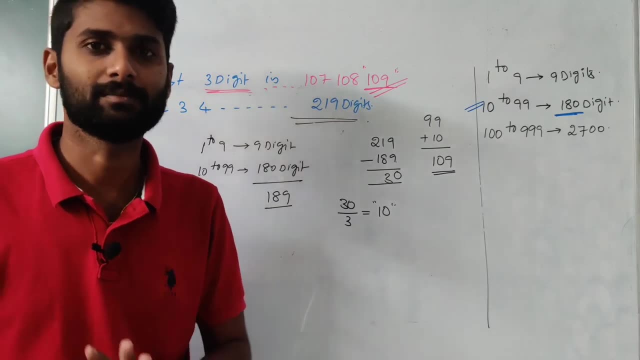 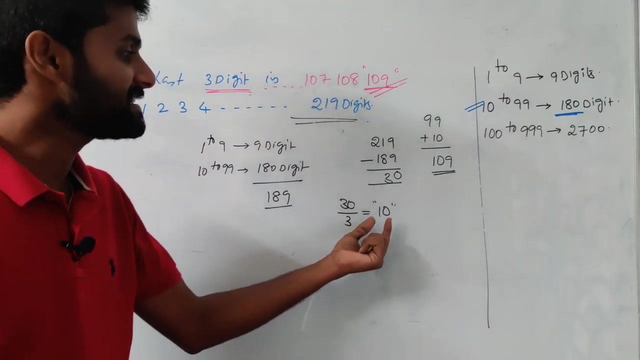 recognize that there is a three digit number. That is why the 189 is subtracted from 299, we get it So 30 numbers. those 30 numbers is related to three digit number. That is why those 30 is divisible by 30, we are forming a 10 three digit number And these 10 numbers we are added after. 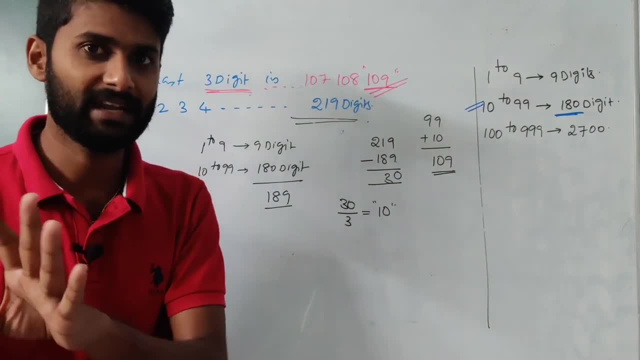 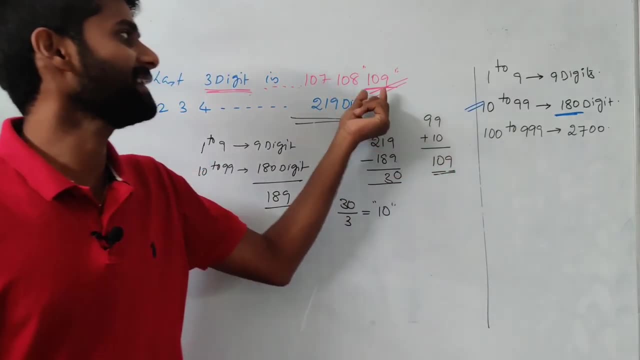 99.. Why? Because the two digit highest number is equal to 99, we simply add 10 into the 99,. the entire resultant is equal to 109.. So these number can exactly indicated a last three digit number. See same model they given in terms of reminder. Find the reminder. 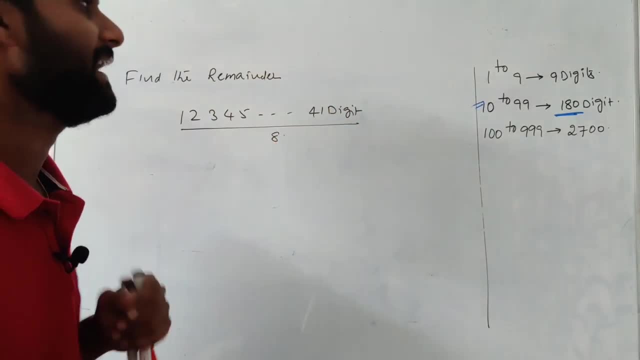 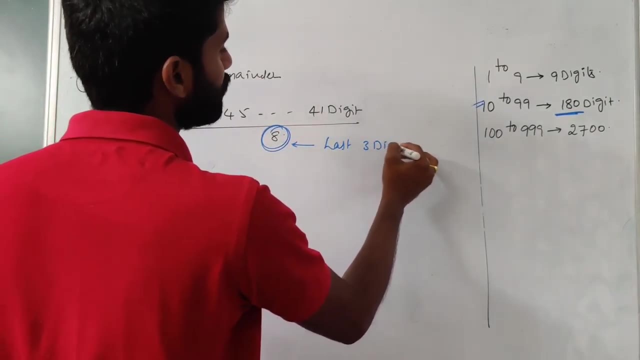 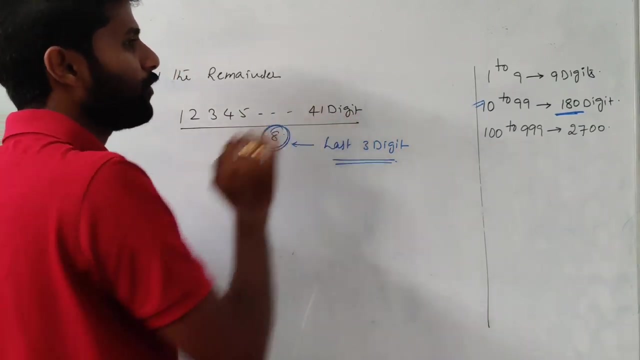 there is a 41 digit number which is divisible by 8.. See if divisible by 8 properties is focus on last three digits. if you focus on last three digits, we get the direct reminders. See the total. we have a 41 digits out of 41 digits. we have a nine single digit number. 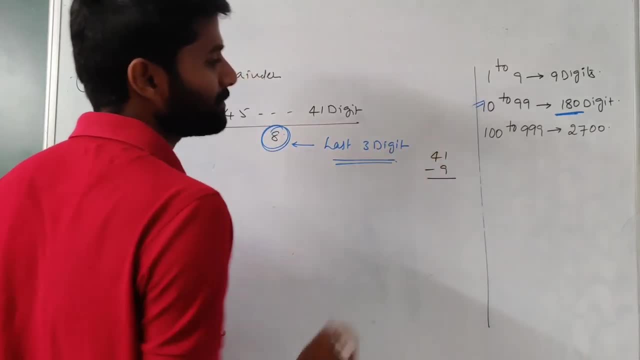 that is why 41 is subtracted from 9,, 41 minus 9,, the value become exactly 32.. Means 32 digits which are consisting of a two digit number. How many are remaining? OK, So the total is 31,. 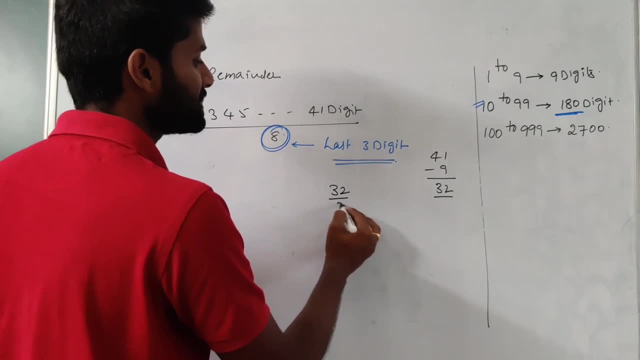 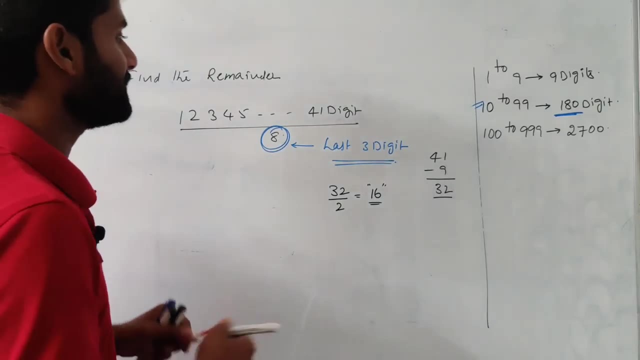 which are OK. So come one, guys. this was a great one because we became the first exam number. That is why 32 is divisible by 2.. The total numbers after one digit is equal to 16 numbers. If we want result, it means simply 9 plus 16, the total value is equal to 25.. It means 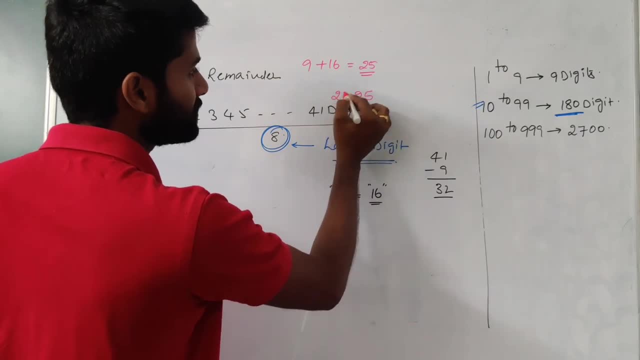 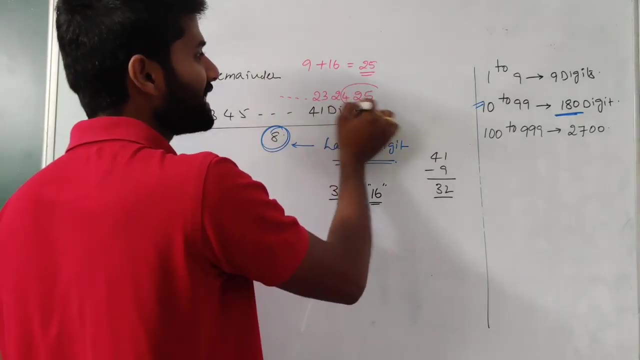 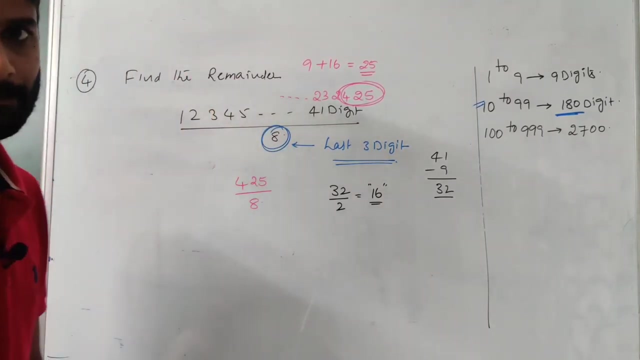 the last numbers are 25 and the previous number 24, the previous number 23,, so on. According to the divisible by 8 rule, you just focus on last three digits. See, if you focus on last three digits, it means 425 divisible by 8.. See what is the remainder here: 8: 1's are 8,. 8: 5's are 40,. 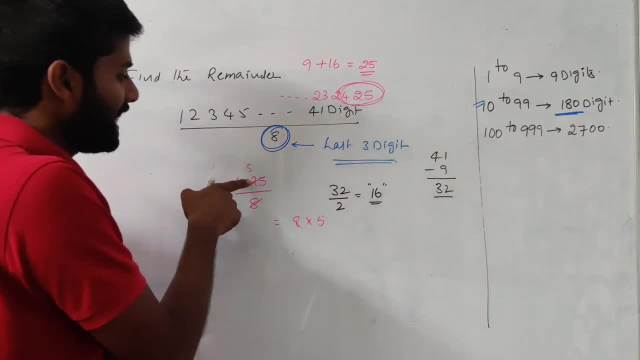 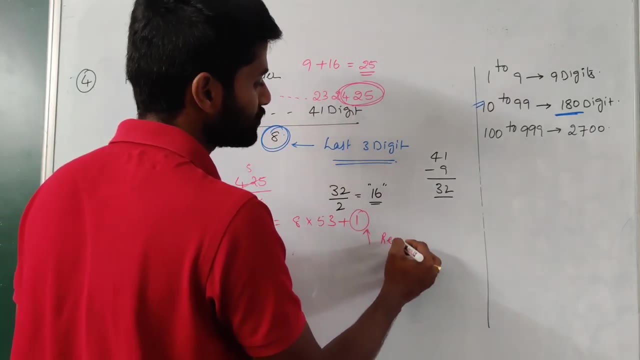 clear. So 8 1's are 8, 8 5's are 40 and we have 2 as a forward, and 8: 3's are 24 and we get 1 as the remainder Means those particular number is exactly divisible by 8, we get remainder with the. 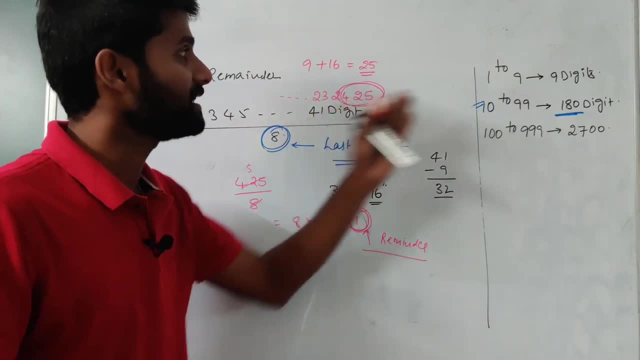 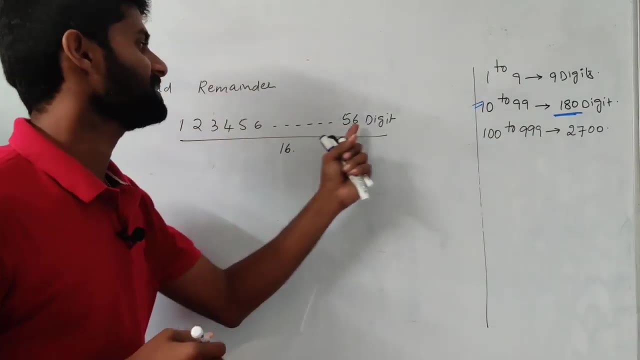 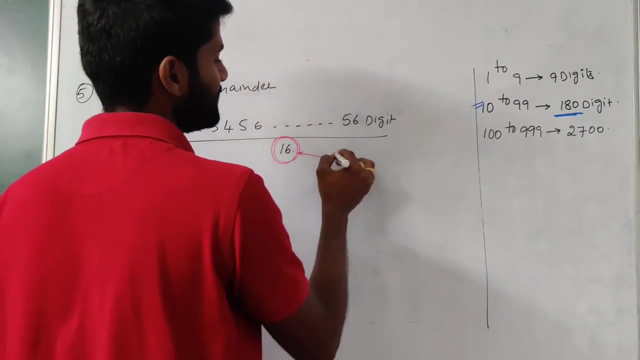 1. This is the important in digits concept: to focus on Number of single 1 digit, 2 digit and the 3 digits clear. See if find the remainder for these expression which is divisible by 16.. See first of all, focus on the 16 properties, The divisibility rule for 16, focus on last 4 digits. 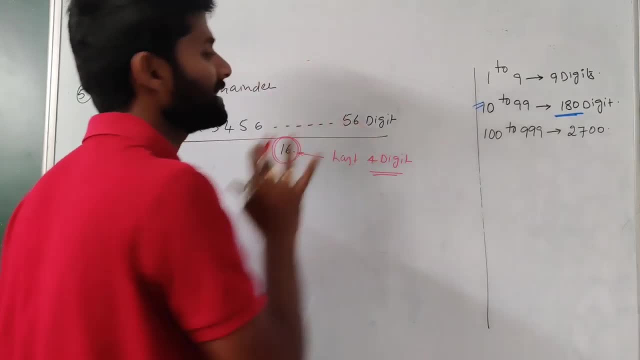 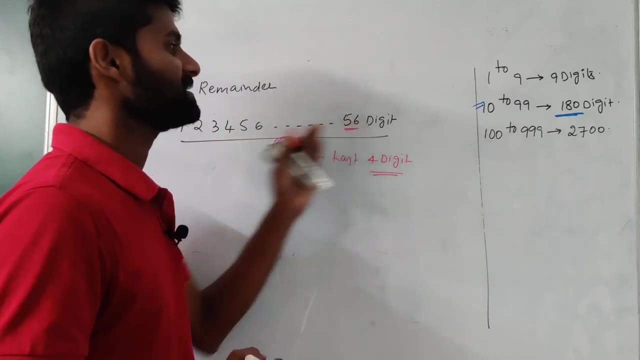 If you know the last 4 digits, we get the remainder for entire number. They given as a 56 digits. So 56 is subtracted 9.. So if 56 is subtracted 9, we get a 35. So 35 is divisible. 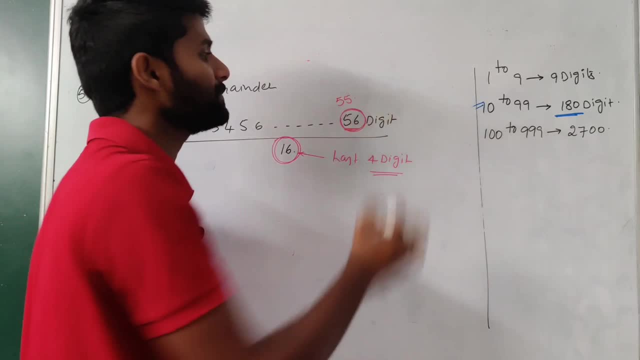 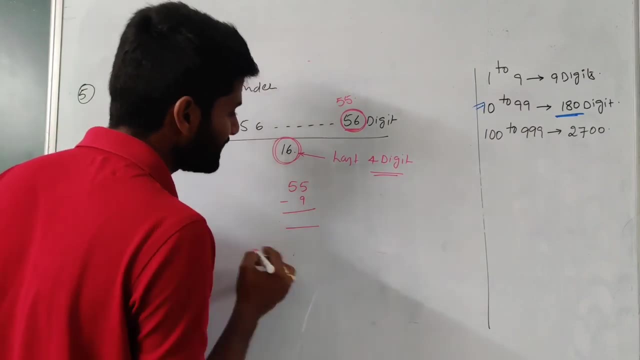 by 2.. So if I pick a odd number digit, I just pick a 55 in the previous digit, clear. Then same thing: 55 digits is subtracted a single digit number, we get the resultant is equal to 46.. 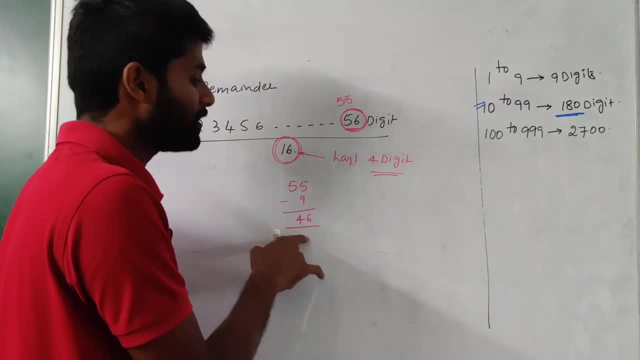 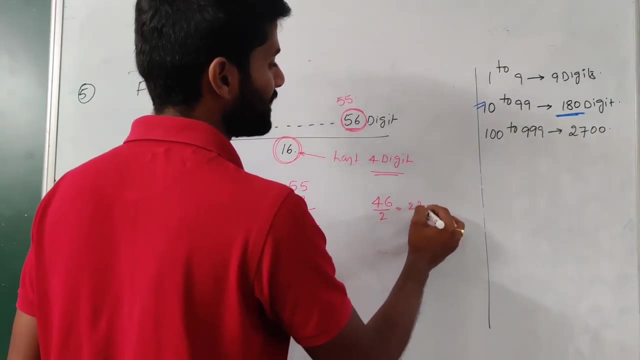 It means after single digit number, we have 46. 2 digit numbers are available, If you want. the exact number means 46 divisible by 2, we get the value of 23.. If you get 23 as a resultant- previously we have a 9 numbers- the entire number is equal to 26.. So we get the value of 23.. So 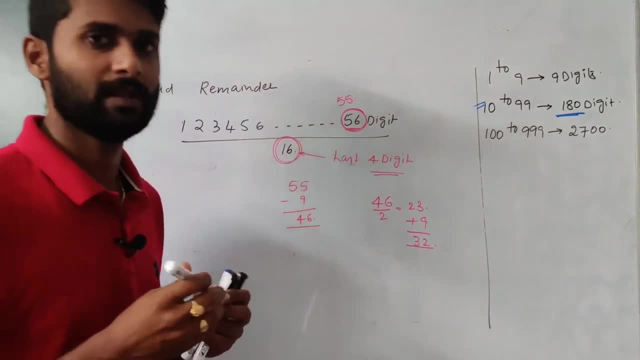 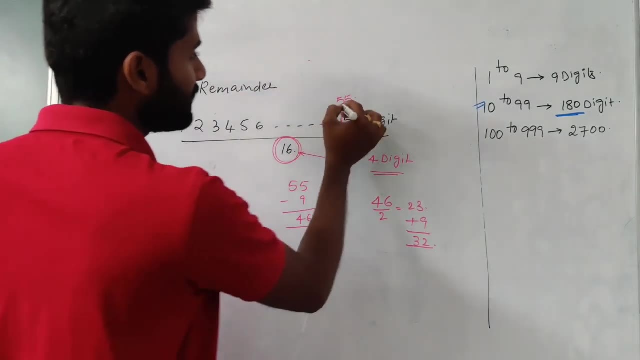 the resultant is exactly equal to 32.. Means this is the 32 number for 55th digit, not a 56th digit. See, if you want 55 digit, means 55 digit is equal to 33, then the previous number 31,. 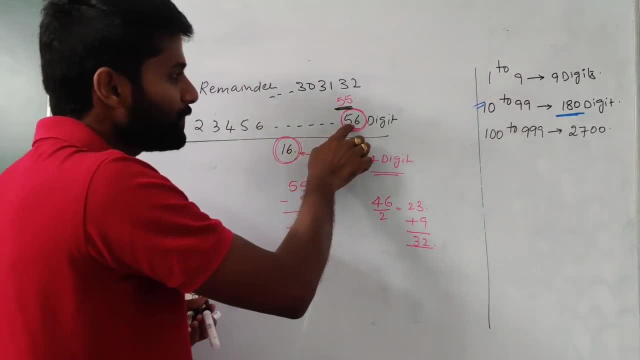 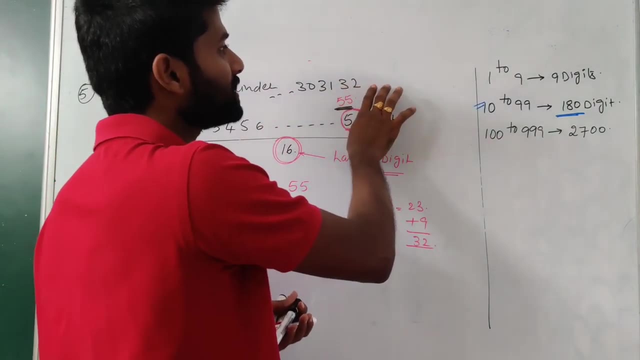 the previous number, 30, so on. But if you want a 56 digit means see, these are related to 30s, 31,, 32,, 33,, 34.. After 32, the next number is equal to 33.. But we required only 1 digit If 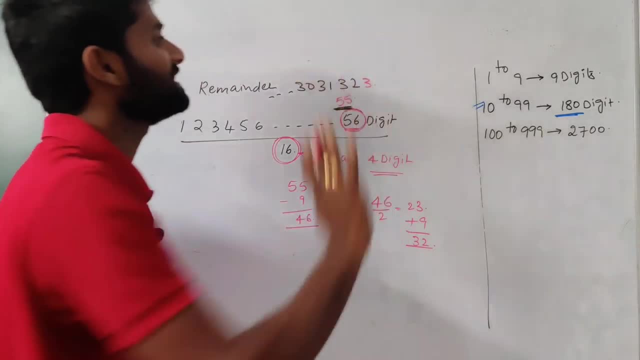 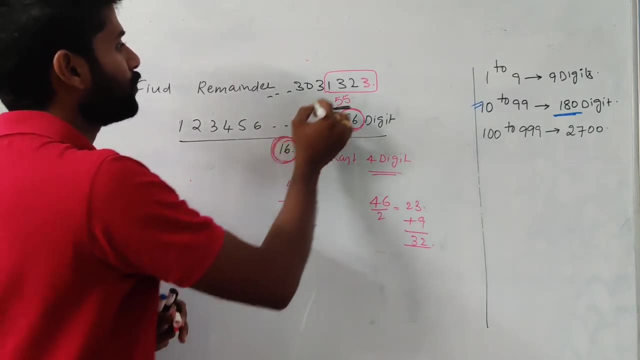 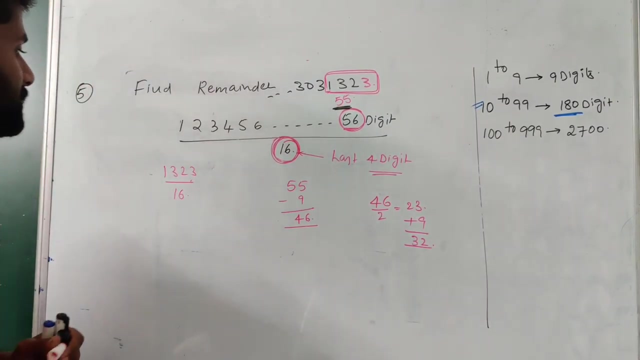 you required. only 1 digit means I just consider as 3 only. Then here my question: if you want these number which is divisible by 16 means focus on last 3 digits. What is the last 3 digits here? 1, 3, 2, 3 divisible by 16.. See: concentrated 16 become how many times 16? 8s are 128.. So 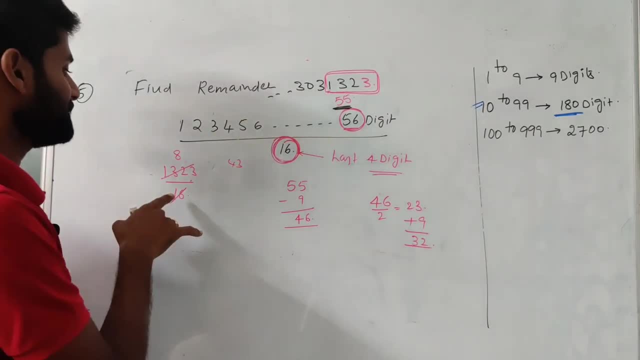 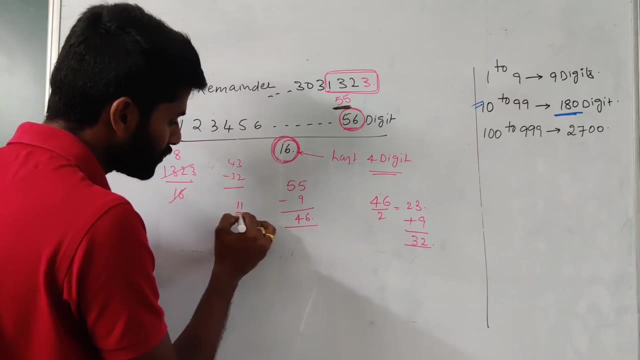 we left with a 43 as a reminder. And same thing: 16: 2s are 32,. 16 2s are 32, we get a reminder is 11. only It means if these entire number, which is divisible. 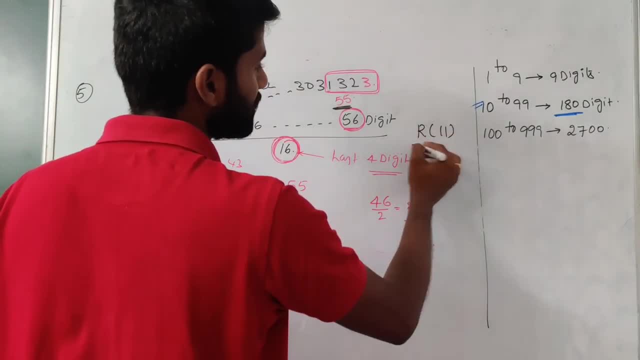 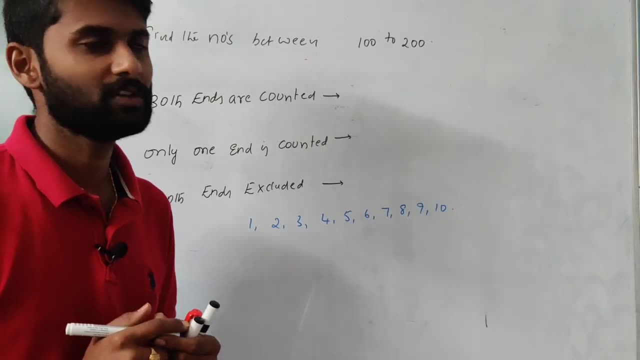 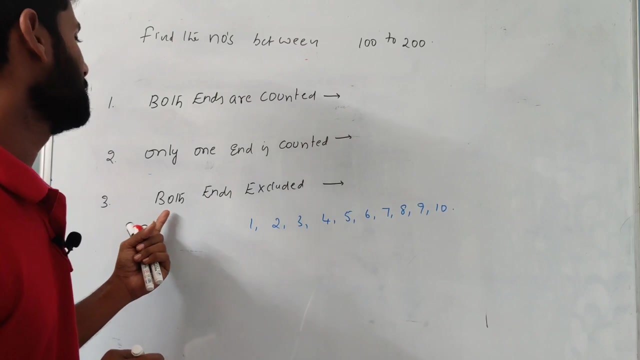 by 16,- we get the reminder- is equal to 11.. So these are the different models which are related to the digits concept. Next see find the numbers between 100 to 200.. How many are there? If both ends are counted? only one is counted and both ends are excluded. Before these example, I just 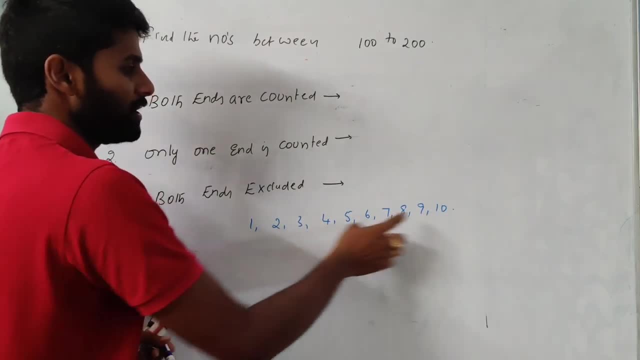 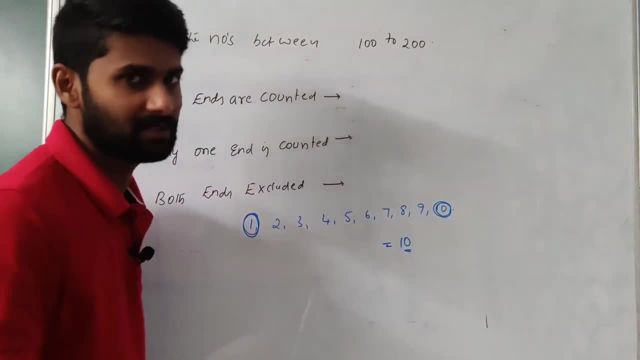 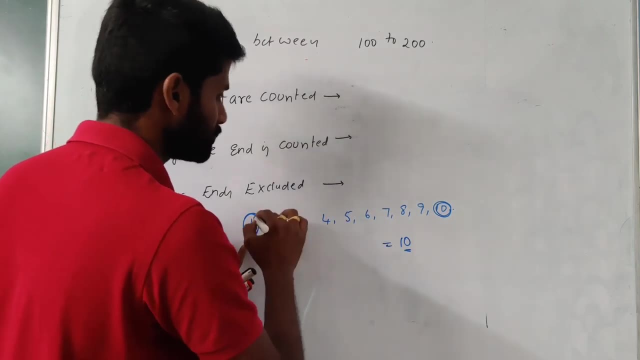 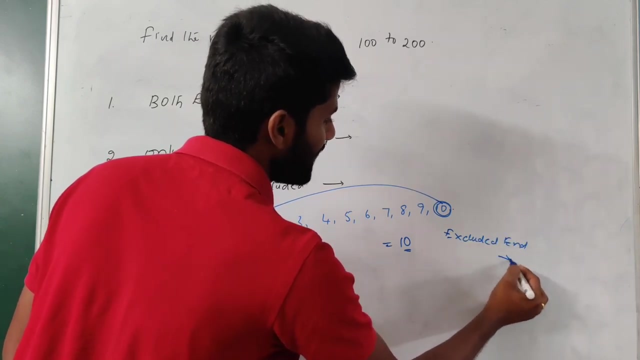 including first number and we are including last number, clear. For example, if you excluding these two numbers, If you excluding these two numbers, the total. if you excluding ends, the total numbers. if you excluding ends, we have a 8 numbers. If both are including we. 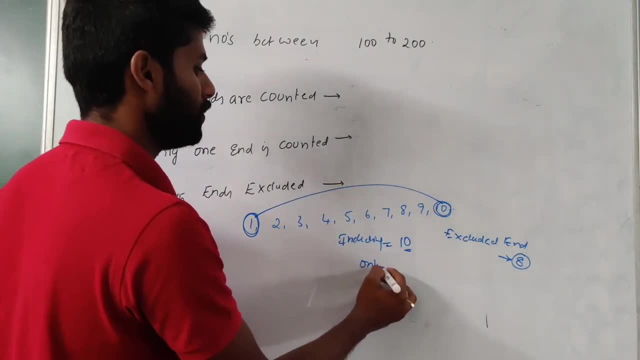 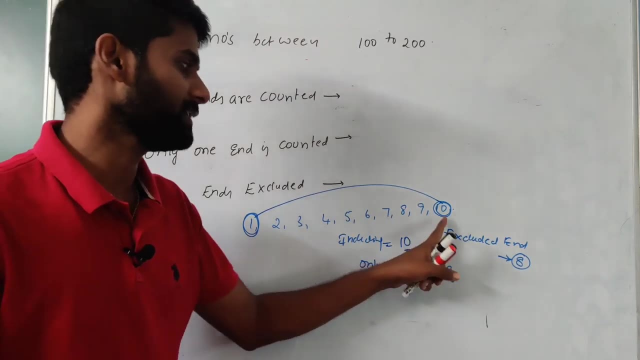 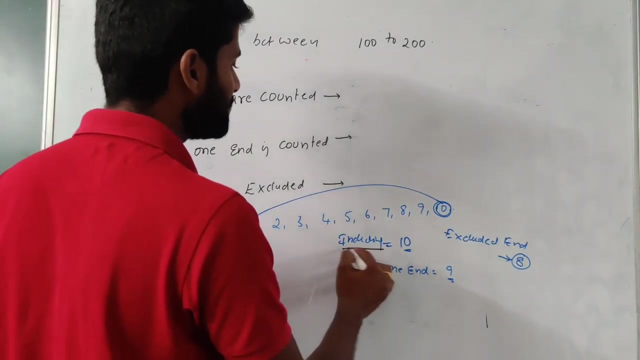 have 10 numbers. If only one end- only one end is including the total numbers- are 9 only means out of 1 or 10, you can consider only one particular end. These are the three examples. If you go with a direct approach, see if you are including the, both the numbers, if you are including both the. 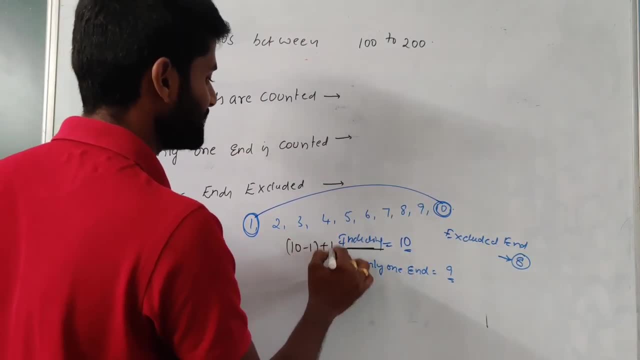 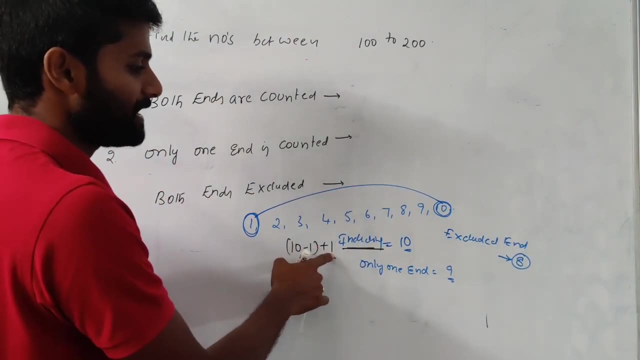 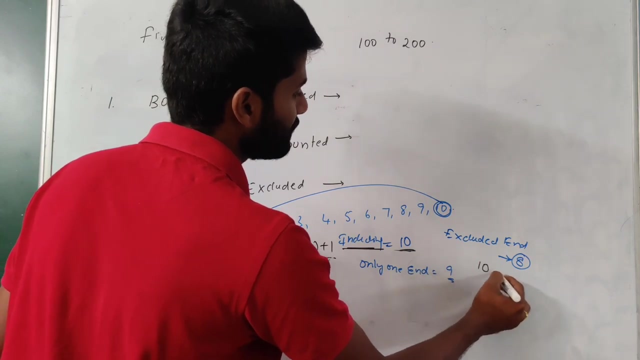 numbers means 10 minus 1 plus 1. that is the theory. So we can subtract final number minus initial number. we can add with a 1: 10 minus 1 plus 1. the total numbers are 10 only If you excluding both the ends. if you excluding both the ends means final end minus starting end, we can. 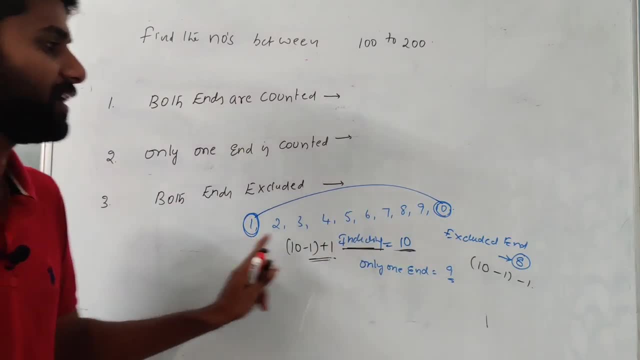 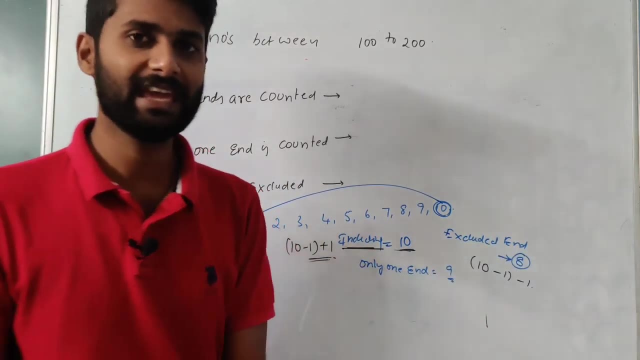 subtract a minus 1 means 10 minus 1. again we can subtract a minus 1.. Why? Because while we counting a numbers, we including both the one. but here my question: we need to excluding the ends. If same thing, if only one end is included, means simply final value minus initial value. that is the 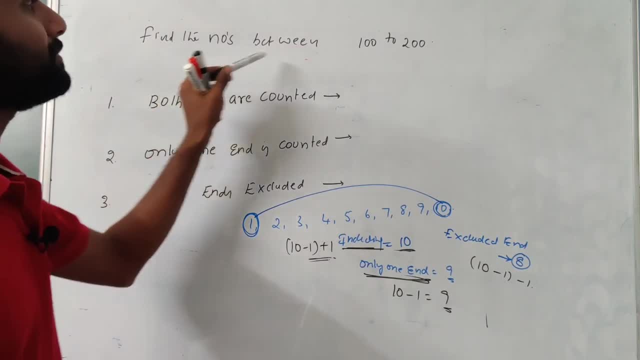 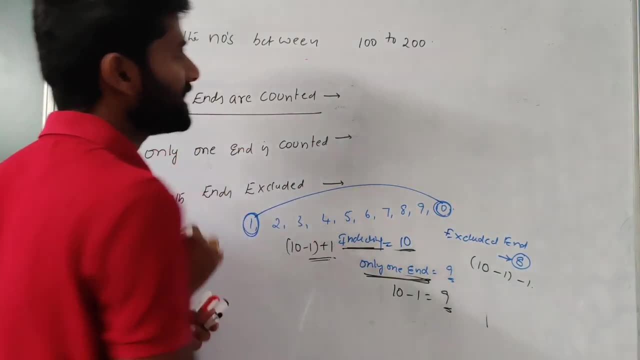 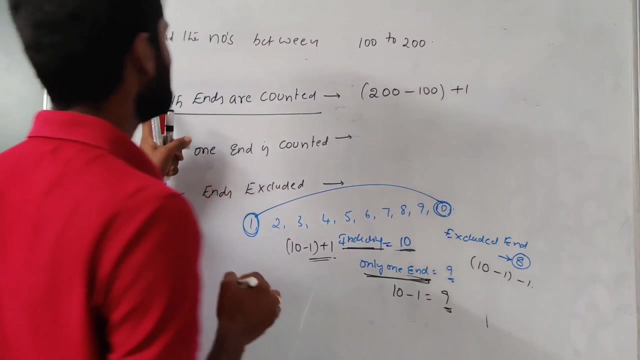 result In the same way if find the numbers between 100 to 200. if any number is given, we need to find how many numbers are there. Here my question: if you consider both the ends, if you consider both the end, means 200 minus 100- we need to add plus 1. Why? Because we are addition both the ends. if 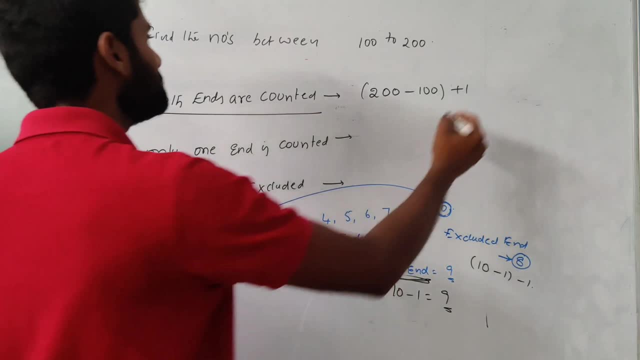 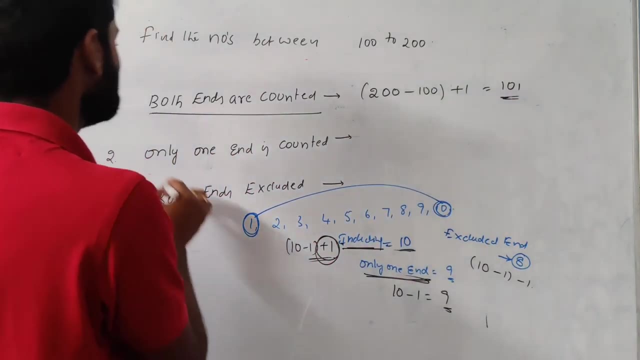 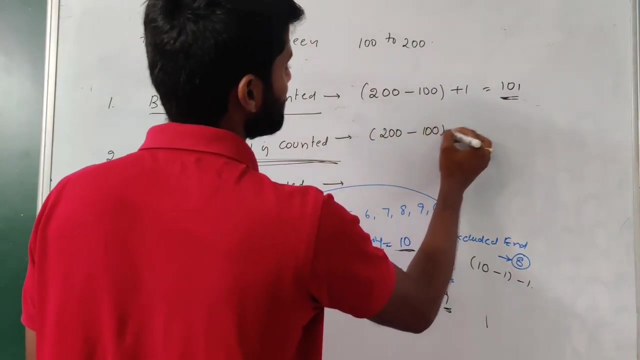 you including both the ends, we are added a number. The total then resultant is equal to 101, means 100 to 200. the total numbers are 101.. He said that if you including both the ends, if you including only one end, if you including only one end, means simply the final value minus initial value, the 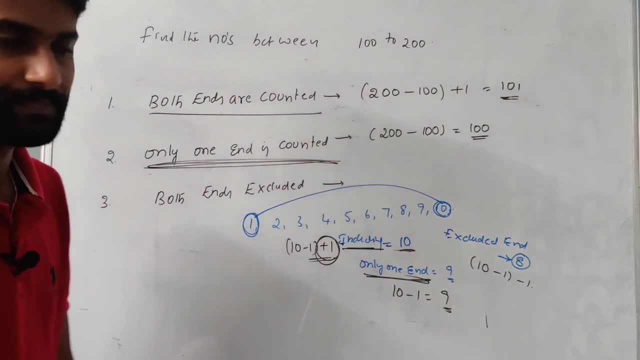 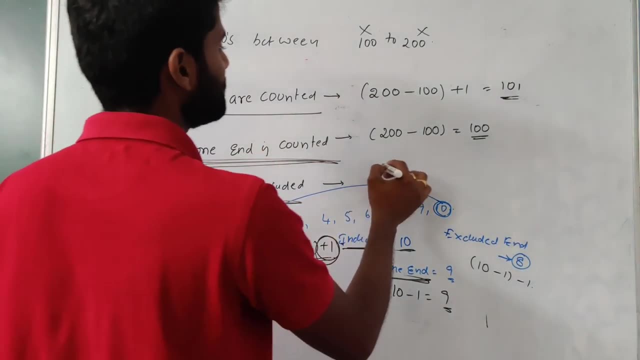 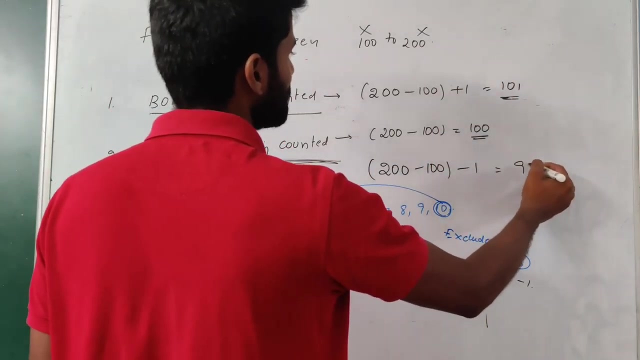 total resultant is equal to 100. only. If he said that if you are excluding both the numbers means we are excluding 100 and 200, if you, excluding both the numbers, simply subtracted 200 minus 100, again you can subtracted minus 1 the total resultant, the total numbers between 100 to 200, excluding both the 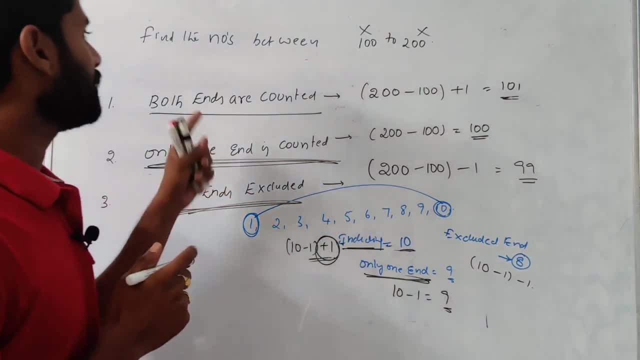 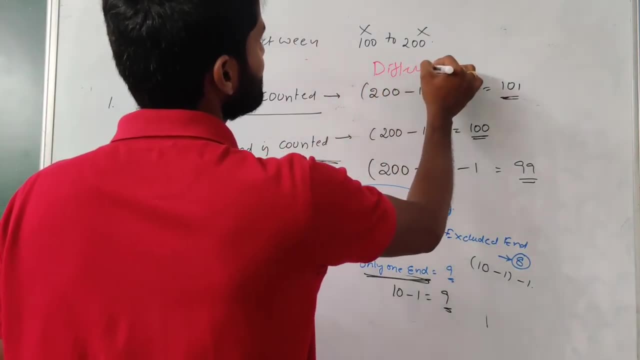 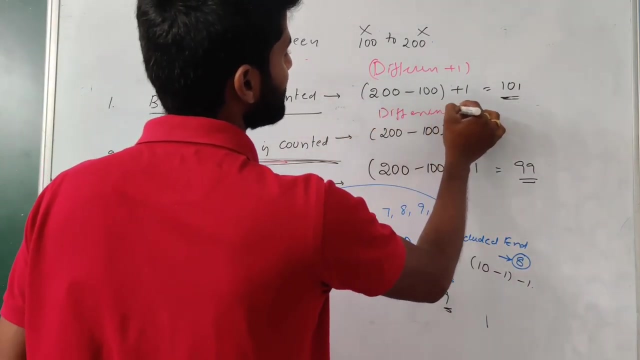 ends is equal to 99.. See if you want to including both. the end means difference plus 1.. See if you want including both. the ends means difference plus 1. that is the answer. If the question related for only one end is included, your answer is related to difference between the number. If you cannot, 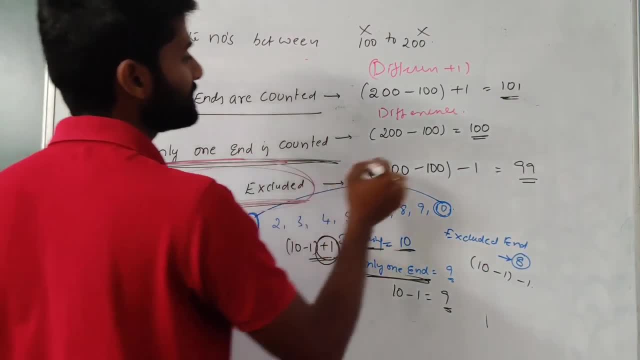 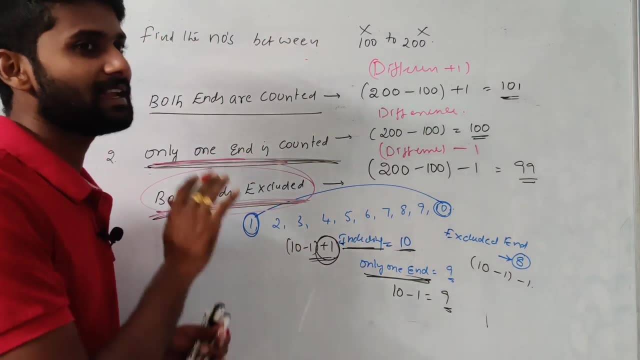 consider both the ends. if you are excluding both, the end means your answer related to difference between the numbers, again minus 1.. So this is the theory. if you counting a numbers between the any digits, between the any numbers is given, we are counting. this is the approach. 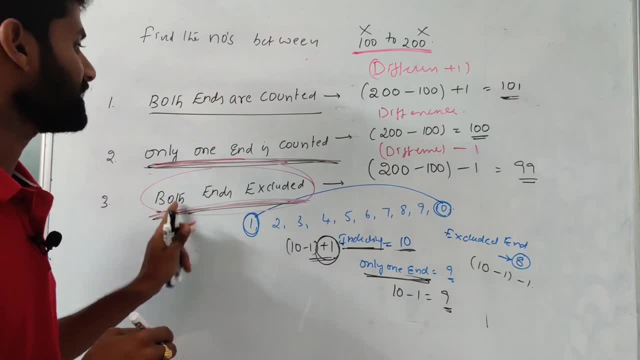 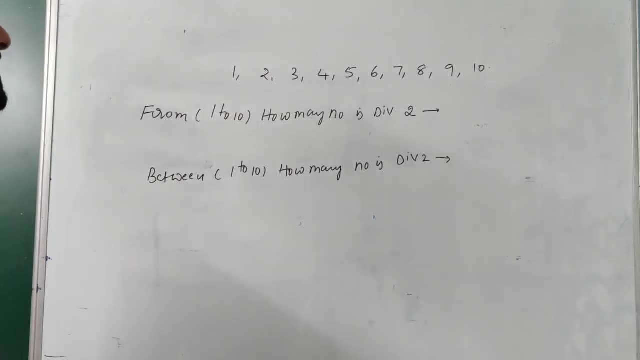 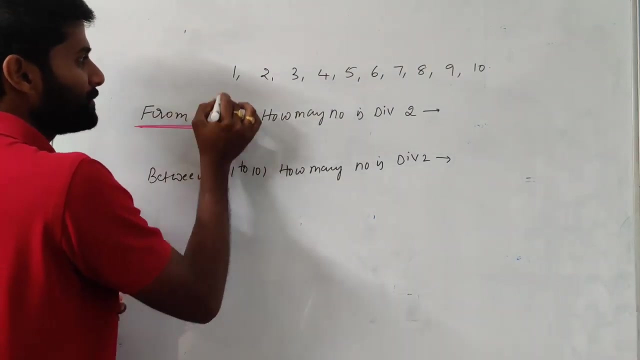 So concentrated if you both ends are included or both ends are excluded, or only one end is a included, So concentrated on the questions. We go with the divisible calculation. these are the 10 numbers here. my question: from 1 to 100.. See if the question related from 1 to 100 means. 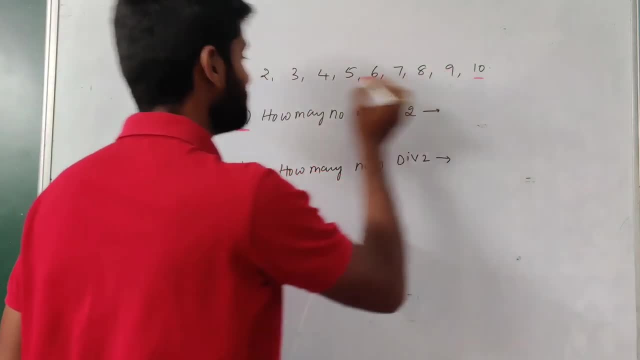 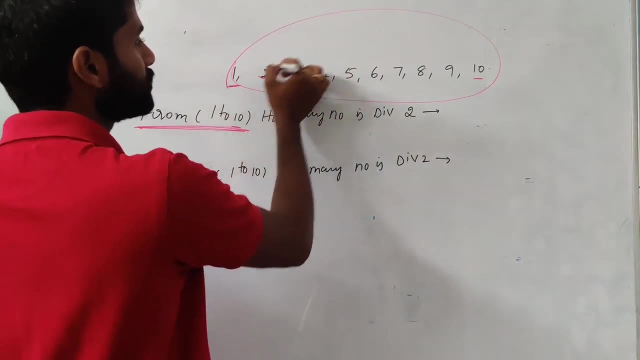 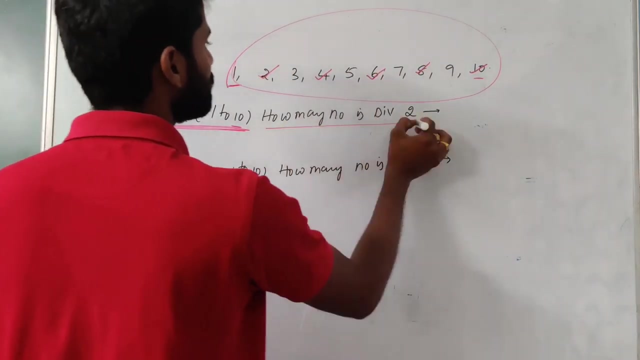 we consider First number. between last number you can consider the entire 10 numbers. that is the meaning of round. So out of these 10 numbers, how many numbers are divisible by 2.. So 2 is a divisible, 4 is a divisible, 6 is a divisible, 8 is divisible and 10 is divisible. The total number of 2 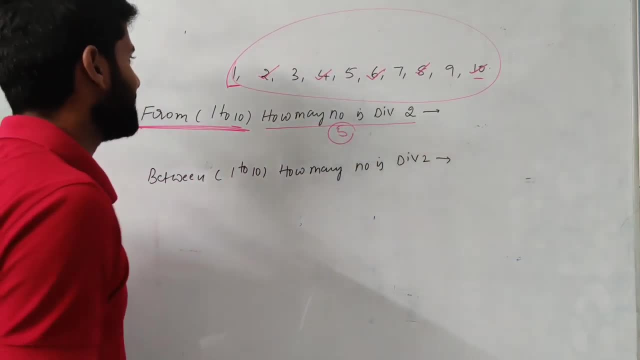 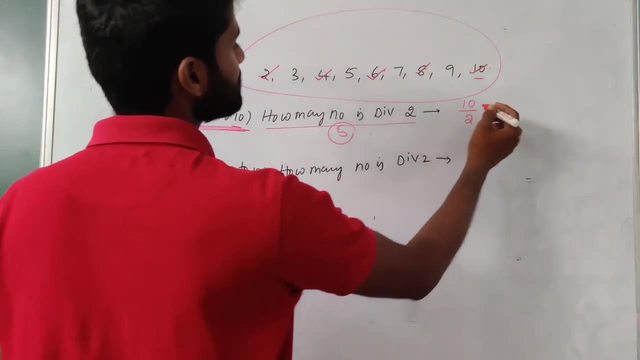 divisible numbers are 5.. If we want to go with a direct one means focus on the last number, the last number which is divisible by 2.. If last number which is divisible by 2, 10 divisible by 2, the total numbers are: 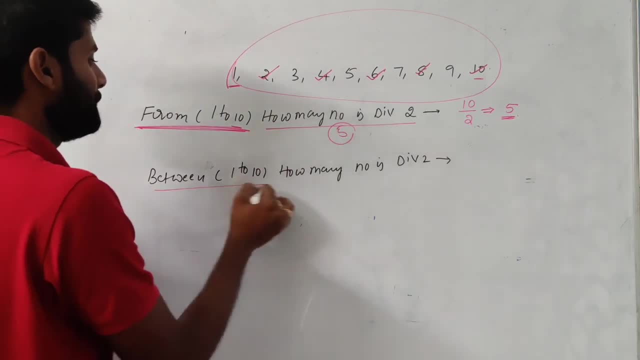 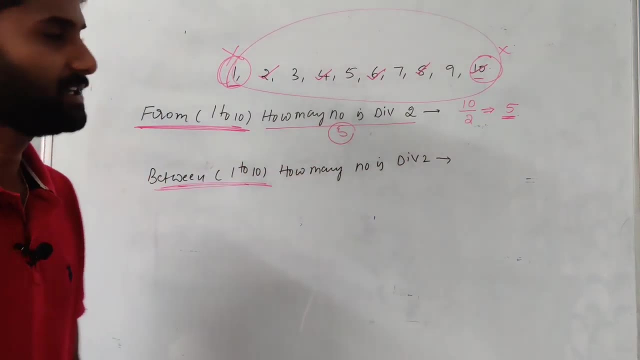 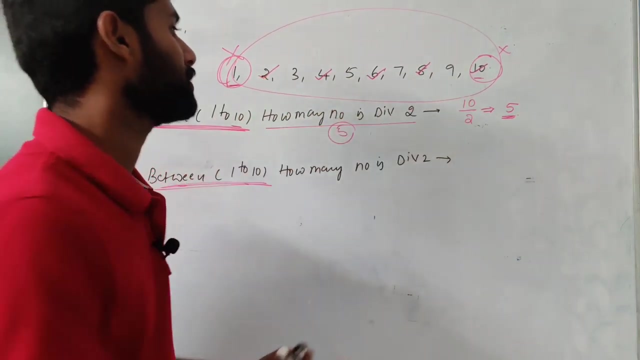 5, only 5 only Here. same question: between 1 to 10. between 1 to 10 means we need to eliminated first number and the last number. See, if you just eliminated first number and last number, we can got the remaining one. If you counted as a remaining means 2, 4, 6, 8, the total numbers are 4 only If you want to go. 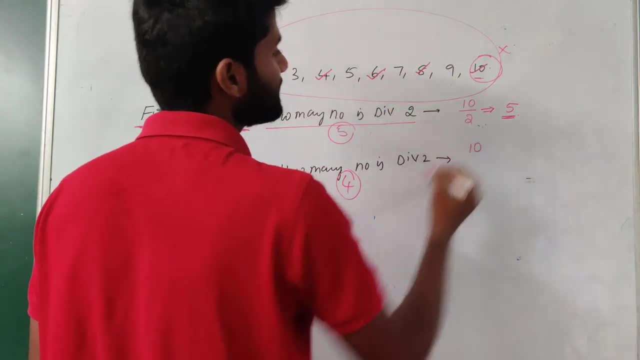 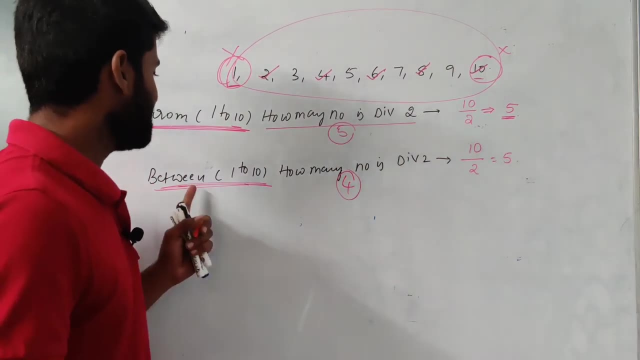 with this direct one, focus on the last number. the last number is equal to 10, and 10 is divisible by 2, we get the value of 5, but 5 is not an answer. why? Why? Because he said that we need to count it from 1 to 10.. So, between numbers, we require: 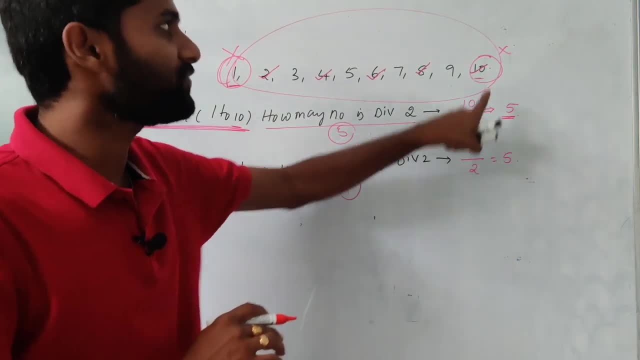 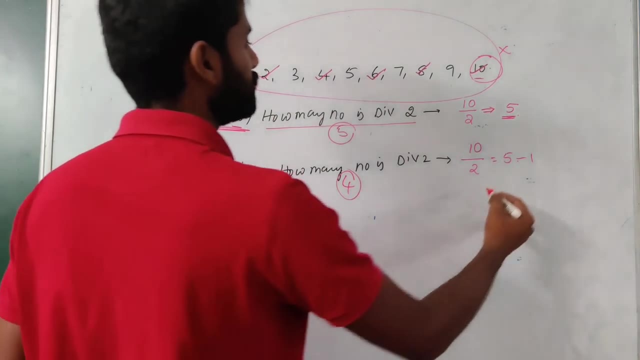 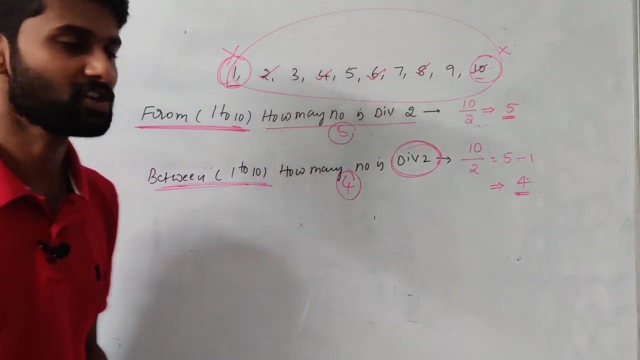 First focus on 10.. If 10 is divisible by 2 means we can consider these counting also. That is why those counting is subtracted from 5.. So the total number of digits between 1 to 10 which is divisible by 2 is exactly equal to 4 only. So observe that if the question is related. 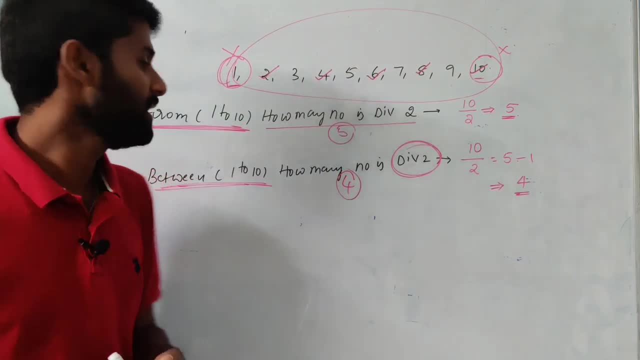 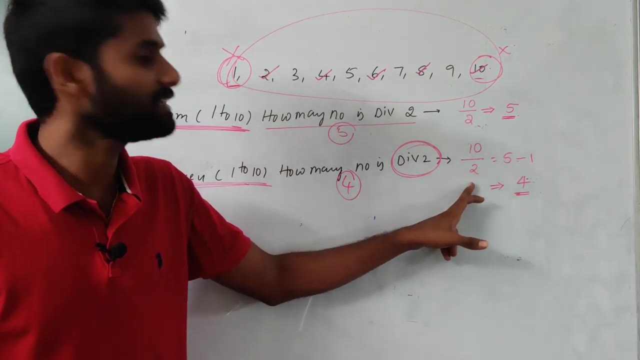 from 1 to 10 means we just including 1 and 10.. The question related: from between 1 to 10 means we just excluded 1 and 10.. If your number is exactly divisible, the given number. we need to subtracted those number. Why? Because we required between numbers only See the first question. 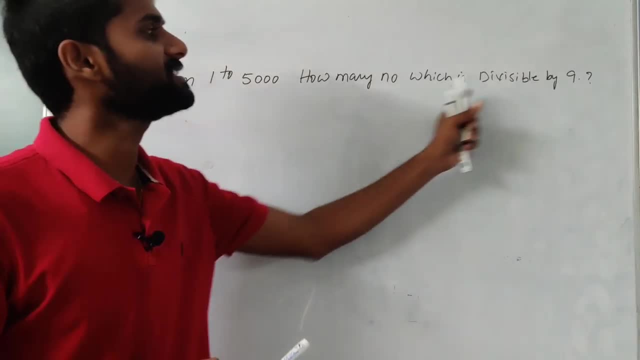 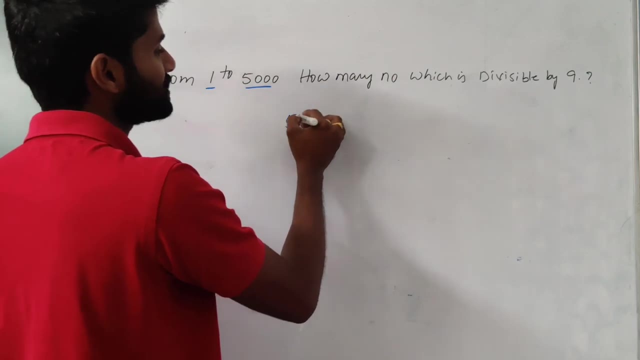 From 1 to 5000, how many numbers? which is exactly divisible by 90?. So we required from means we consider first number and last number, Simply the last, whatever the last number, which is exactly divisible by 90.. So we require from means we consider first number and last number. 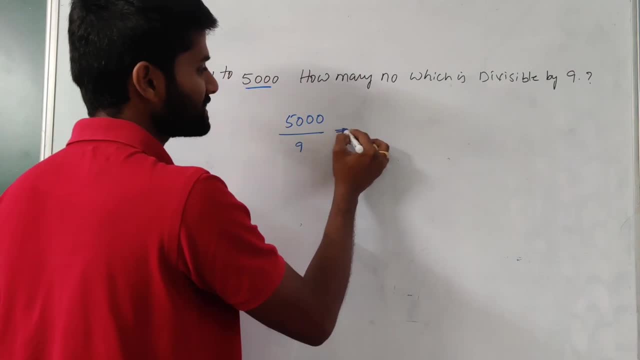 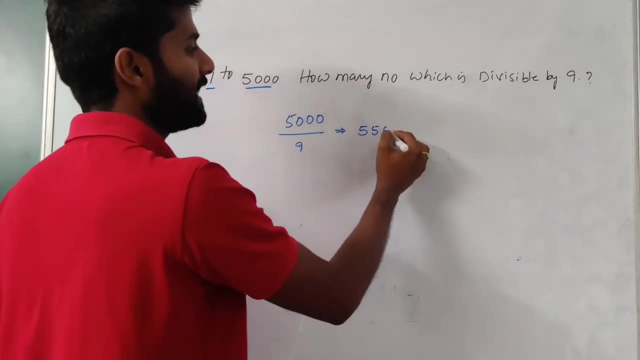 Exactly divisible by 90.. Focus on the exact cancellation. See 9 become a 10.. It is a 5 times 9. 5s are 45.. Again forward, 9, 5s are 45.. Again, 9, 5s are 45.. We have a decimal. Again, 9, 5s are 45.. 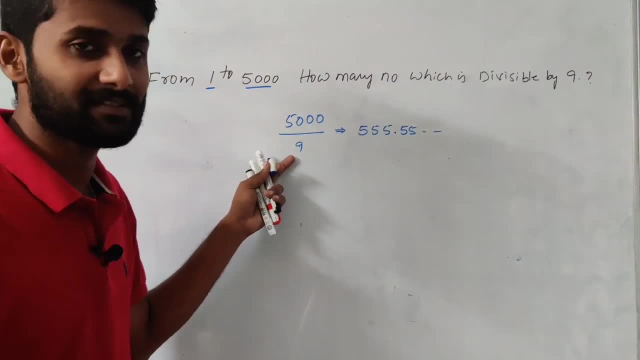 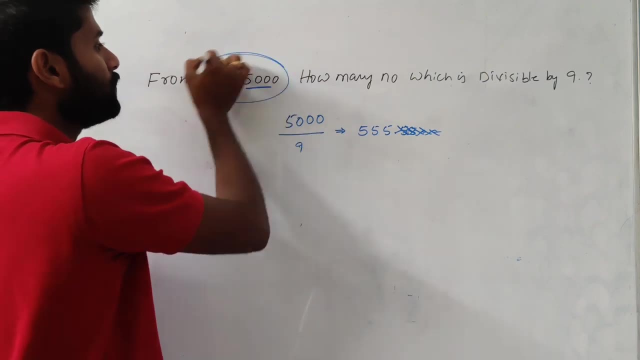 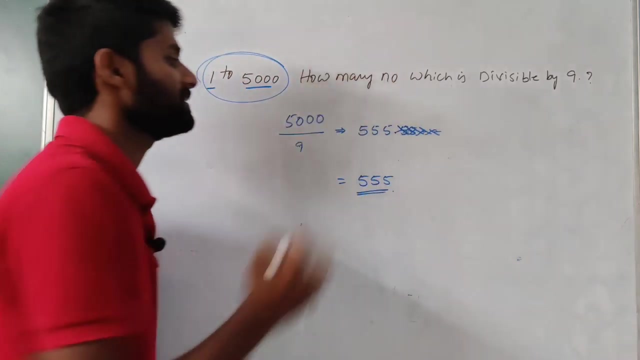 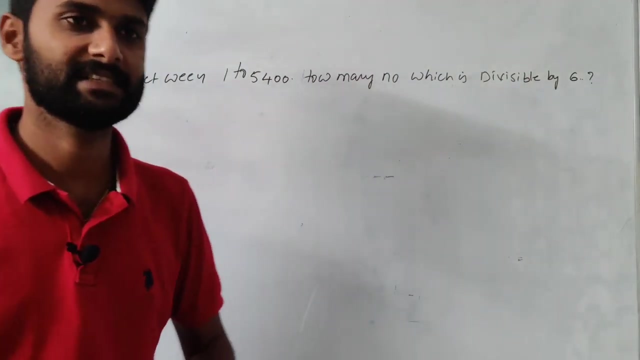 So on. means these number is not exactly divisible by 9. means simply eliminate the decimal values. It means the question if 1 to 5000, the total number of divisibles by 9 exactly equal to 555. That is your answer. Between 1 to 5400, how many numbers? which is divisible by 6? Same thing. 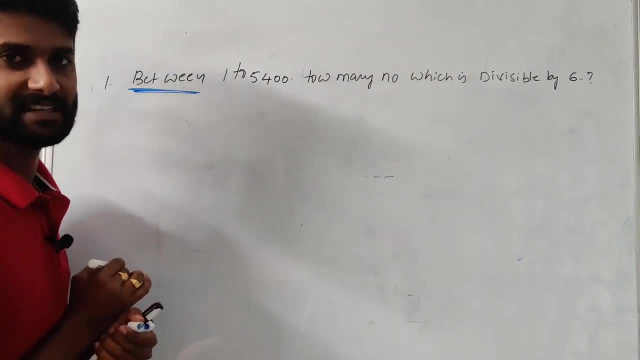 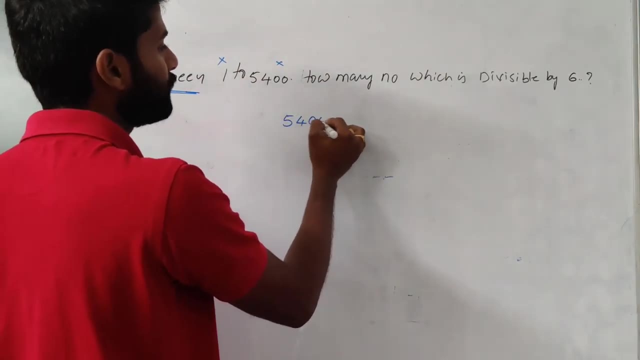 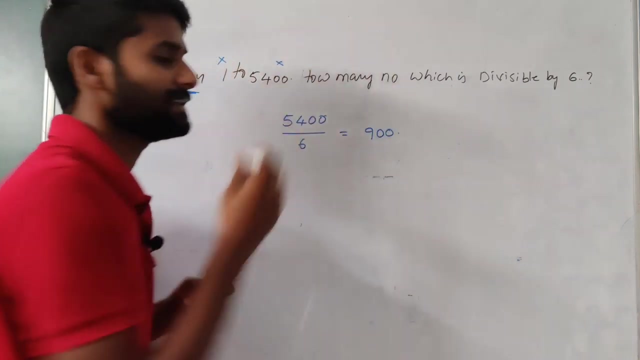 We are question concentration part. be the between Between means we need to eliminate a first number and a last number First. take it as a last number: 5400 is exactly divisible by 6. So 6 become a 54. Exactly, there are 900 numbers. So out of 900 numbers. 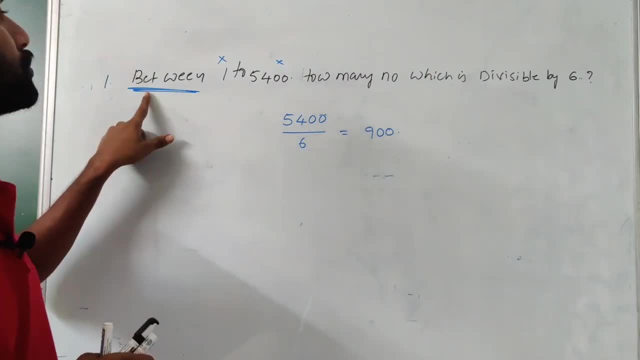 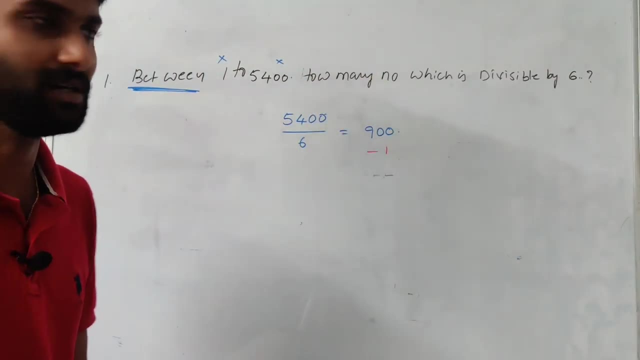 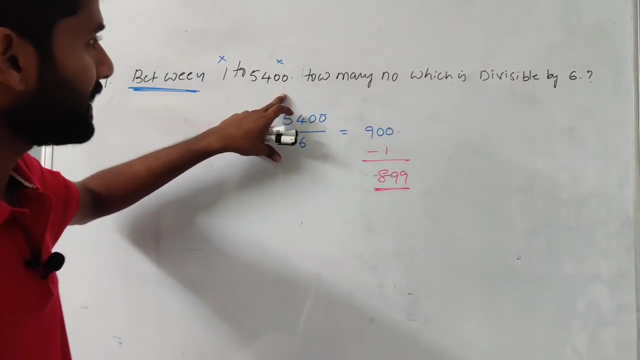 they included 5400.. But my question is related between the numbers. means we need to exclude 5400.. That is the one number. It means your calculation is related for 899.. It means between 1 to 500, the total number of divisible basis is 899.. 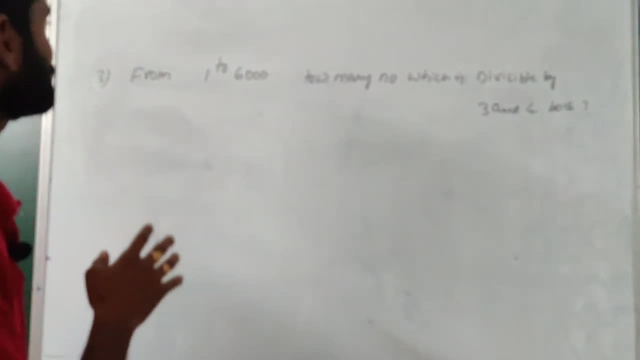 Let us see the next question: From 1 to 6000, how many numbers which is divisible by 6? 899.. 9 live numbers solve it. 7 eat numbers solve it. 8 satellite numbers solve it. Now, the answer here is: from Q1 to Q6, there is calculation of 1 to 6000.. How many numbers which is divisible by 6 is 1 haven and 99.. 5 The number of. 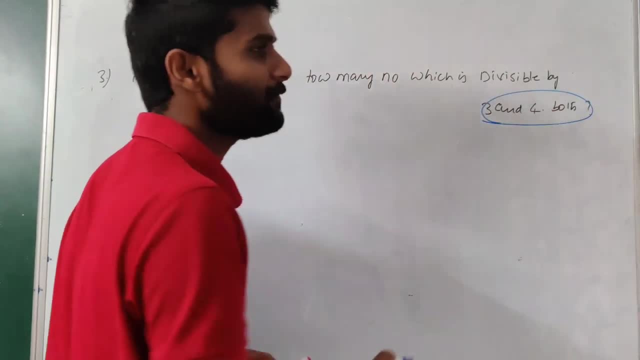 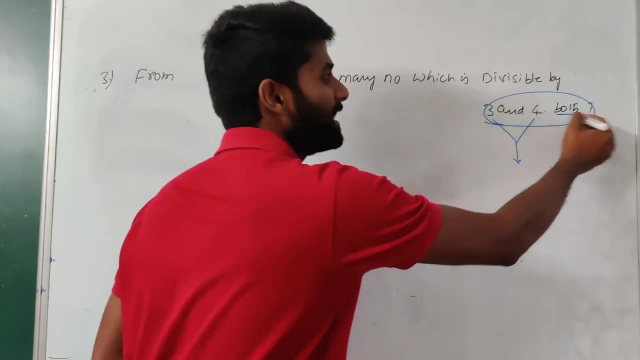 is divisible by 3 and 4. both 3 and 4. both means the common multiple of 3 and 4 is the exact divisible number. They are given as 3 and 4.. Means the LCM. Find the LCM of 3 and 4.. What is the? 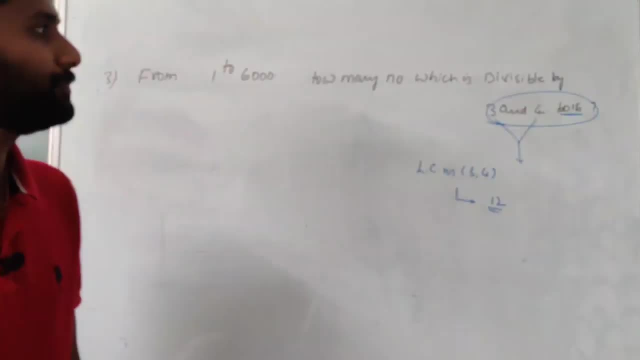 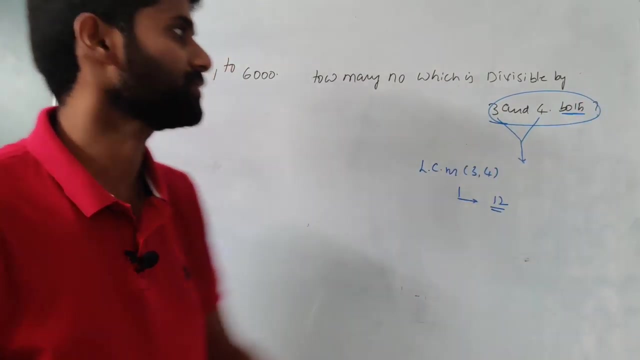 common multiple of 3 and 4? That is exactly 12.. Means how many numbers between 1 to 6000, which is exactly divisible by 12.. That is the meaning of 3 and 4, both Simply. our answer related to. 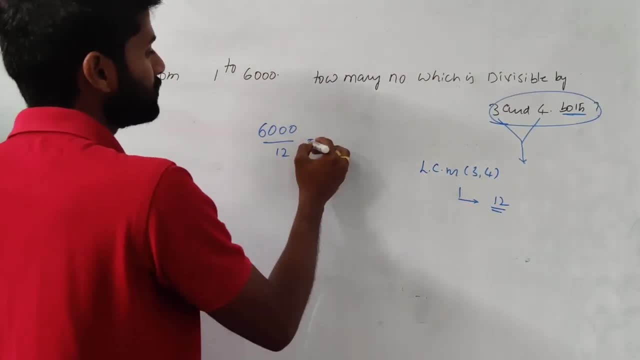 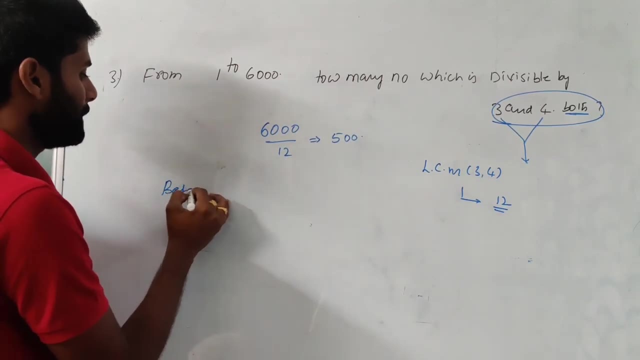 6000 divisible by 2.. If 6000 divisible by 2, the total numbers are 500. Why? Because 12 5s are 60.. If same question related for between 1 to 6000.. Between 1 to 6000 means 6000 is exactly. 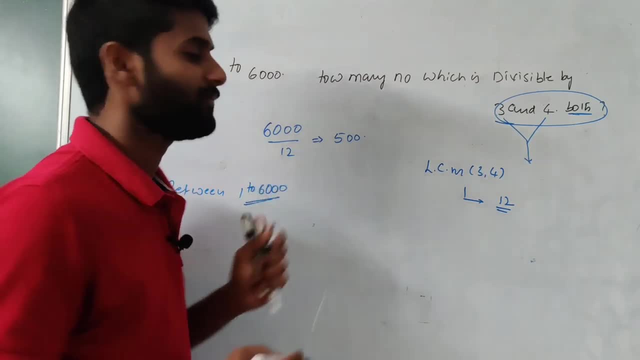 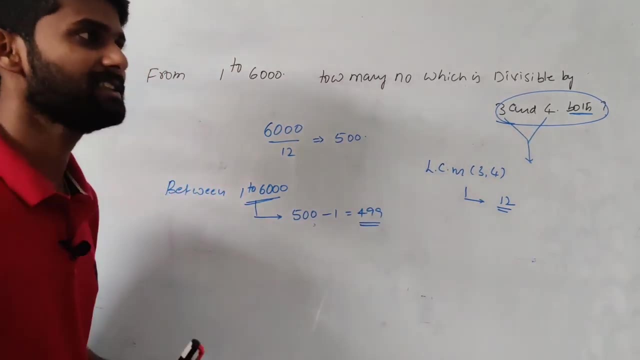 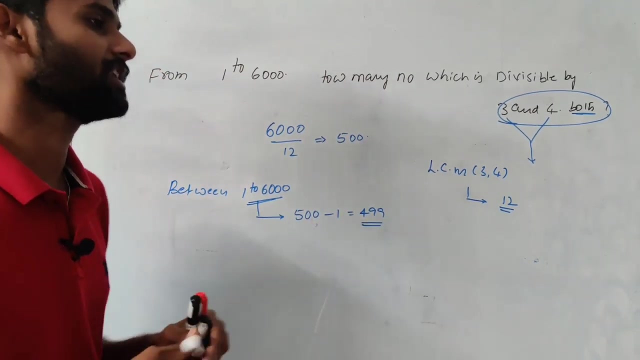 divisible by 12.. Means those number is subtracted from 500. Then your answer is related to 400 minus 1.. The answer is related to 499.. See the question. From 1 to 6000, the total numbers are 500.. Between 1 to 6000, between 1 to 6000, the total numbers which is divisible by 12 is: 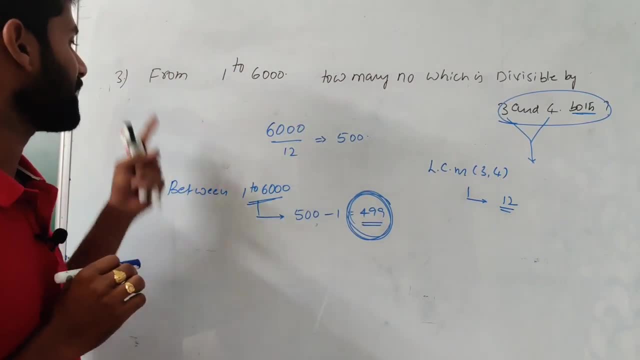 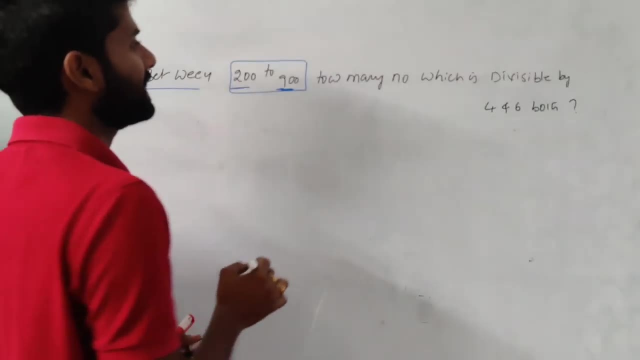 equal to 499.. So just see the question: from or between Same Between 200 to 900,. if they are given for 200 to 900, how many numbers? which is divisible by 4 and 6, both 4 and 6, both means. 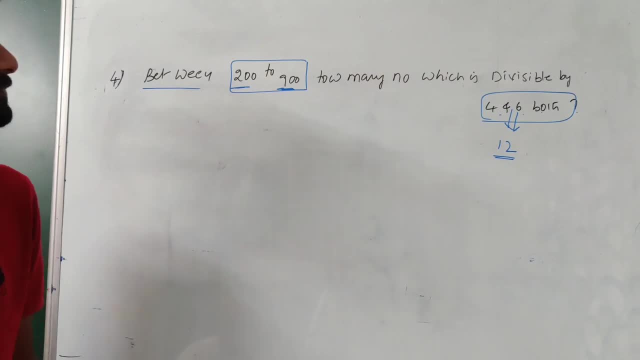 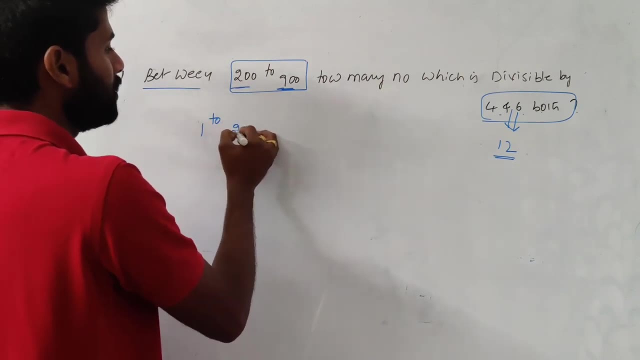 the total LCM of 4 and 6 is equal to 3.. But here the numbers are not 1 to 900, 1 to 900. First of all, concentrated, how many divisibles are there from 1 to 200. See. 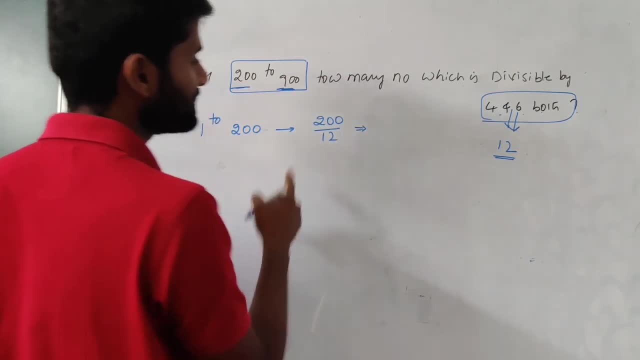 if 200 is divisible by 12, how many numbers are there? Just check it out. So 12: 1s are 12.. 8 AB the carry forward and 12: 6s are 72. The total numbers are 16.. See, 200 is not. 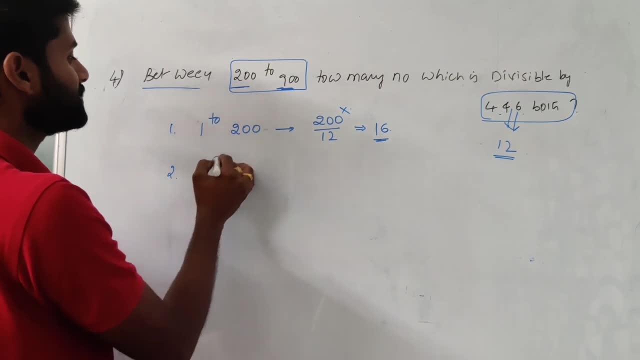 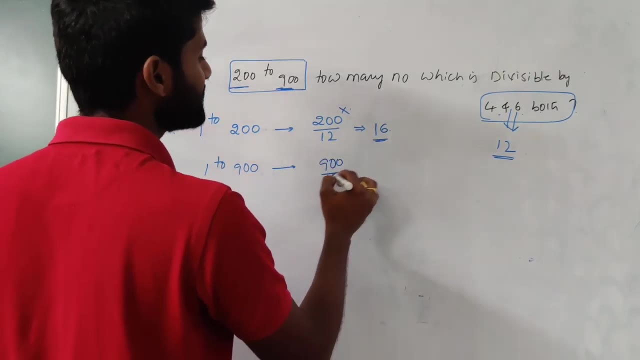 a divisible number And second one- So just check it out- How many numbers are between 1 to 900?? So 1 to 900 means If 900 is exactly divisible by 12. So 900 is exactly divisible by 12.. How many are there? 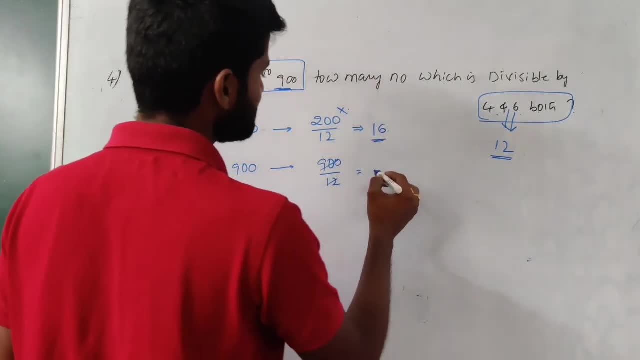 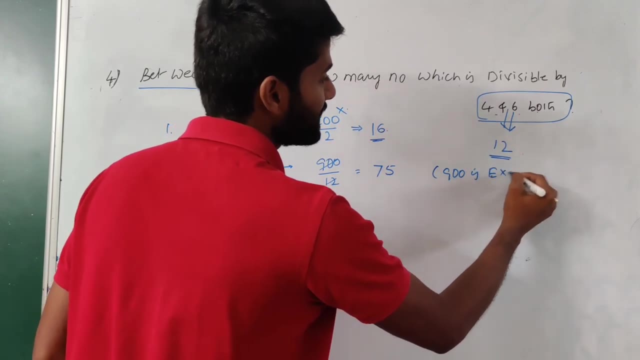 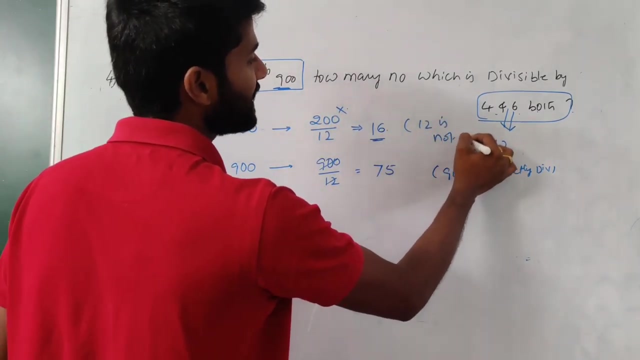 Just check it out. So 12 become 12, 7s are 84. So 12: 5s are 60. It means 900 is exactly divisible. So that is the important point we need to note here. And 12 is not exactly. 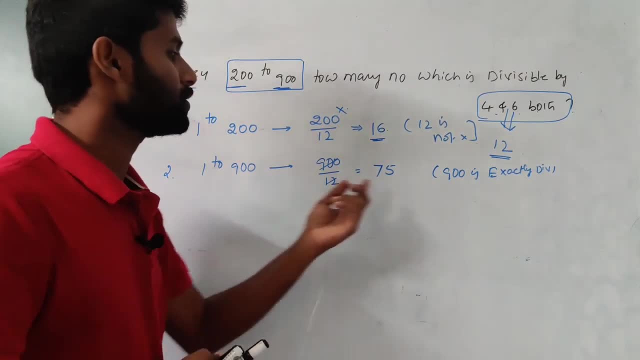 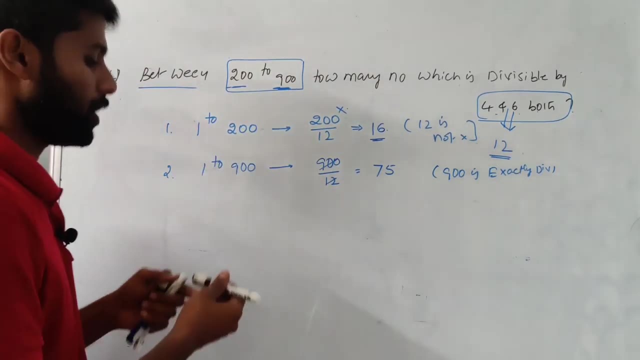 divisible From 1 to 900, the total numbers are 75.. From 1 to 900, the total numbers are 60.. From 1 to 900, we have 60 numbers. My question: between 200 to 900, how many numbers? 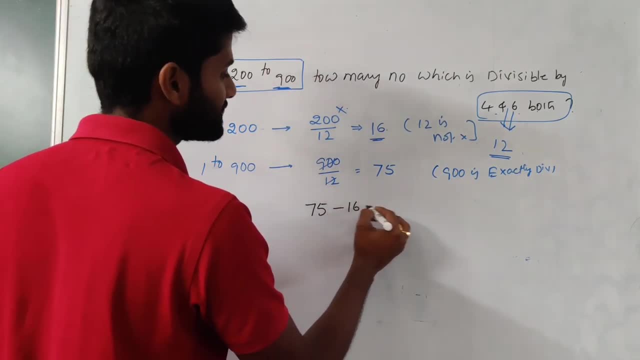 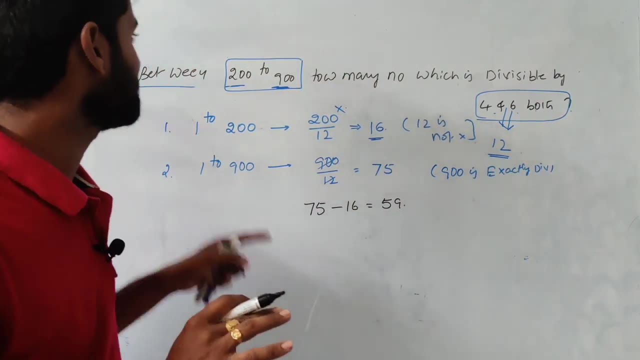 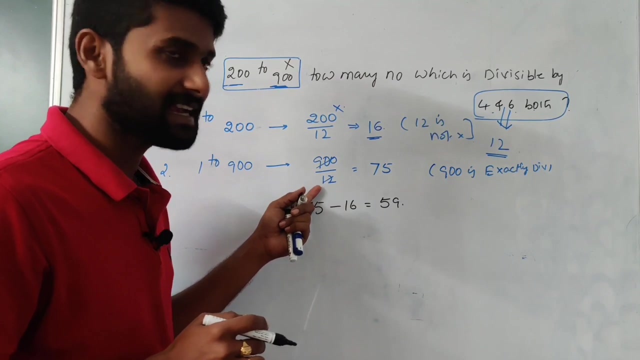 are there Means 75 minus 16.. The total numbers are 59. But you can just 59 as answer. But remember that we required between means we need to excluding exact 900 divisible number. Why? Because 900 is exactly divisible by 12, means we need to subtract those number also. This is the important point. So that is why you have to answer to the exact 900 divisible number. So that is why you have to subtract those number also. So that is why you have to answer to the exact 900 divisible number. So that is why you have to answer to the exact. 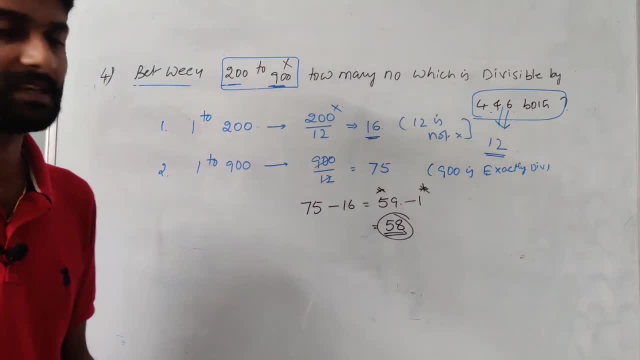 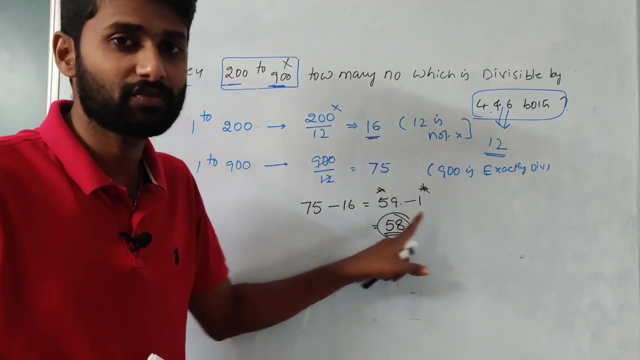 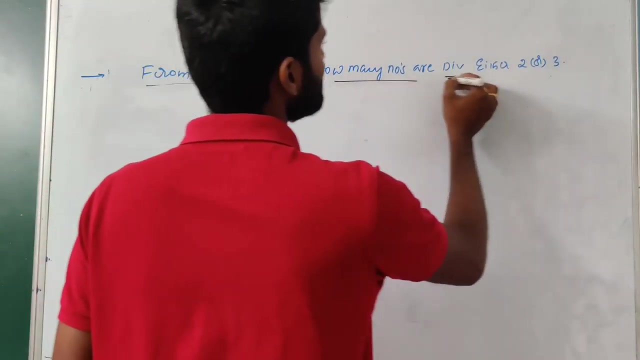 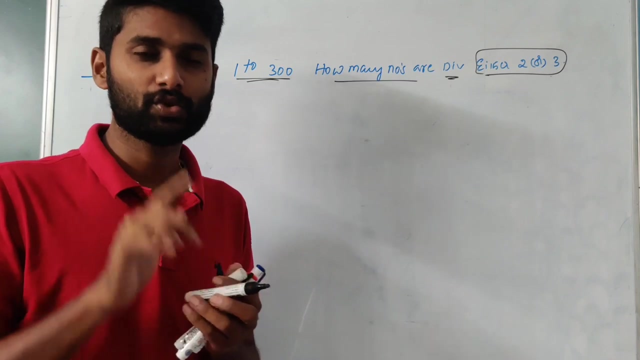 number also See. there are 9 of these reactions for this particular situation. They can distance to familiar of the two results, So that is why you need to extract one of those numbers and see. Thank you for watching the video. This video is being reproduced on diesesvinaryorg. 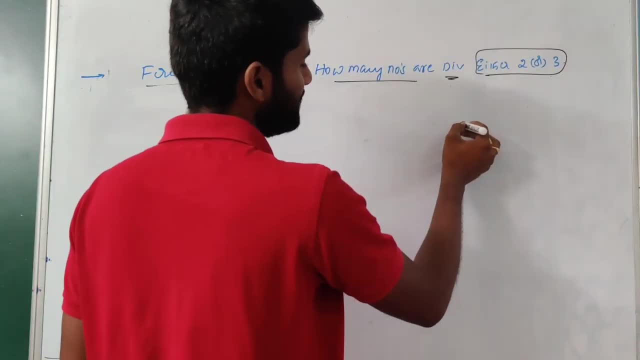 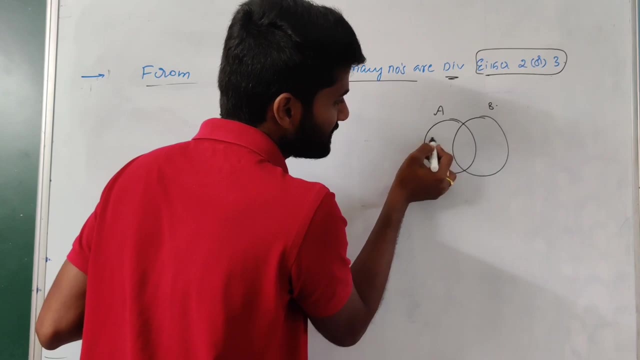 So that is the meaning of aetheron. If you go with a Venn diagram, see they deals with the one circle, that is, a, and they deals with the other circle, b. So this particular space is defined with only a section, means this section is not intersected with b and this section is intersected. 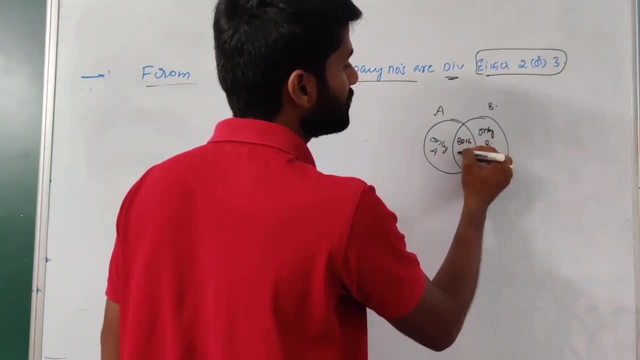 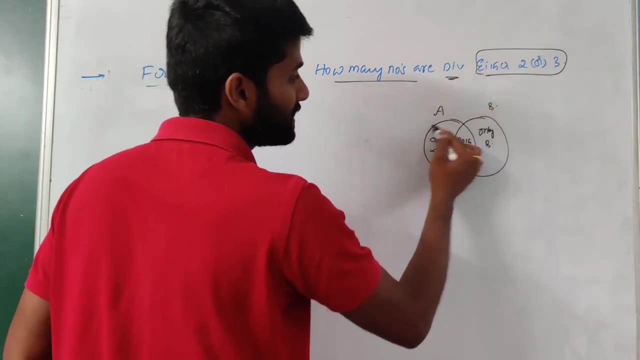 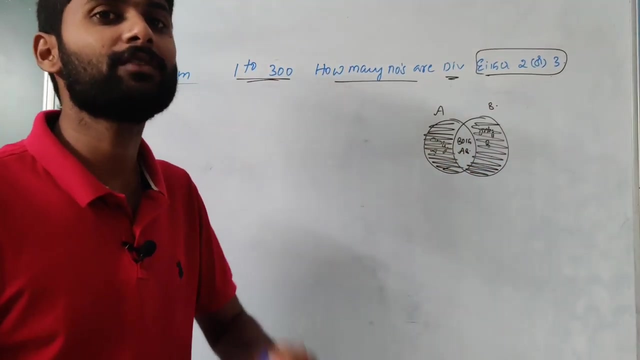 with only b, and this is the combination of both a and b. Previous question: they are discussing for both a and b. For this question we can choose, as either 2 or 3 means you can choose either these case or these case only, But out of these two cases, we cannot confirm a particular case. 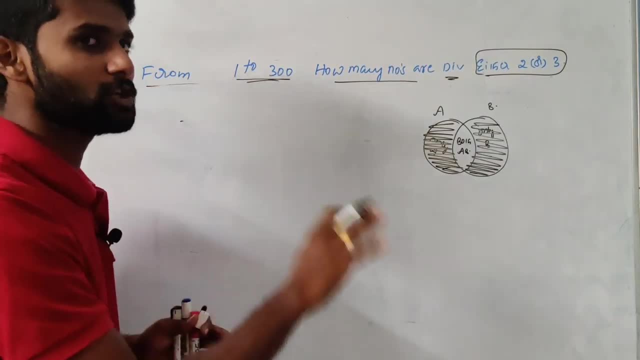 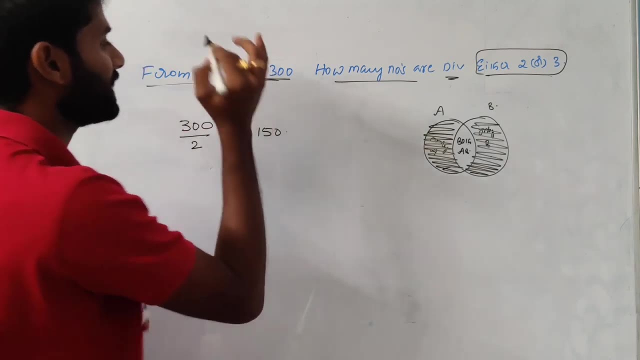 That is why focus on from 1 to 300 means we just including numbers from 1 to all 300 numbers. So 300 is divisible by 2, we get the total numbers are 150.. If maybe that is divisible by 3 means 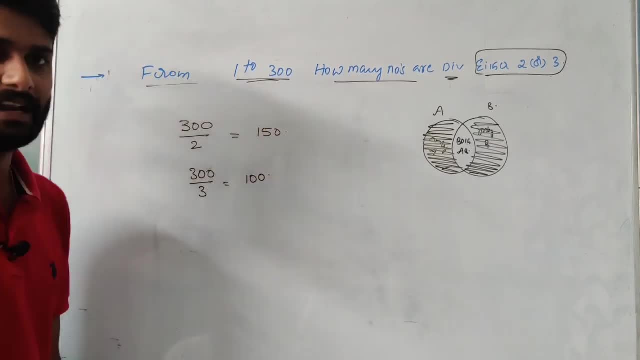 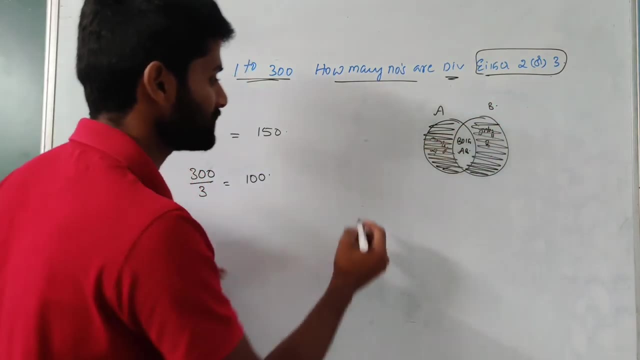 300 divisible by 3, the total numbers we left is 100.. But these 350 numbers and these 100 numbers, it is a combination. It is a combination of both 2 and 3.. Why? Because, for example, 1, 2,, 3,, 4,, 5, 6,, 7, 8, for example. 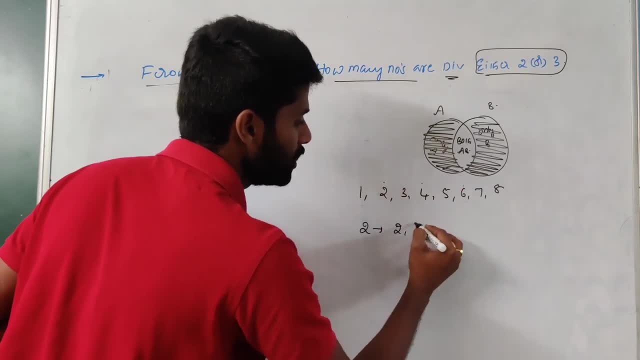 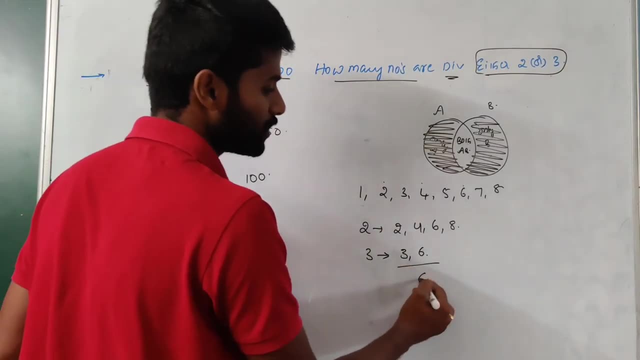 So how many 2 divisibles are there? 1, 2, 3.. So those are 2, 4,, 6, 8.. If same question, how many 3 divisibles are there? 3, 6. The total numbers we can conclude as 6.. But this is the wrong answer. 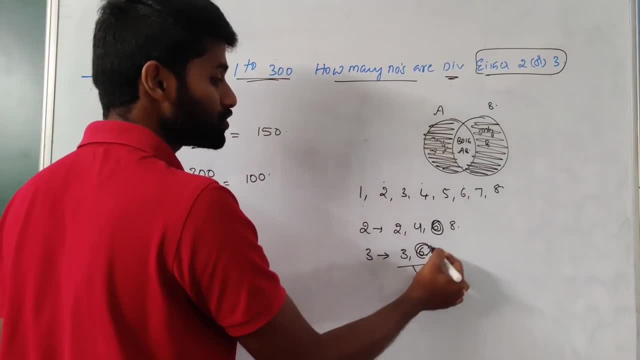 Why? Because 6 can be counted as 2 times. Those 2 times we can subtract at one time only. That is why the 300 which is divisible by 3.. So that is the combination of both 2 and 3.. So that is the. 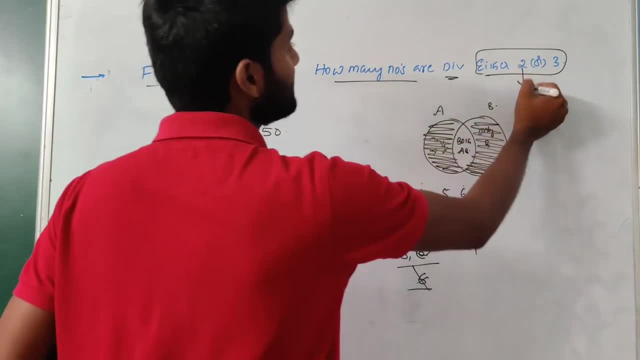 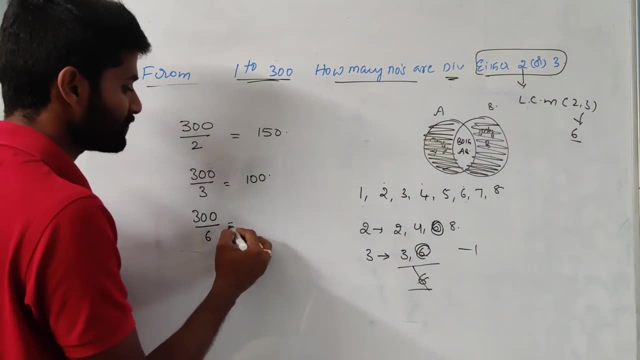 reason why the 300, which is divisible by 6, focus on 6. also Why? Because the LCM of 2 and 3 is exactly equal to 6. only Clear, If 300 divisible by 6, we have a common multiple, 50 common multiples. 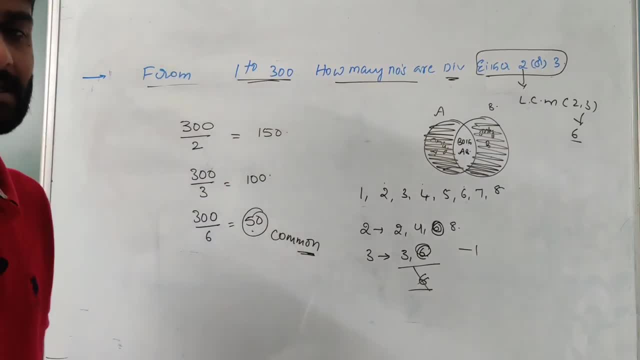 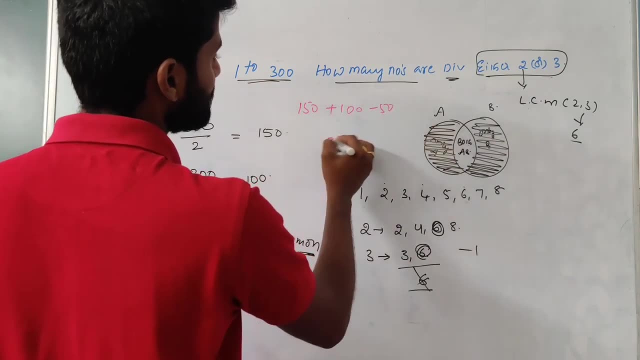 of 2 and 3. Those 50 we can subtract from these numbers, Then the final resultant of this question: 150 plus 100 minus 50. The total numbers are 200 numbers. The 200 numbers which is divisible by 6. 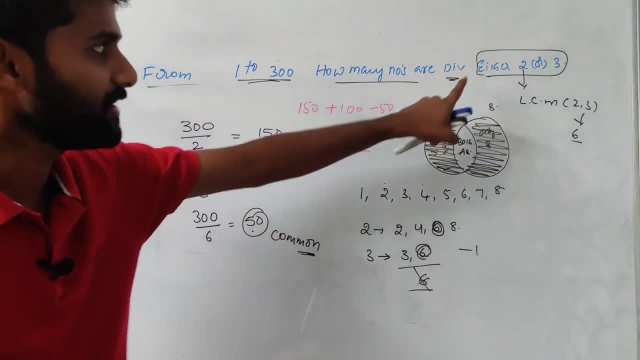 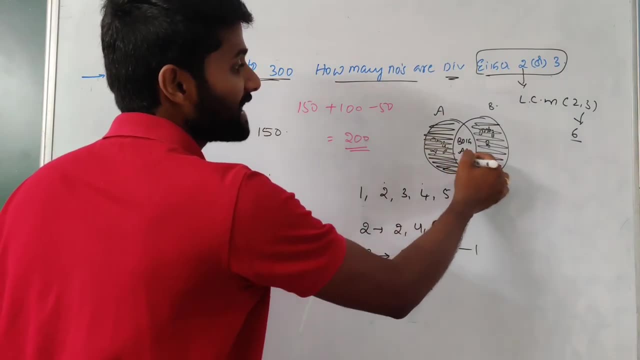 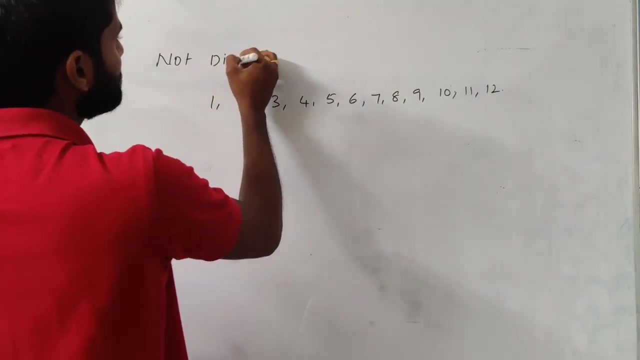 are divisible by either 2 or 3.. So see, if the question is related for either 2 either or case means we can consider only one case and we can subtract a common case. that is the important part. If the questions are related to not divisible cases, how many numbers are not divisible by? 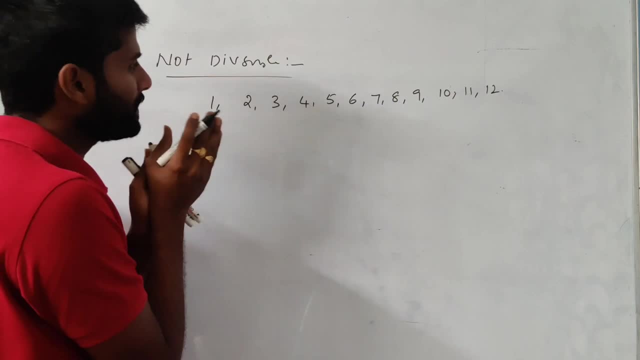 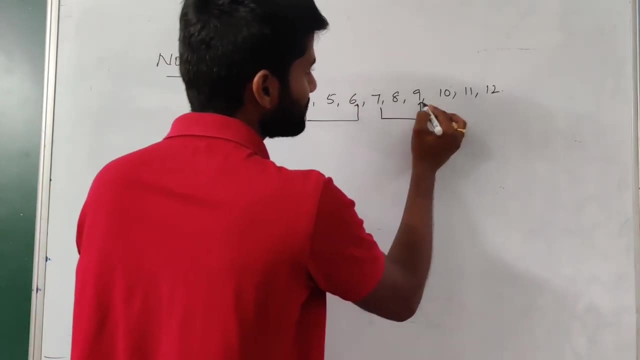 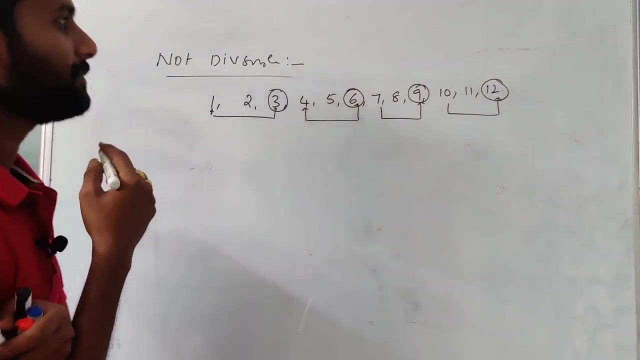 number. See, if you consider as these numbers, If you go with the, how many 3 multiples are there? means the 3 multiple we get every 3 numbers C, So get every 3 numbers, we get a 3 multiple. means 3 multiples are 3, 6, 9 and a 12.. Here my question. 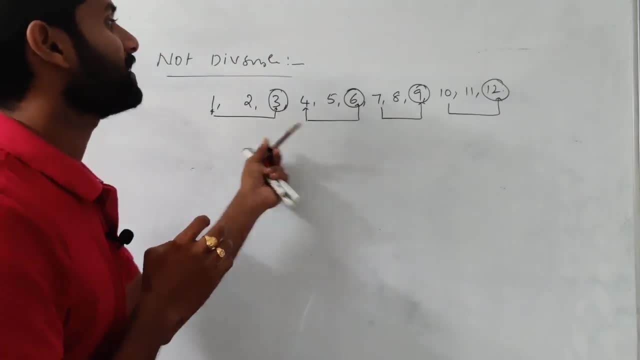 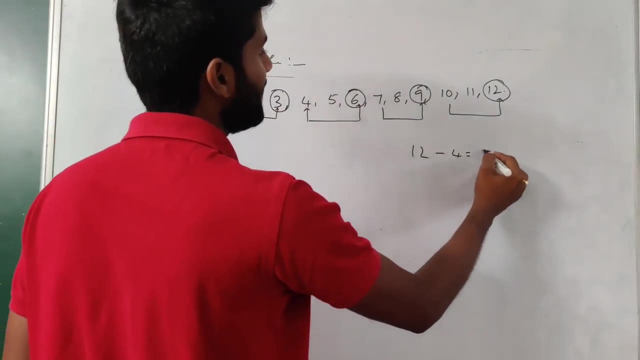 out of 1 to 12. how many 3 divisibles are there? So we have a 4 divisibles. How many numbers which is not divisible by 3 means the total number 12 minus 4, 8 numbers is not divisible by 3.. 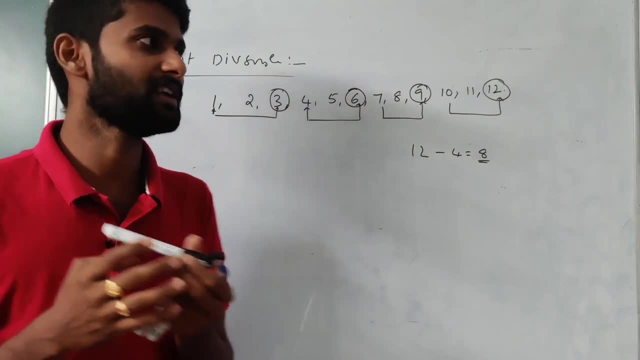 If it is a larger number, not divisible case be the difficult why? because not divisible can indicated total minus 4.. So if we take that method, which is just for given a formula, So so it is not divisible. So M is divisible by 1.. So number not divisible is divided by 3 and 3.. So so that is a number which is not divisible, then its something that total minus 3.. So by this we can give a serious number, because not divisible, for the total number 12 minus 4 is solved to a very written problem, So so. 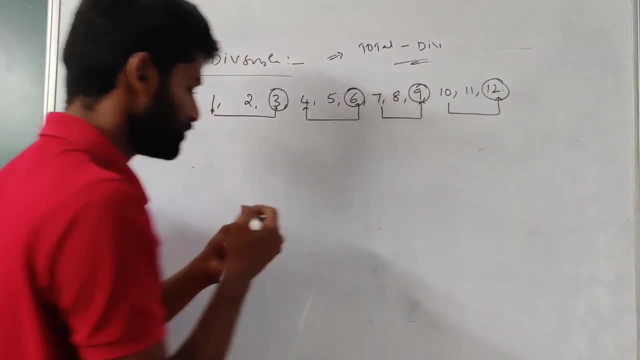 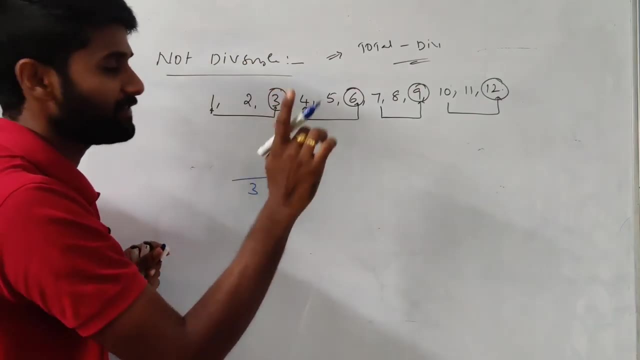 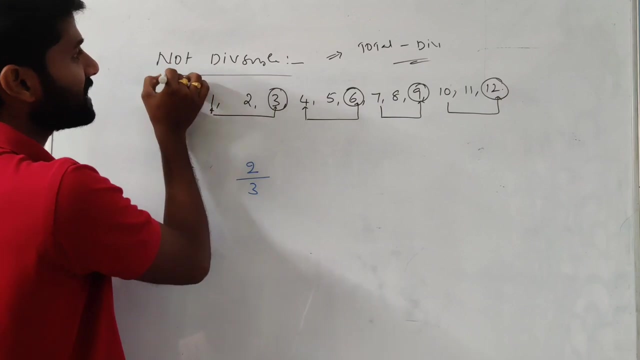 divisible. So we just focus on the other concept. see here: see, out of three numbers we have a three numbers. out of three numbers, we have a one divisible means, out of three numbers we do not have two divisibles. That is why, if the question is related for not divisible by three means, we 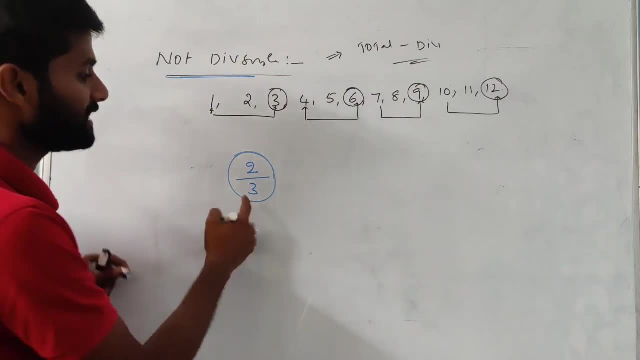 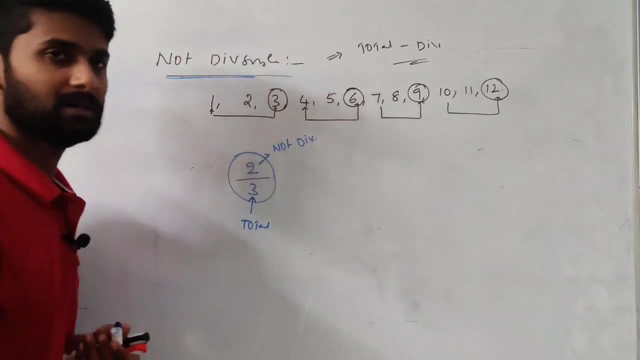 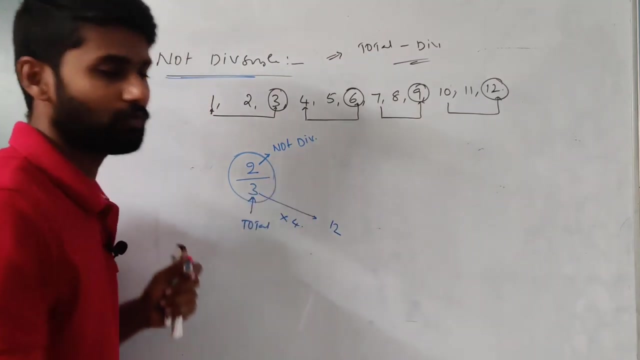 can consider, the fraction is equal to 2 by 3.. Here denominator can indicate a total value and numerator is indicated, not divisible number. It means- see I will give the example from all these numbers- if 3 divisible by 12, the total number is belongs to the 4 and same thing: 2. 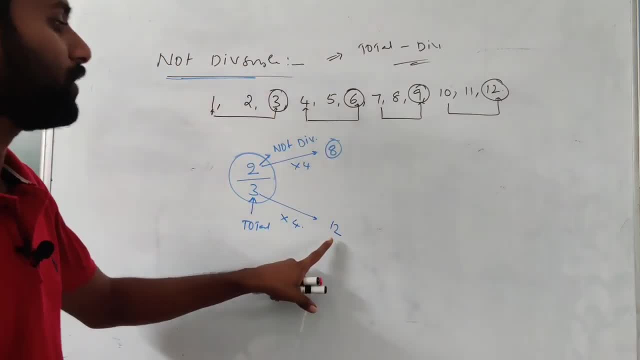 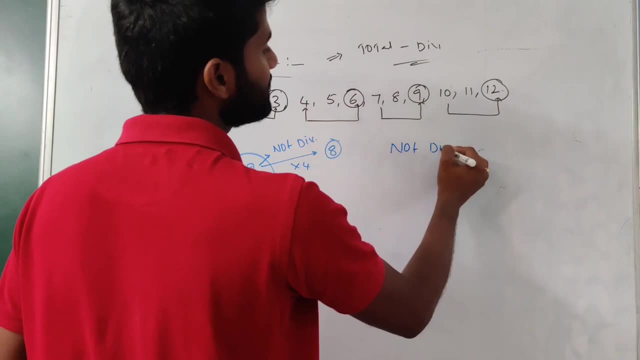 into 4, the total value become 8. means, out of 12 numbers, 8 numbers are not divisible by 3.. If same concept, if not divisible by 7, how many numbers are there in not divisible by 7.. See, every 7 number is not divisible by 7.. So we can consider: the fraction is equal to 2 by 3.. 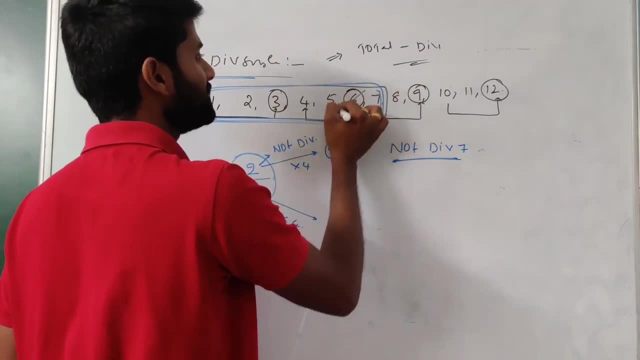 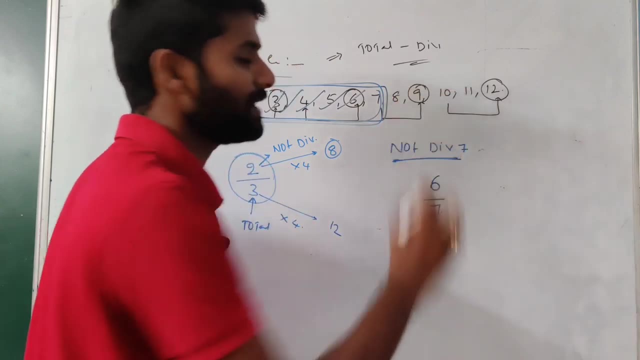 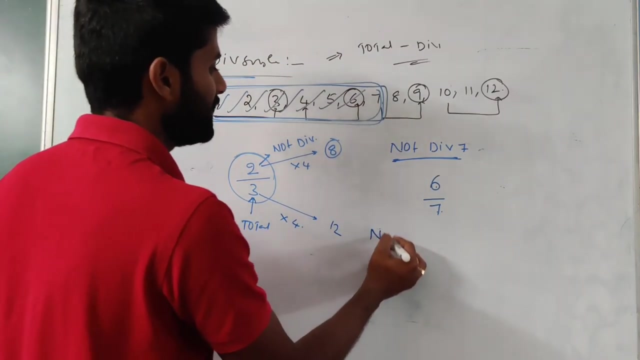 If you have concentrated on every 7 numbers, every 7 numbers, 6 numbers are not divisible by 7.. It means the fraction is a representation of 6 by 7, means, out of all the numbers, 6 numbers are not divisible by 7.. If same concept, if not divisible by 5, if you consider as a 5 numbers out of 5, 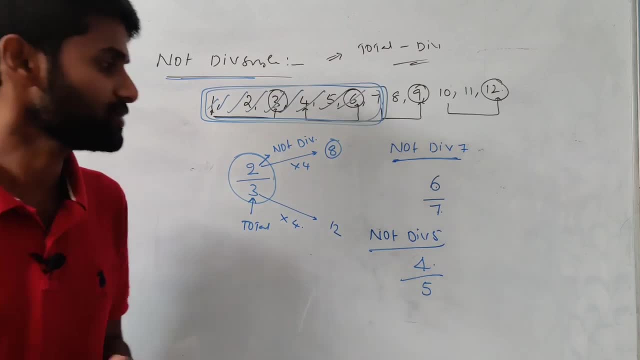 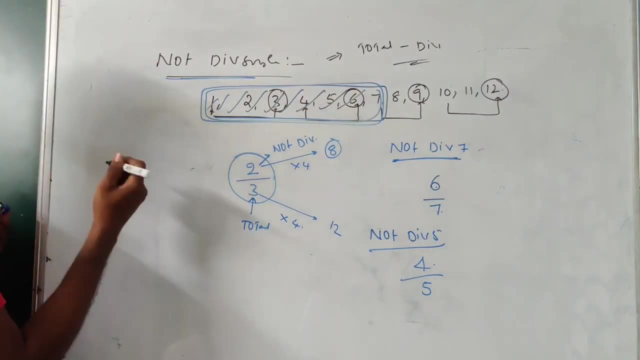 numbers, 4 numbers are not divisible by 5.. So you can consider these type of fractions, Ok, If you go. the same question from 1 to 12: how many numbers are not divisible by not divisible by 2 and 3? this is your question. See, out of 2, 1 number is not divisible. If you want to, 3, not divisible. 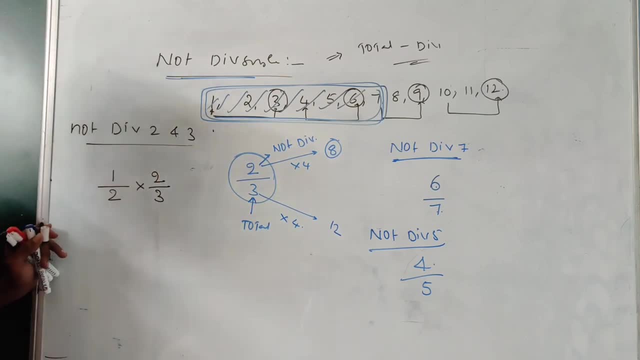 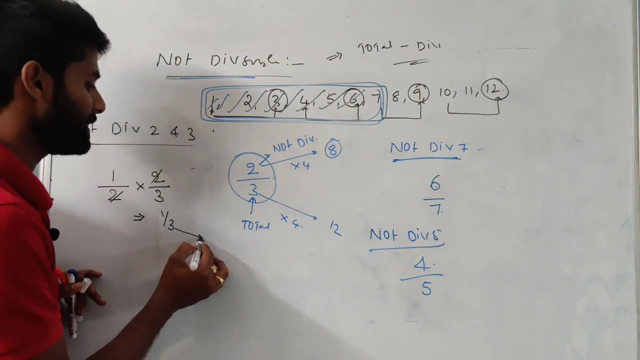 means we have a 3 numbers out of 3. 2 numbers are not divisible. Then 2: 2 cancel. we left the fraction is equal to 1 by 3. Then 3 can be represented total value. So 12 is exactly. 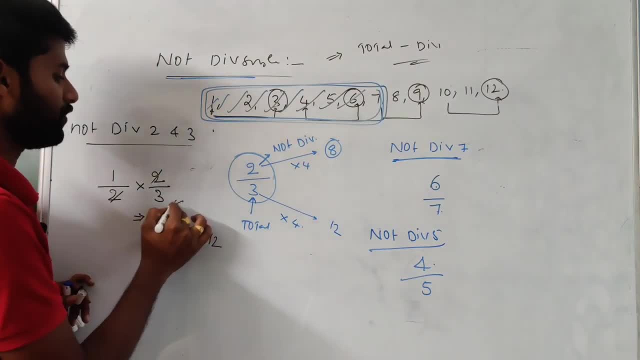 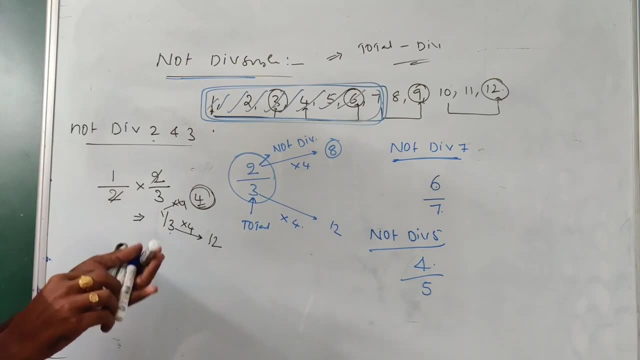 cancel means 3 become a 12.. 4 times again 1 into 4, exactly equal to 4.. From 1 to 12, 4 numbers are not divisible by 2 or 3, just concentrated 2 and 3 divisible means this is divisible. This 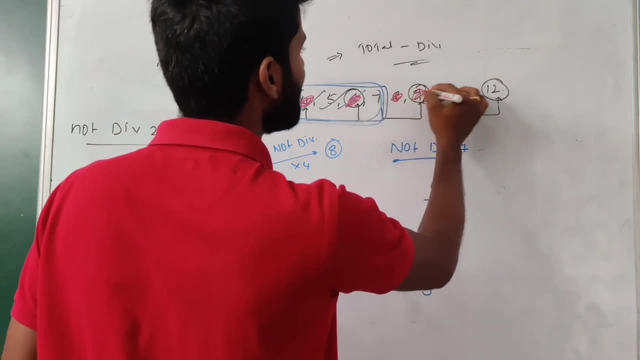 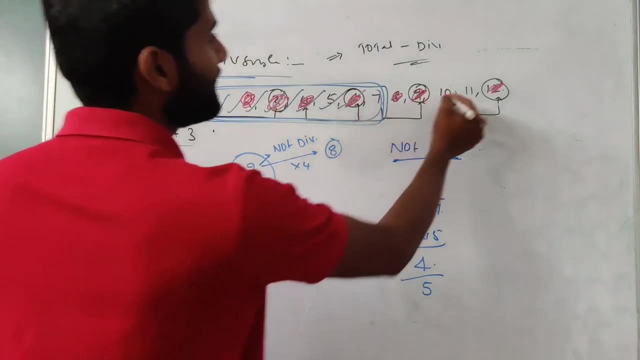 is divisible, divisible, 6 divisible, 8 divisible, 9 divisible, 12 divisible, and, and 2 and 3.. So 2 and 3 and 10 is also divisible and counted final numbers, we have a 1 number, 5,, 7.. Now 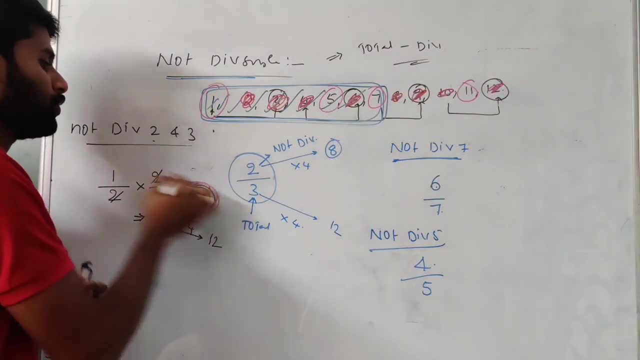 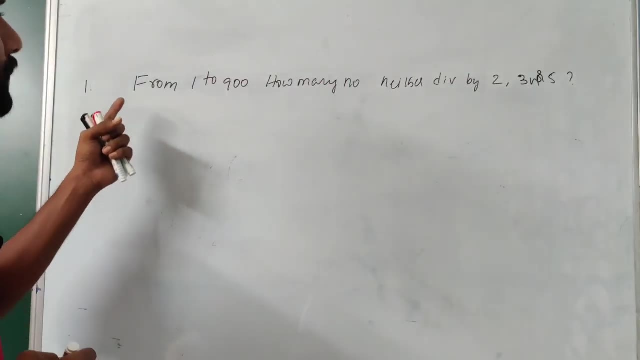 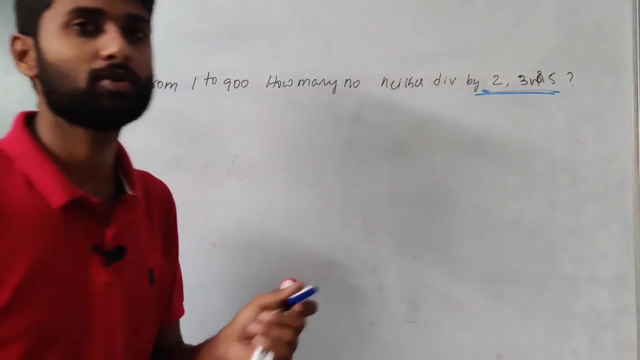 and 11. total, we have a 4 numbers. This is the not divisible concept, clear. So application, just check with application, See from 1 to 900, how many numbers are neither divisible by 2,, 3, 5.. We need to consider how many numbers are not at all divisible by 2,, 3, 5.. I will tell you the 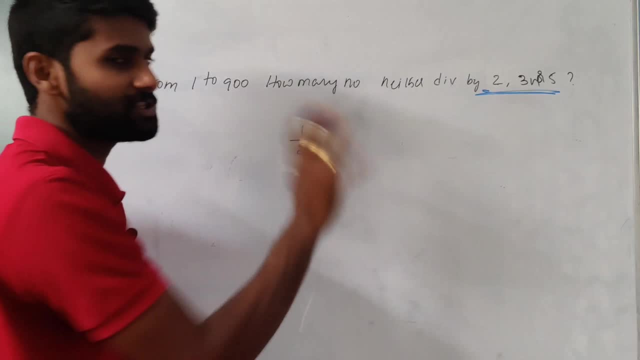 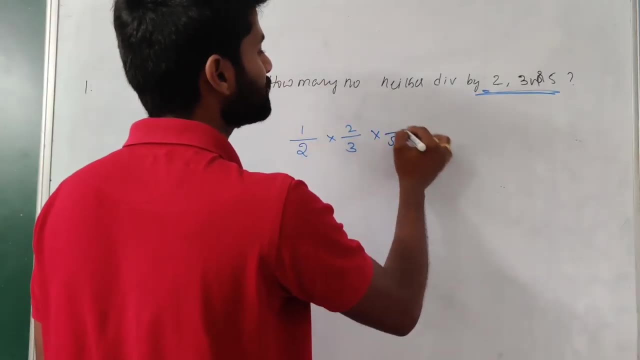 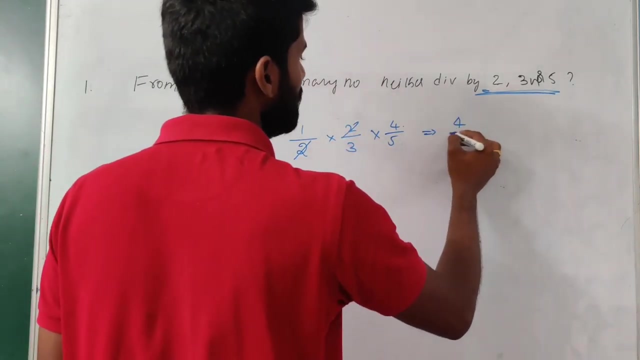 concept: Out of every 2 number we have, 1 number is not divisible. If you want, 3 means out of 3 numbers, 2 numbers are not divisible. Out of 5 numbers, 4 numbers are not divisible. Then check with the calculation Here: 2 to cancel the final calculation. be the 4 by 5, 3's are 15.. See if you. 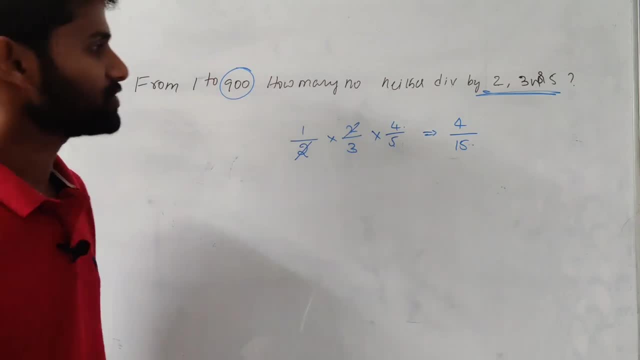 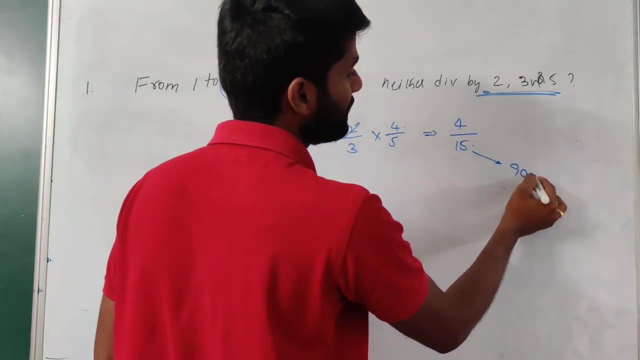 from 1 to 900 means you consider 900 also. So 900 is exactly cancellation on 900. sorry, 15 is exactly cancellation on 900.. See if 5 become a 900, if 5 become a 900, check how many times it is. 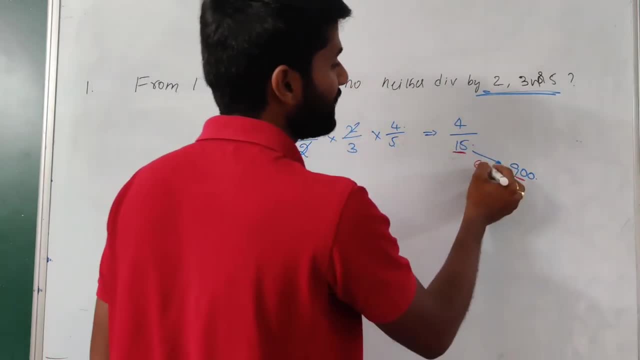 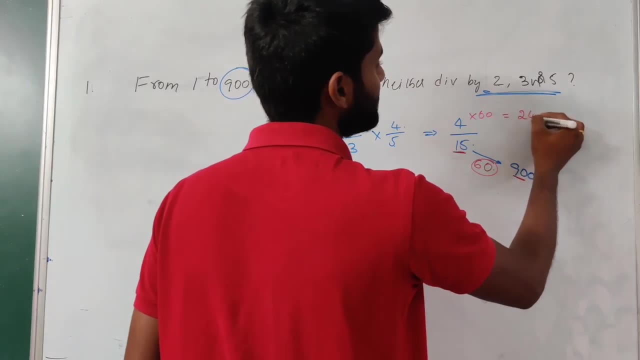 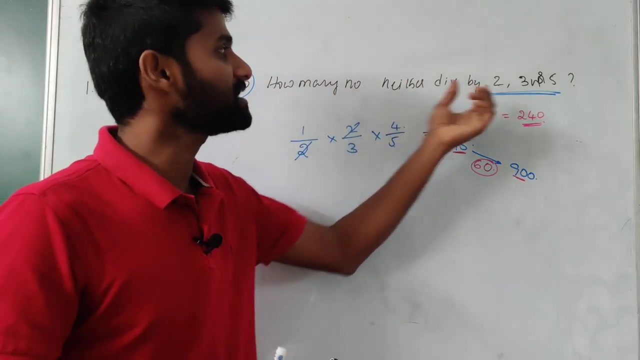 So 15 become 6, 15, 6 are 90 and we have a 60 times. If 15 become a 900, that is 60 times 4 into 60, the total number is equal to 240. clear. So from 1 to 900, the number numbers, which is not. 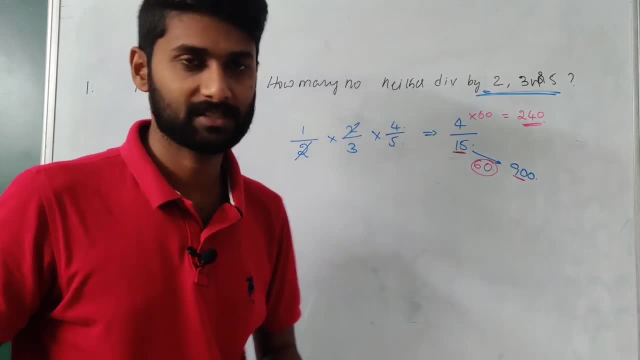 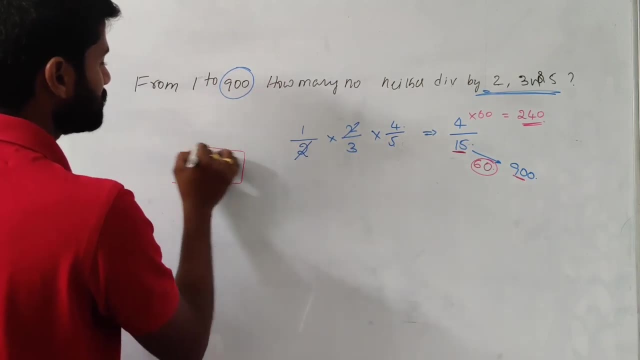 divisible by 2,, 3, 5, those are 240 numbers. For example, if same question, if the question related for 1 to 1000, 1 to 1000, how many digits which are divisible by 2,, 3, 5.. So 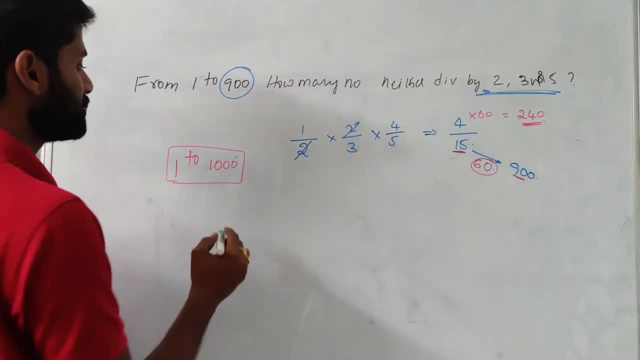 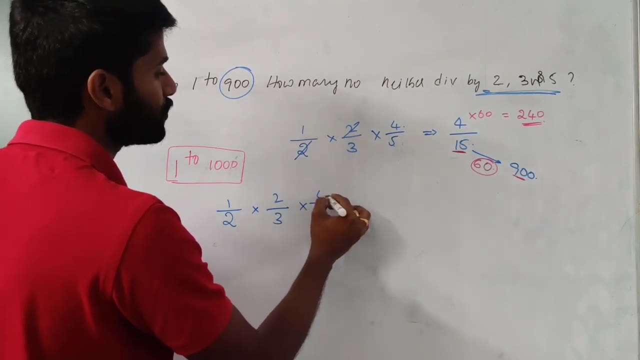 out of 2 numbers, 1 number is not divisible. Out of 3 numbers, 2 numbers are not divisible. Out of 5 numbers, 4 numbers are not divisible. Then the final fraction become 4 by 15.. Just go with the. 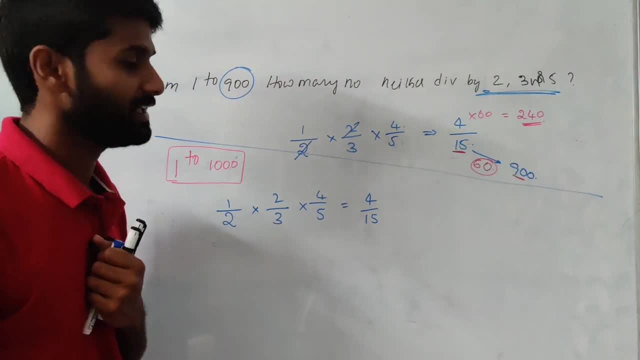 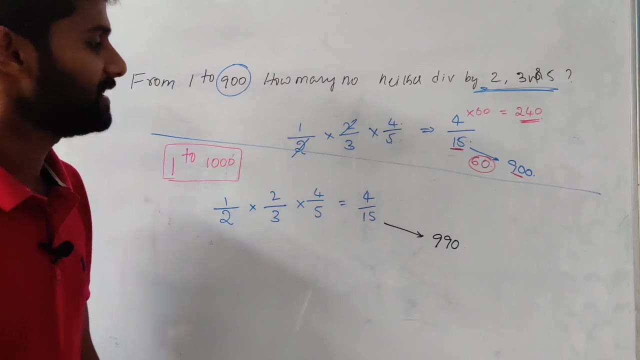 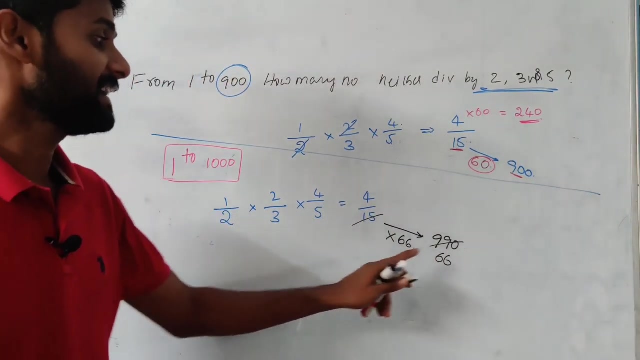 calculation. and 1000 is not divisible by 15.. Consider nearest multiple. the nearest multiple I just consider as 990.. Then concentrated 15 become a 66 times. So 15- 66 are 990.. Consider the exact divisible number. That is why I just consider 990.. 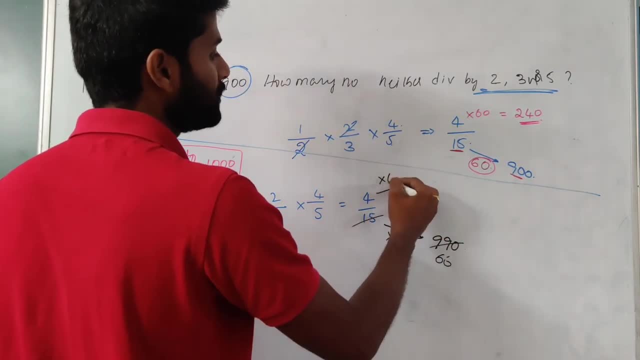 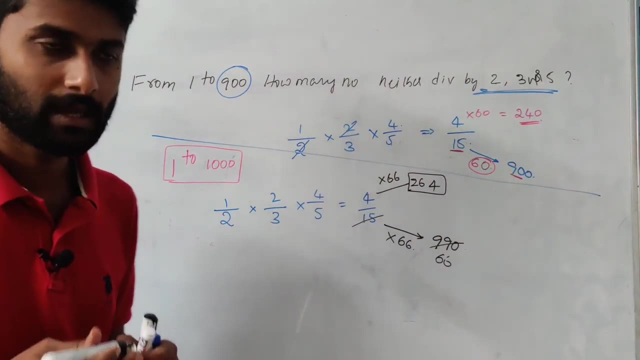 And 15, 66 are 990, and 4 into 66, 4, 66 are 6, 4 is 24, 4, 6 is 24.. Then answer is equal to 264.. But we have a doubt, sir. We consider up to 1000, but you consider 990.. That is why remaining 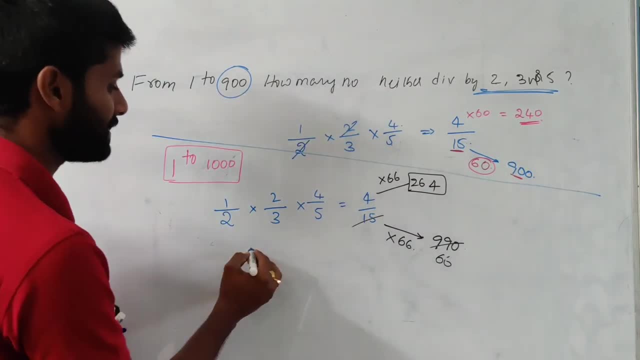 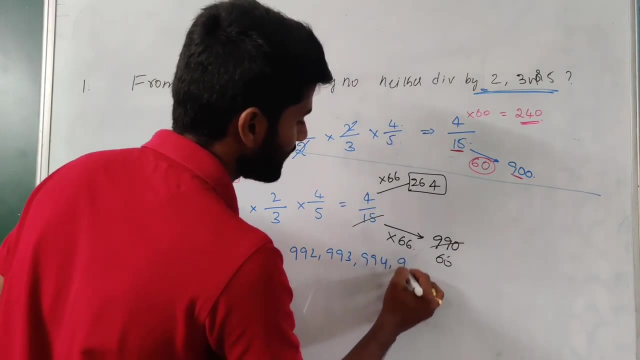 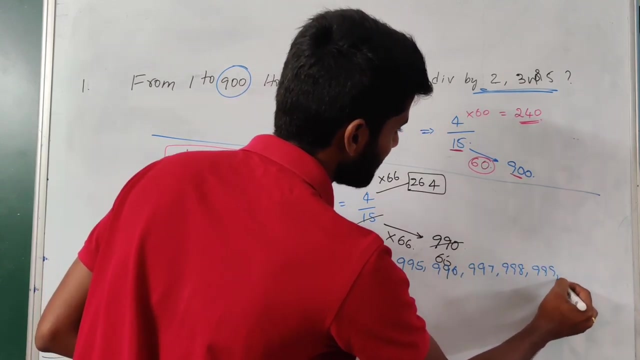 numbers you can. counted in manual way Means what are the remaining numbers? 991, 992, 993, 994, 995, 996, 997, 998, 999 and a 1000.. So just check it out Out of these 3. 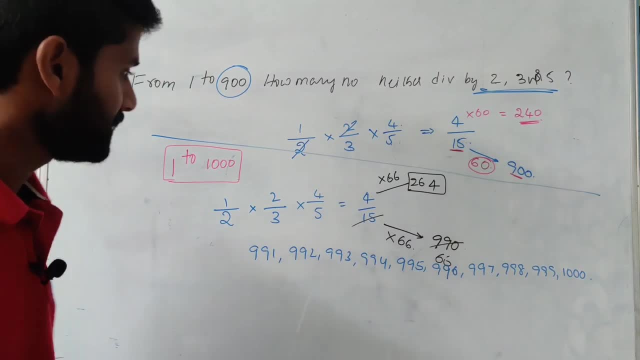 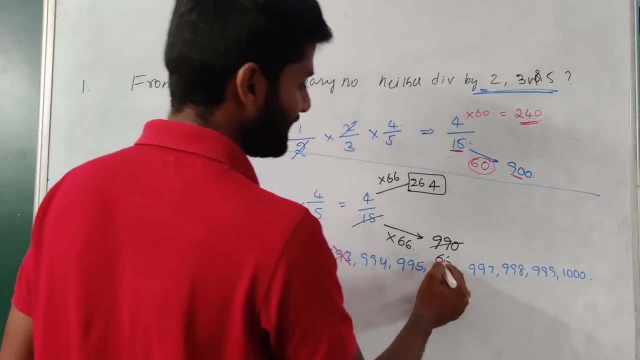 numbers. what are the numbers? which is not divisible by 2, 3, 5.. We know that, according to the 2 rule, 992 is divisible by 2 and 993 is divisible by 3, and the 996 is also divisible by 3.. 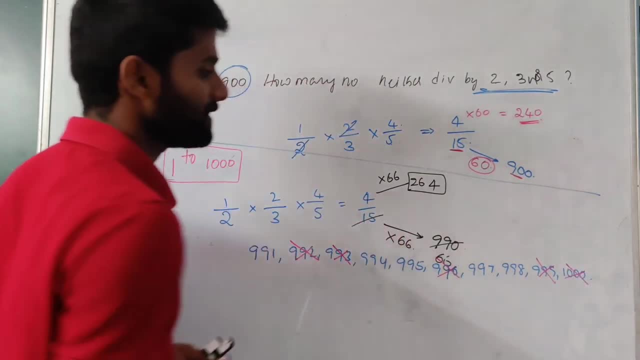 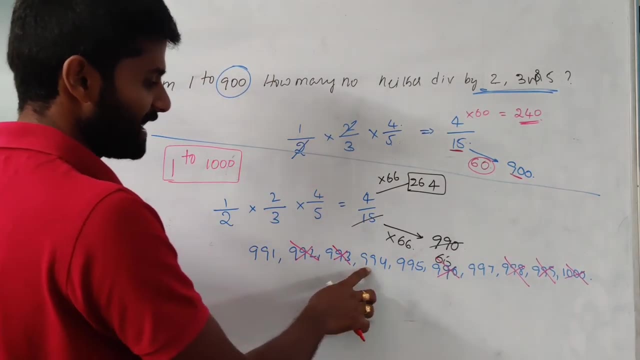 999 is divisible by 3, 1000 is divisible by 5 and undivisible by 2, and 998 is also divisible by 2, and check with remaining number: 991, 994 is divisible by 2, 995, 997.. See, these are all the. 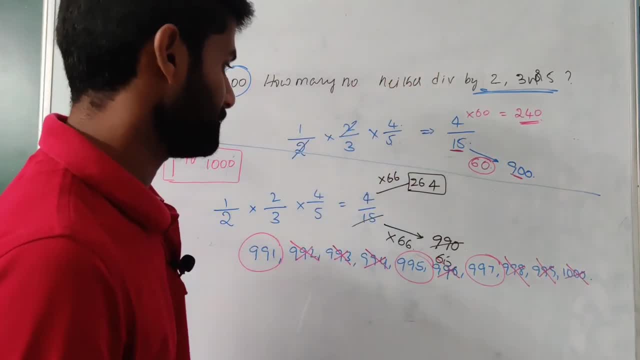 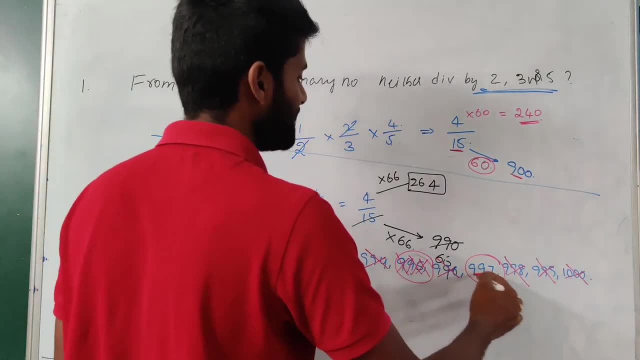 three numbers which is not divisible by those number. Just check with sorry. 995 is also divisible by 5 means 991,. 997 is not at all divisible by 2,, 3, 5. Then the answer belongs to add 2.. So 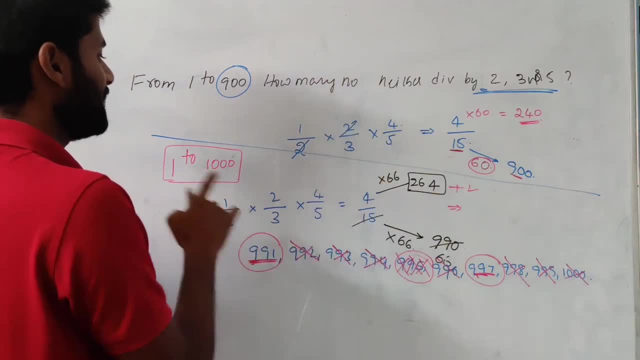 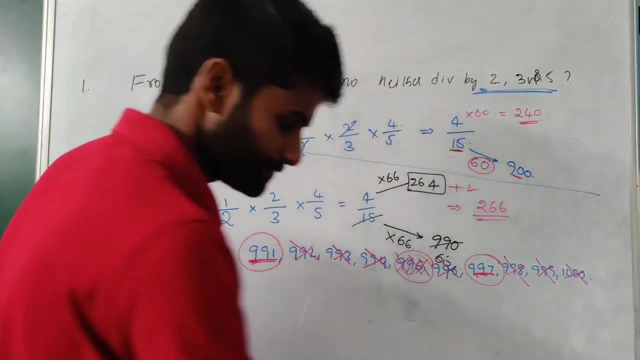 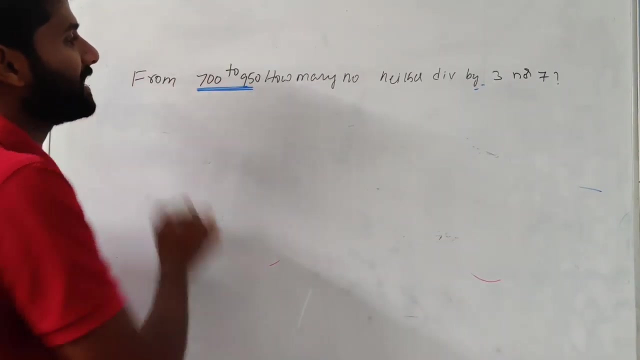 the total numbers, which is not divisible by 2,, 3,, 5 in 1, 2000 are 266 numbers. those are the answer. So one more question, for neither nor The question related from 700 to 950, which is not. 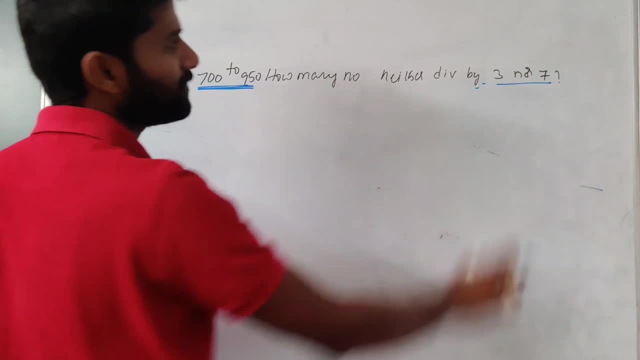 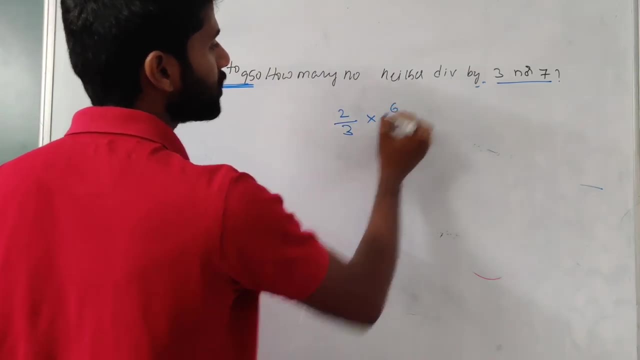 divisible by 3 or 7. First frame: a fraction part for 3, 7.. Out of 3 numbers, 2 numbers are not divisible. Out of 7 numbers, 6 numbers are not divisible. Then the fraction 3 become 2 times. The fraction is exactly equal to. 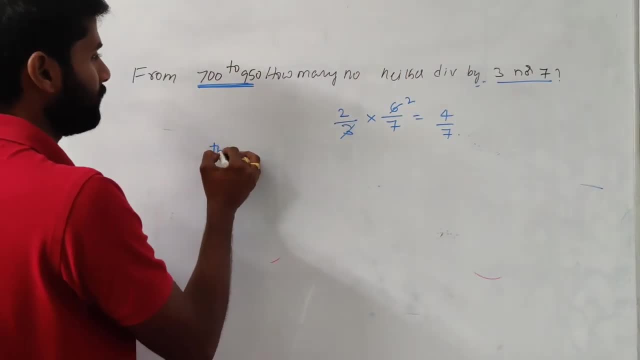 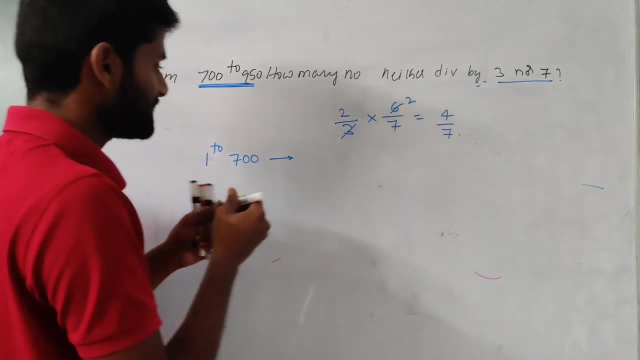 4 by 7.. First I just calculated from 1 to 700.. 1 to 700, how many numbers are not divisible by 3 or 7? We already know that 7 and 700 is exactly cancelled. So 7 become a. 700 is a 100 times. 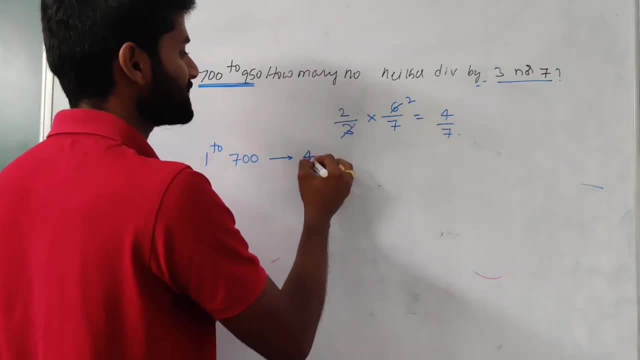 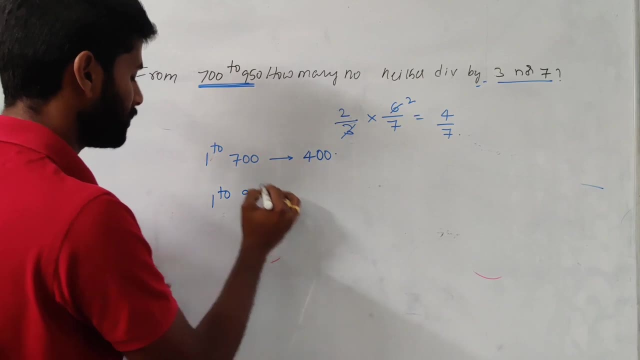 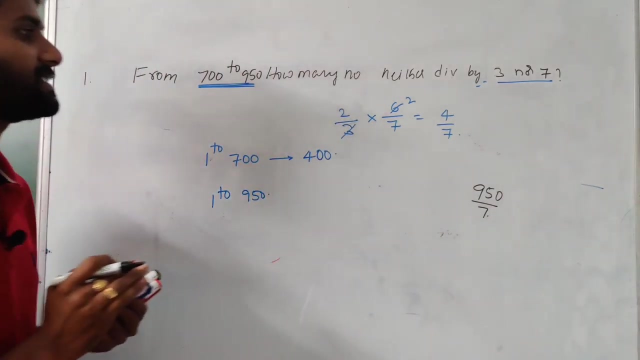 Out of 7, 400.. These numbers are not divisible, Means the answer is equal to 400.. And second one we need to focus on 1 to 950.. 1 to 950. See, 950 is divisible by 7 or not? Just check it out: 950 is divisible by 7. 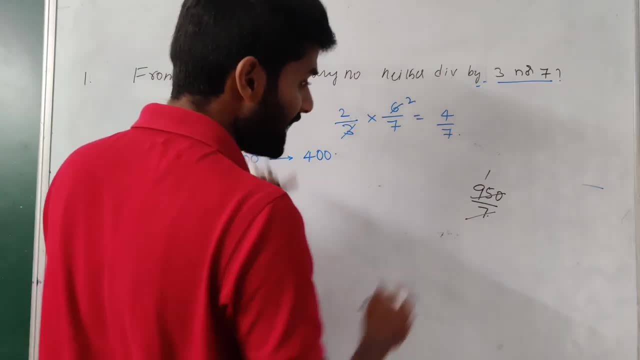 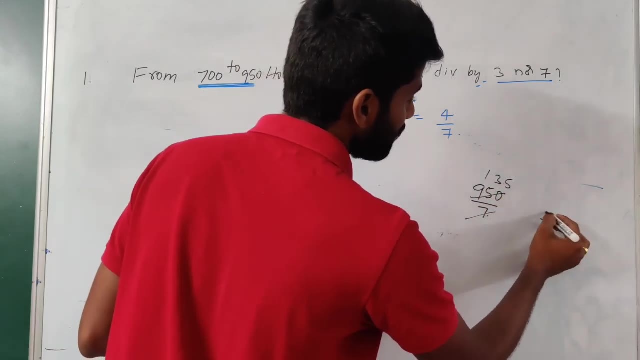 or not. See 7. 1s are 7 and 7. 3s are 21,. 4 and 7 5s are 35. We left with extra forward as a 5. Means. we left with a reminder. 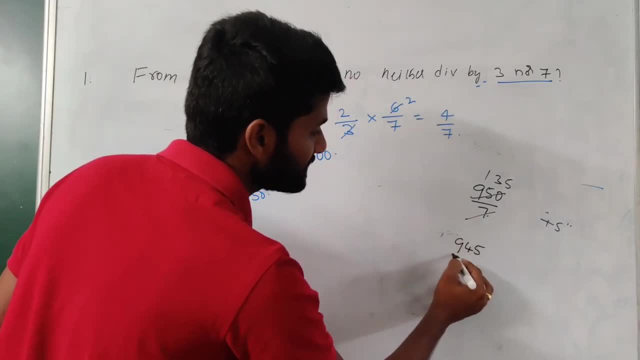 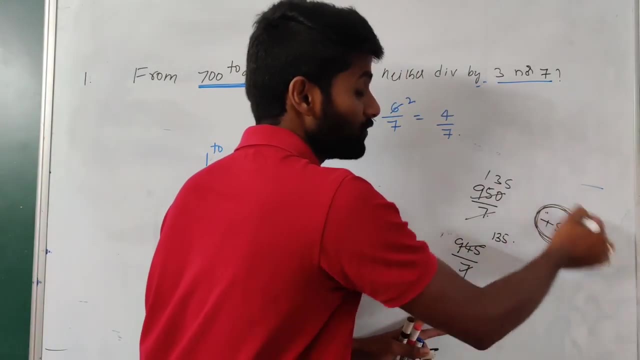 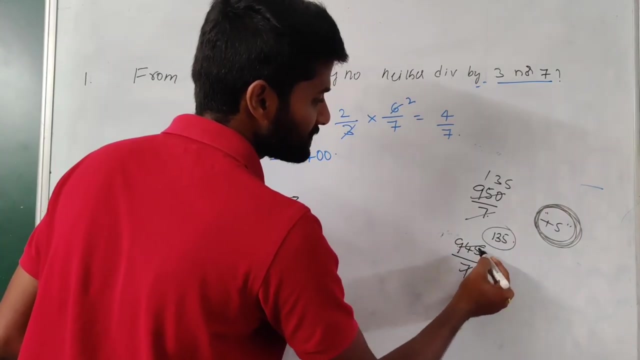 5 means 945 is exactly divisible by 7. in 135 times Means we just: whatever the 5 reminders, So whatever the 5 numbers, we can go with a manual. Then 945 is divisible by 7.. We left with.